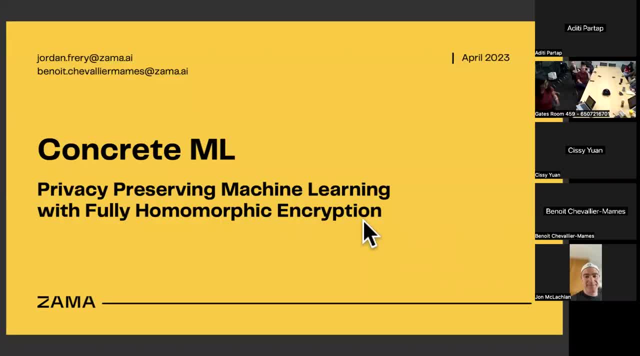 Hello everyone. we are very pleased with Jordan to be here this week in San Francisco. So actually we are finishing a long week of presentations everywhere. So on Monday we were at Google. in the afternoon we watched Pascal, our CTO, present the company. 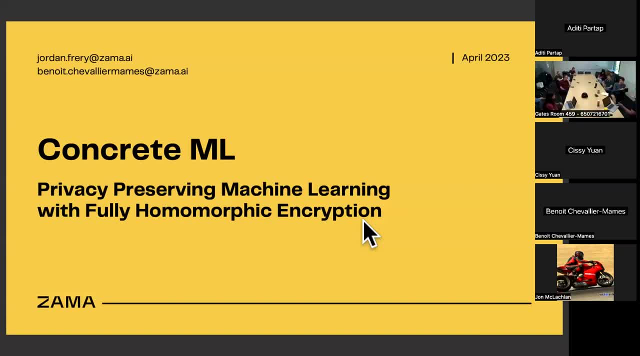 at the RSA Innovation Contest. So unfortunately, as you can see, I'm not with any kind of trophy. So, yes, we were quite good, but we didn't win. Then on Tuesday, we were on stage with Jordan at the AI and ML track, and now we are in. 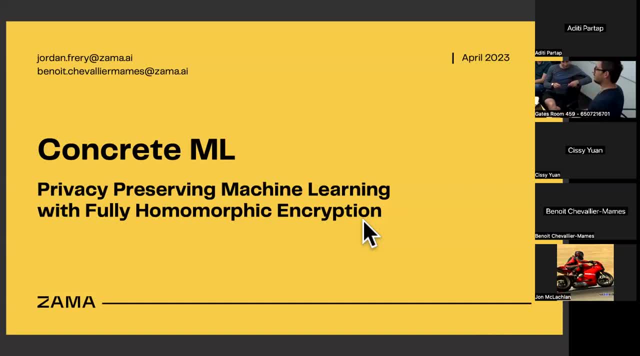 San Francisco Well, with you guys. So we are very happy. a bit tired, Jordan is very tired, but he will find the energy to win, Yes, And you know we are. you know we also have some jet lag from France and so on. 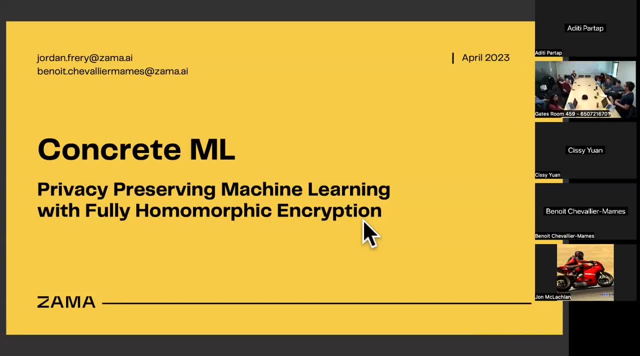 But we are going to present you what we are doing at Zama, which is, I think it's quite exciting, And we are very happy to be there to present this because we know that, I mean, Stanford is the cradle of FHE. 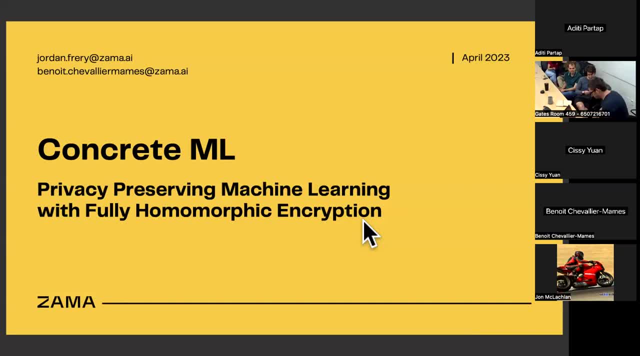 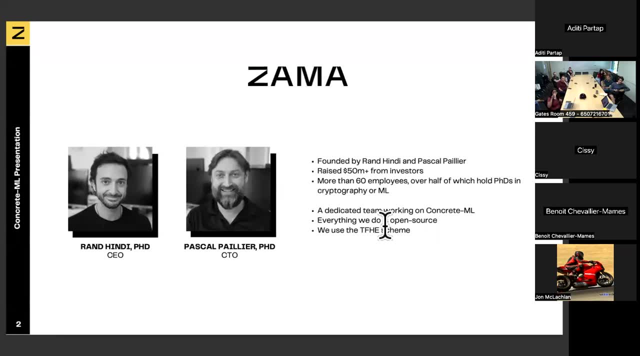 So it's amazing. Yeah, And that's it Okay. So what Zama is? So Zama is the startup in France, mainly in France. We are also in Europe and we are about 70 people. Maybe 60% of us are PhDs. 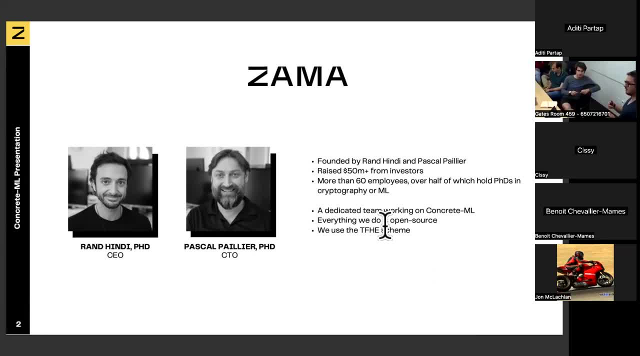 So PhD mainly in crypto, but also some PhDs in machine learning and in compiler, for example, And so our two founders. so Rand, he's an entrepreneur, so he made a few companies and he sold his last one, which was already about privacy. 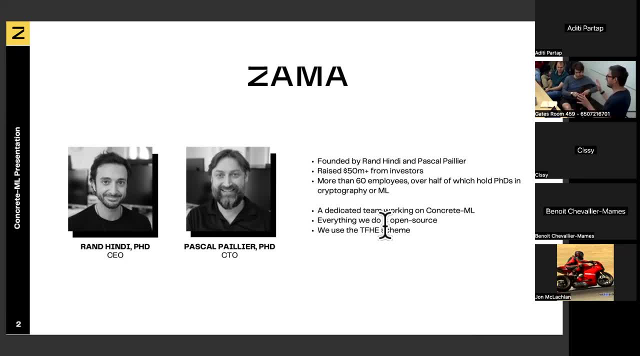 And so we have Pascal. so I don't know who you are exactly, but Pascal is quite well known for homomorphic things for quite a long time. For sure you're homomorphic? Yes, I was in the late 90s, so we've come such a long ways. 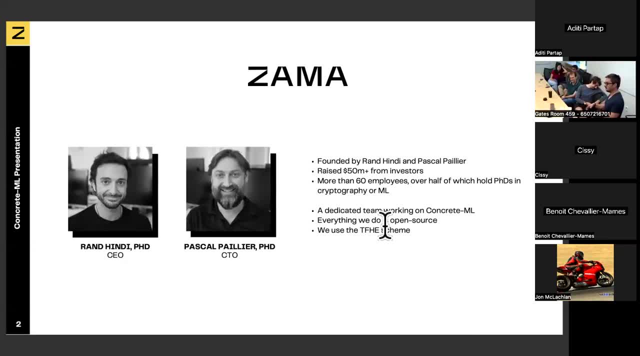 So everything we do at Zama is open source. so if you want to try something, especially for students, researchers, it's free, And so, yeah, we are going to go into the details, but mainly you know what it is. we are using a TSHE. 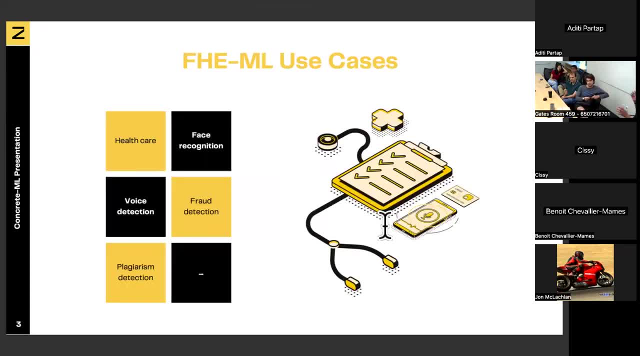 Okay, so machine learning is everywhere, as you know. If you want to classify your emails to detect spam, if you want to have health data analysis, if you want to for your voice recognition, it's everywhere, But obviously no one wants to have this in the clear, no one wants to have this mail or to have health data available to some parties that they don't trust. 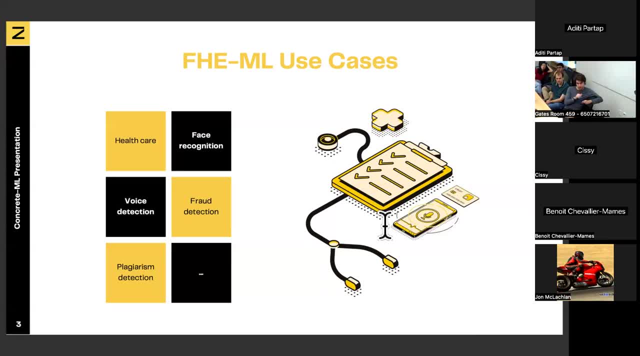 So what we are doing at Zama, especially in the team, is to allow the users to have the same kind of service, but in a way which is privacy-preserving. So privacy-preserving machine learning is what we are doing in the team. 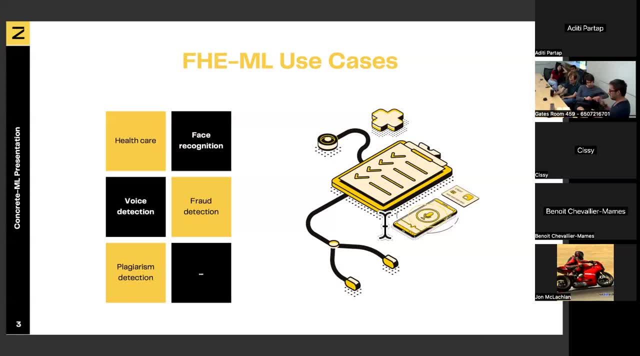 More generally, in Zama it's about what you can do with your IPG. So if ever you have questions, by the way, we'll handle them. And for the good questions, Dan proposed me to give the caps for the good questions. 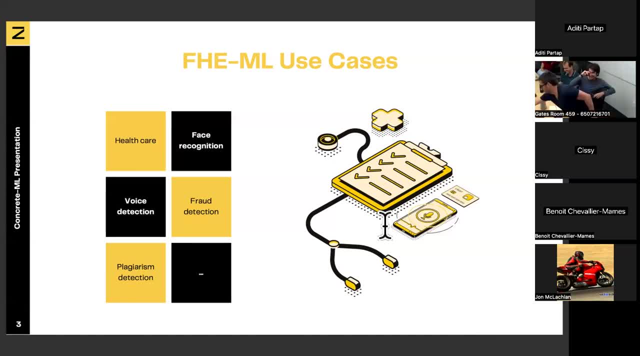 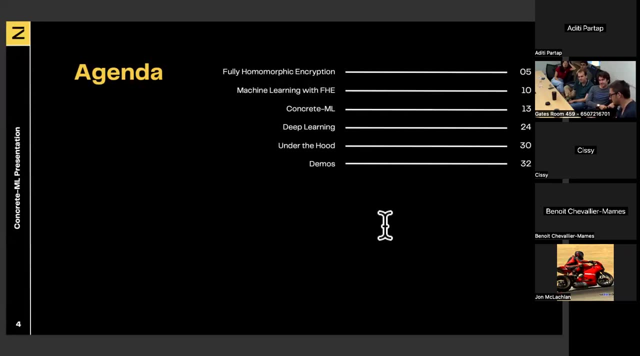 As you can see, they are very nice. a few more questions so you can be very proud of it if you walk in there. So if I were you, I would pick up some questions. Okay, So the agenda. I'm not going to go into the details. you are going to discover all of this. 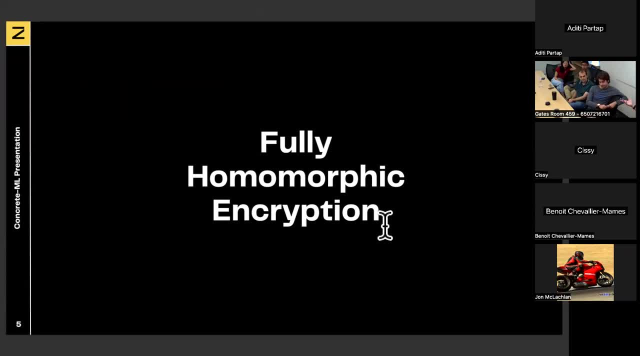 So what FHG is so? sorry if I say something which is obvious to you, and maybe there are some of you in the audience who are not aware of this, so I'm going to take a bit too much, Maybe, for you. So fully homomorphic is the big thing that we are working on at Zama. 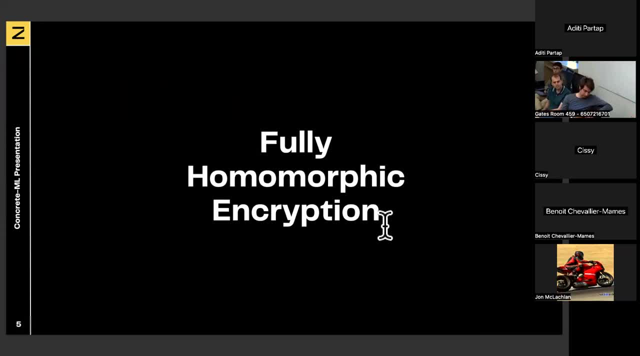 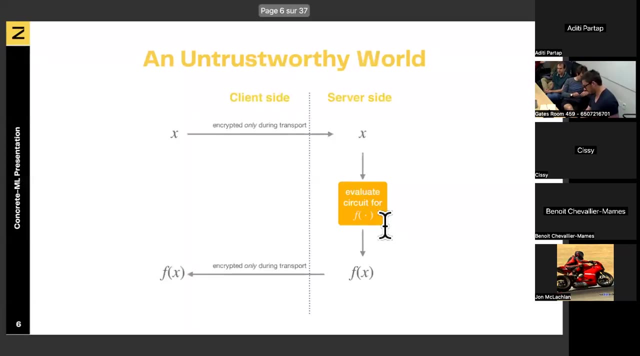 Everything we do at Zama is based on this. So for some products it's for fully homomorphic encryption for machine learning, so our product- or on the other side, there is also FHG for blockchain or these kind of things. 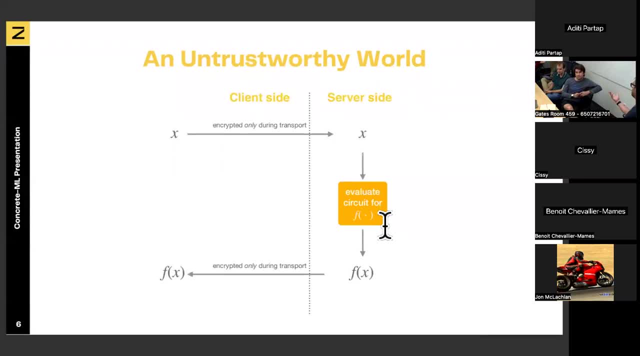 So if you look a bit how machine learning is when you run this in the cloud, something like that, So you have some client in the server, The server is going to run the machine learning algorithm and the client has the data. So the data is x. so maybe it's data that you don't want to share. 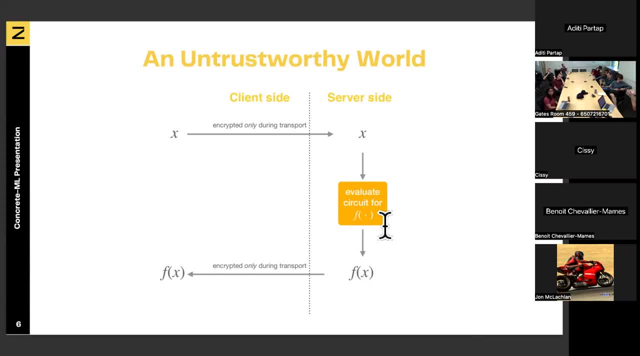 What you do is you encrypt it during the transport. you send it to the server, which is going to decrypt it because it has the same keys as you. Then the computation of the f function is done in the clear and just for the transport. so when you send it back to the client it's also encrypted. 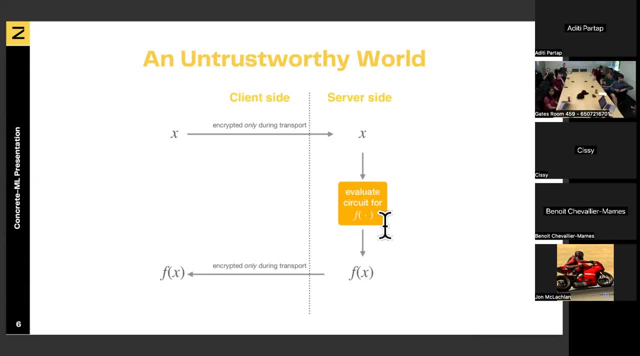 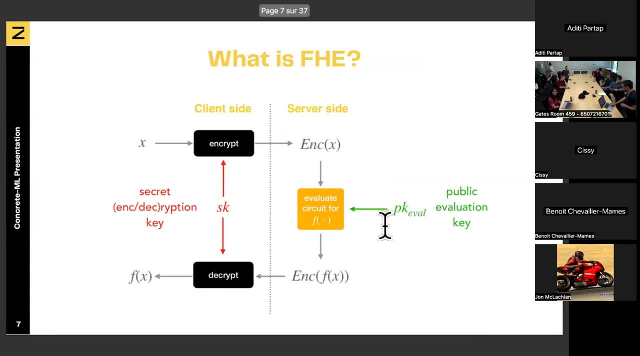 But, as you can see here, the server knows everything, It knows your data and it knows the result of the computation. So that's not something that we want to have. it's not a good property. So what we are doing at XANA is to try to have something which looks like this: 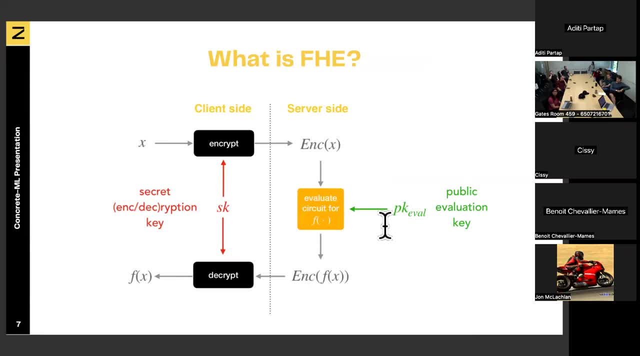 So here you also have the data. you are encrypting it with a key, but the big difference is that this key is not known to the server. So the server will never be able to decrypt anything. it will just have the encryption of X. 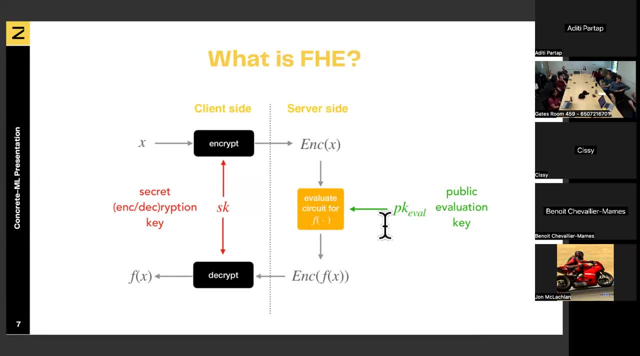 But thanks to some mathematical properties that we are going to discuss, we are able to turn the function f, the machine learning model, or actually any function, into an FHC equivalent, which will be able to take encrypted inputs, which will have some information to run the computation. so public information. 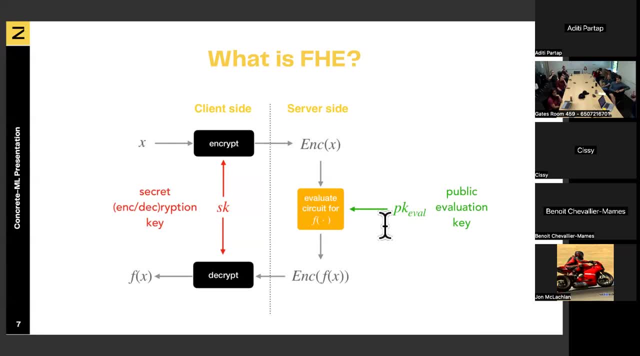 And at the end the result will be f of X, but encrypted, And never Any intermediate value of the inputs or the outputs will be decrypted because actually the server doesn't know the key. And then you send this result back And that's the only moment with the key, which is only on the client side, where you can decrypt things. 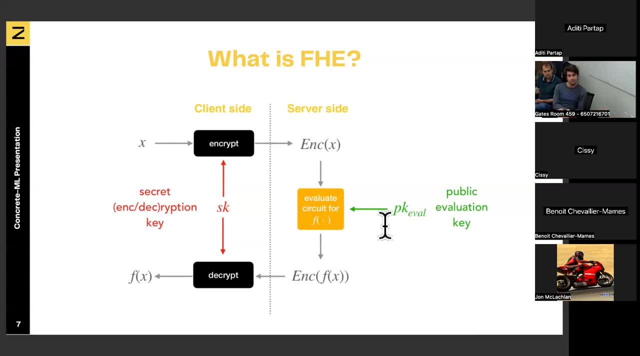 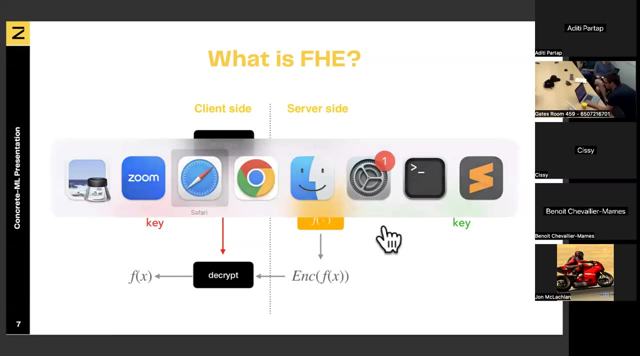 So at the end you have f of X, which is what you want it to be, the compute. But never things have been Okay. So for people who don't know FHC, it looks a bit too magical. So let me show you this in practice. 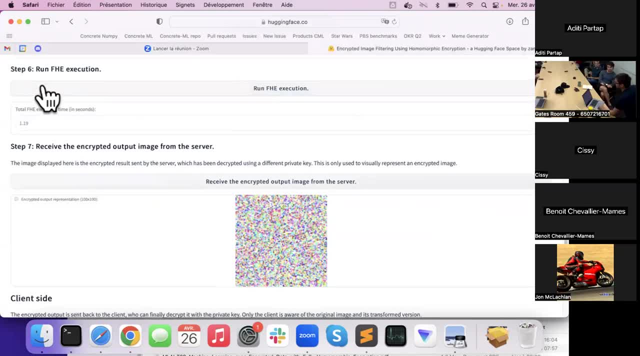 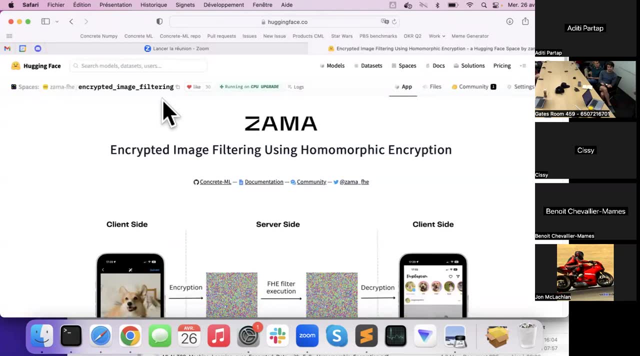 So Hugging Face. So Hugging Face, if you don't know, Hugging Face is a kind of github for machine learning, So it's a bit where people want to show things when they want to make a demo of machine learning stuff. 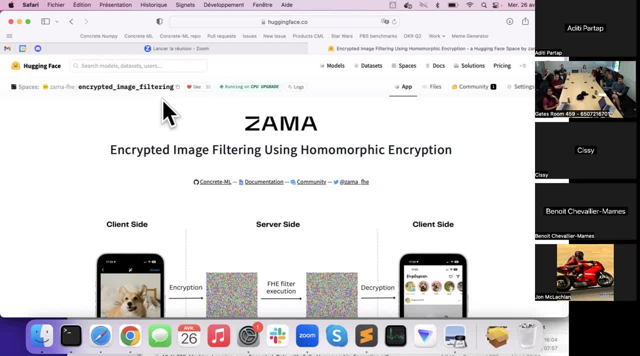 So we have. We have created our own space on Hugging Face And we are publishing some demos of what you can do with Hugging Face. So this one is an encrypted image filtering. There is another one. If you want to run this, it's also possible. 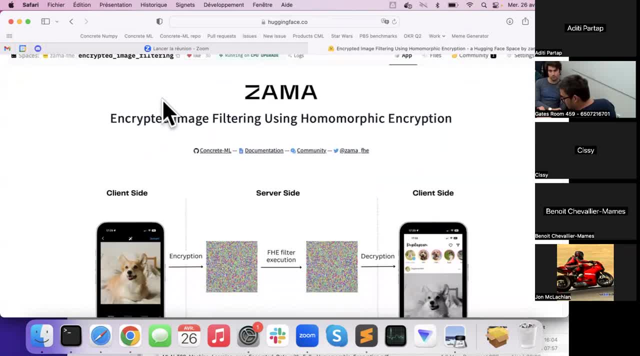 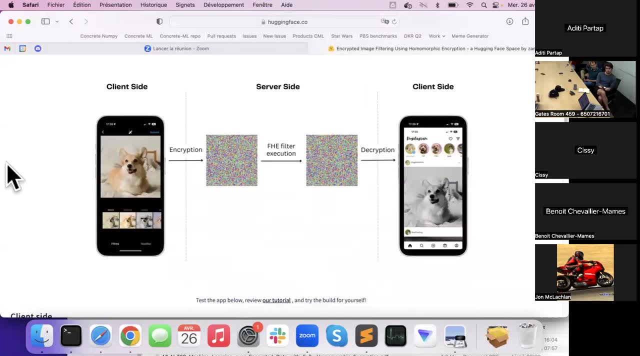 I mean it's publicly accessible, And let me show you what this demo is about. So it's more or less what we have shown in the previous slide. So you have the client, which has some private images that he doesn't want to share. 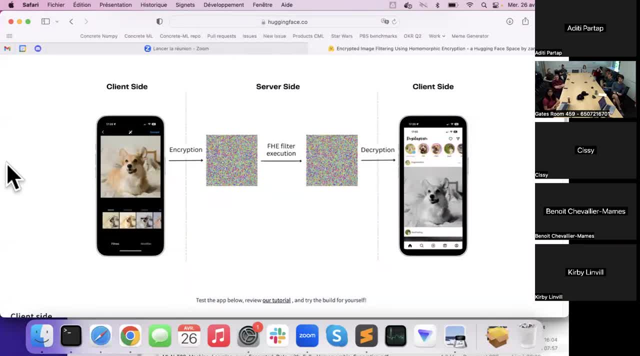 So what it does is that it encrypts this image, Then the image. It's an encryption, So the image is going to be random looking, But still, thanks to the mathematical property, it's possible to apply the filter on the encrypted image. 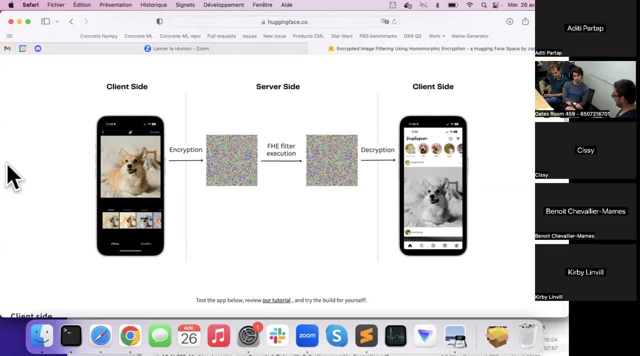 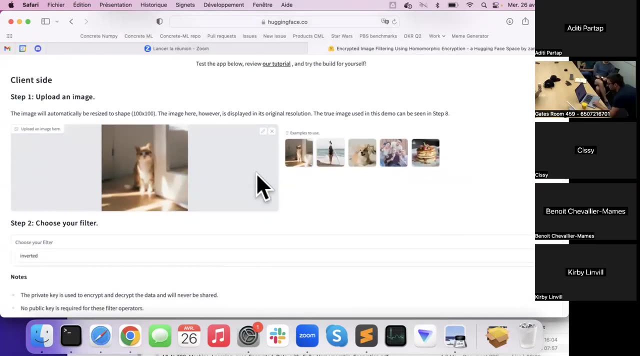 So then you will have the other random looking image on the right, And so this has been computed on the server, And then you send it back to the client who can, with his private key, decode all of this. So, if you look, 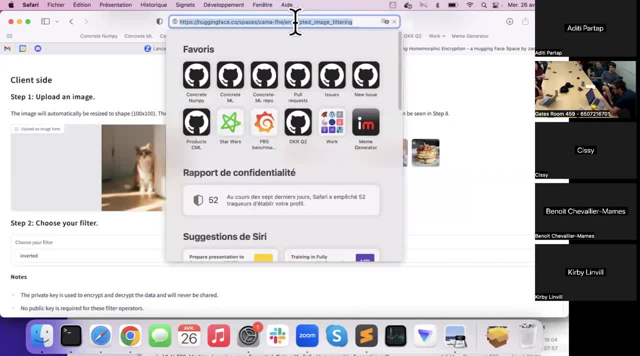 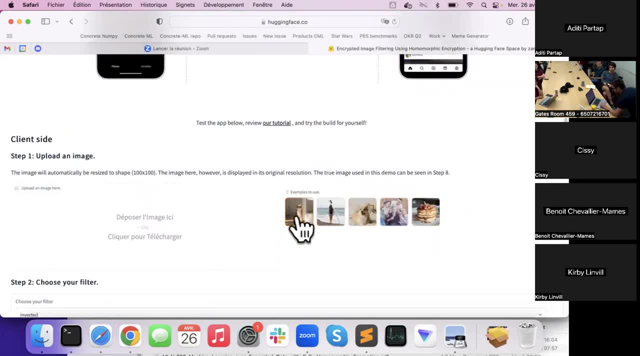 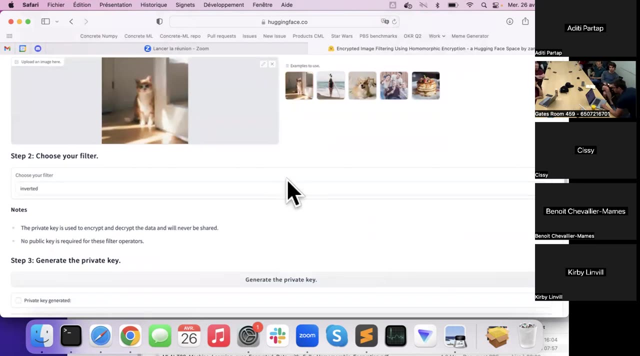 So sorry, I did it this morning, So let me refresh. Okay, so when you want the demo, you have to choose one of the images. So let's take the cat, But you could drag your own image if you want. And then there are some features. 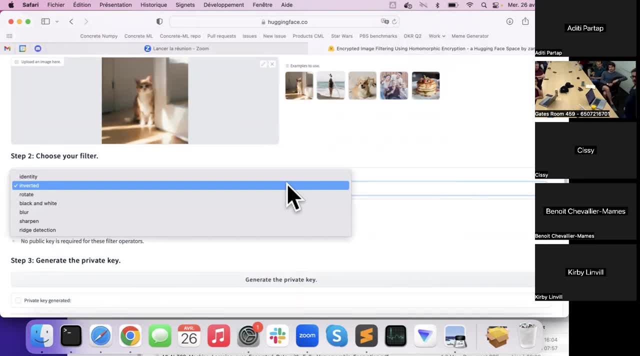 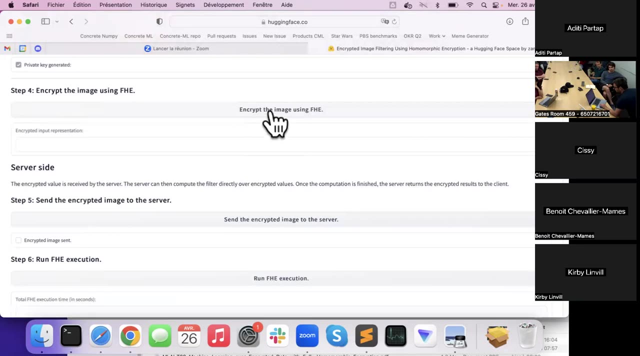 So in the example above it was black and white, So you have a bunch of filters that you can apply, So let's take inverted. Then you generate the key, which is going to stay on the client side, Except for the public key material that you sent to the server. 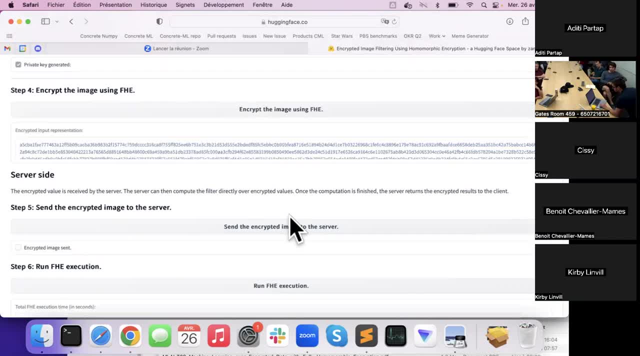 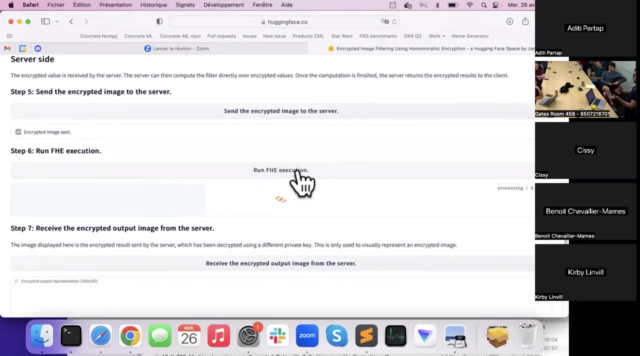 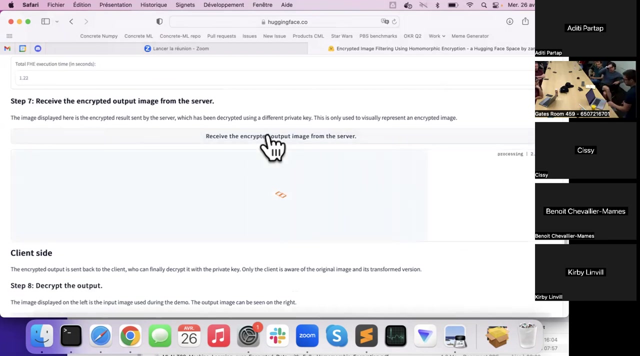 Then you encrypt the image, You send it to the server, Then you run the FHT example, Then you run the execution. So basically, filtering is just a convolution, So it's something which is very complicated to compute, And then you send it back to the client. 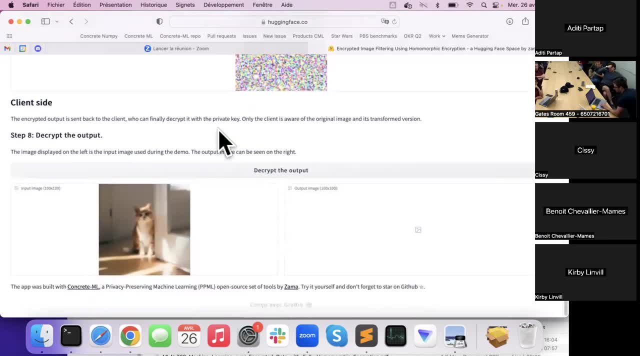 So you have the output, which is a random key And you can decrypt And you can recognize the cat, But the colors have been inverted. Yes, You have the identity in there. Does that mean the server side will know that it's produced the same output as it got its input? 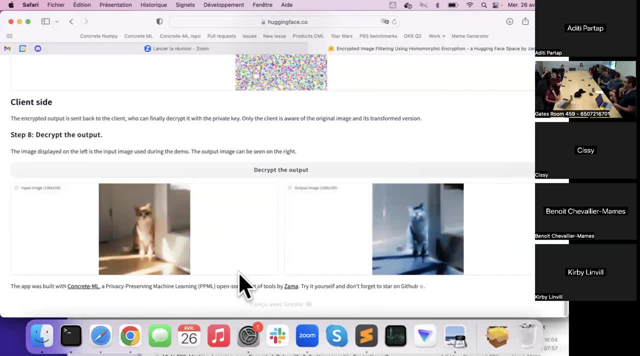 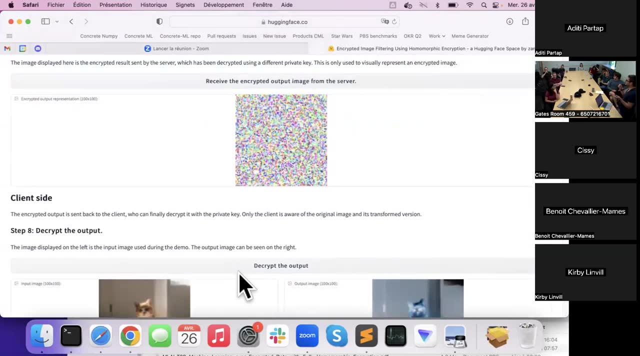 I have not understood this question. So, because it's identity, right? Oh, you mean the identity filter? I don't know what the identity filter is. So the server knows what the function is. So, yes, the function that we are computing is not protected. 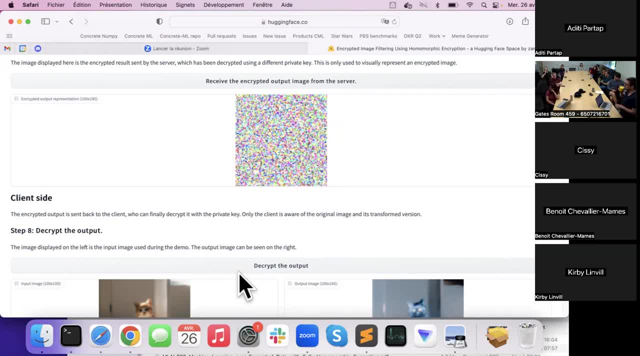 Yeah. So what I'm wondering is: could there be a function that just by chance produced the same output for a particular input, And would that leak information? It would not leak information because the result is still encrypted, But it's identical to the input. if it happened. 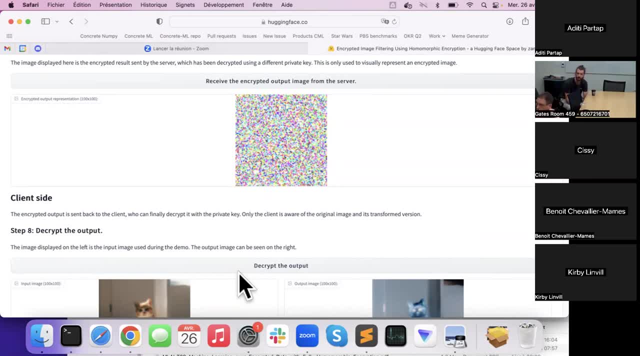 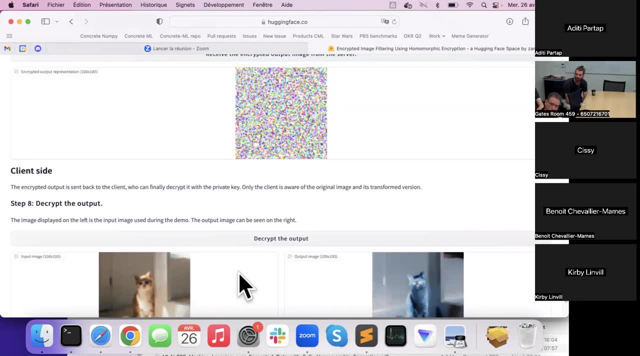 It's not going to be from the site. That was my question. Yeah, that was my question. You know the encryption is Meaning that you can like encrypt this thing twice. It wouldn't be able to. Just thinking of a general algorithm that I by chance put into parameters that produced an identity transformation. 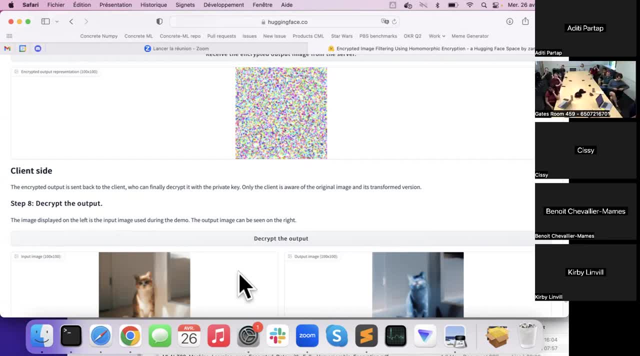 And then the server question was: would the server know that that had happened? And that's a leak of one bit, maybe, But I mean what is computed by the server can be computed by anyone, because there is nothing private. Yeah, So it would mean this would be an attack against the original site. 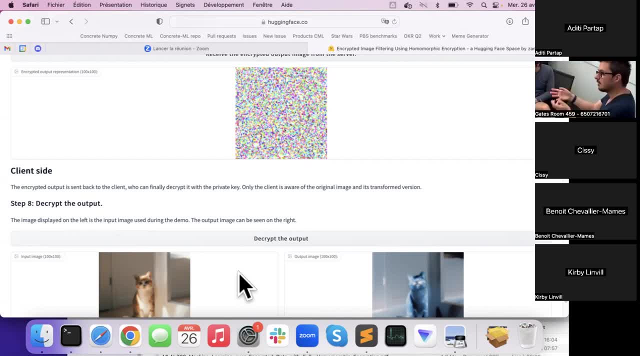 It's the original ciphertext which is proven secure by. You could consider trying to protect the confidentiality of the function, But this isn't something that we support technologically yet. But a lot of people are also wondering: Yeah, that wasn't the question. 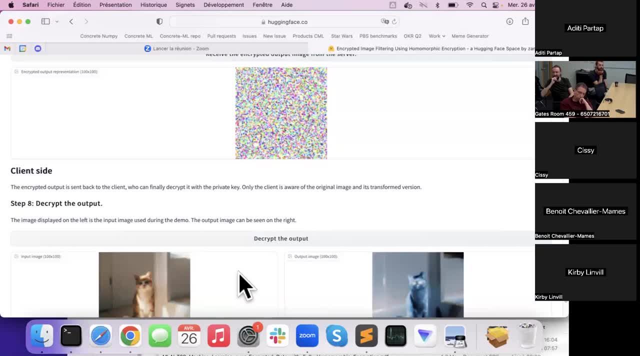 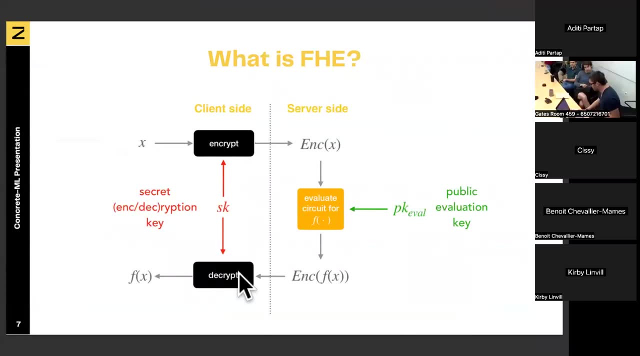 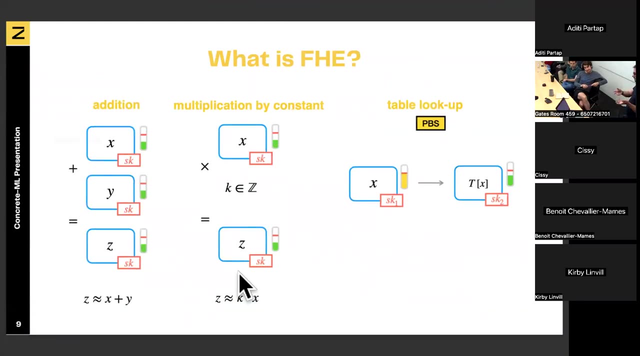 And FHE can do that. by the way, It can do something. OK, that wasn't the question. OK, OK, So you have seen it in practice. Now how does it work? So, actually, FHE is this magical weapon that I'm going to explain. 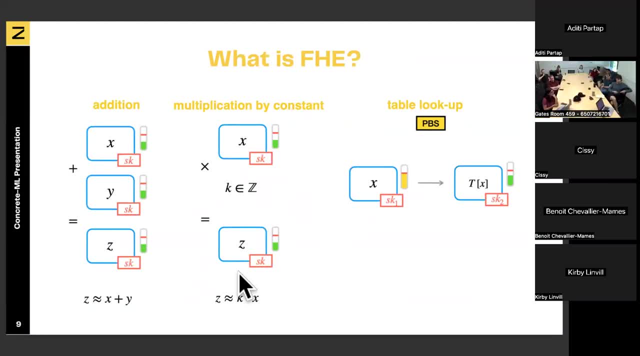 So the important word here is homomorphic. So here it means that there is some kind of malleability for the ciphertext. So notably when you have an encryption of X, an encryption of Y, it's possible thanks to, only with public key information. 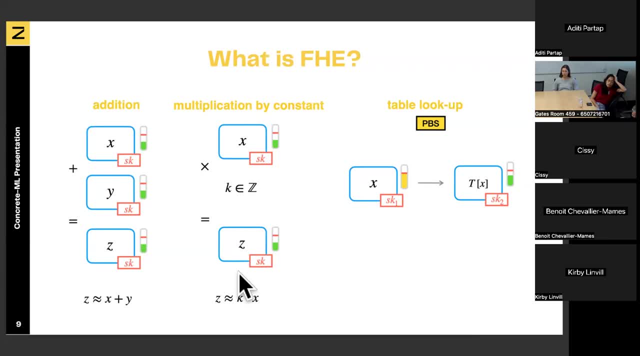 with an encryption of X plus Y. Same thing: It's possible to multiply a ciphertext by a constant, which is in the clear. And then there is a third operator, which is unique to TFHE, which is a scheme that we are using at Zama, which is the programmable bootstrap. 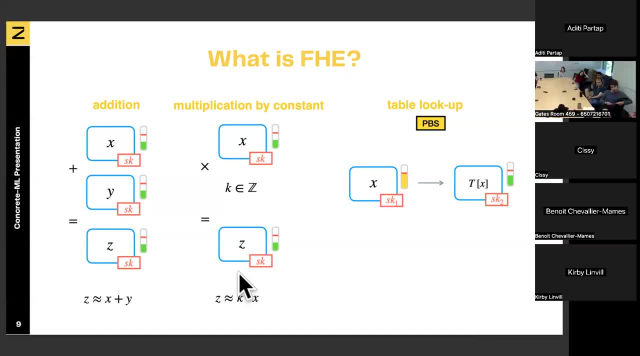 And so programmable. bootstrap is the equivalent of table lookup, but in FHE, Which means that at compilation time you have chosen the function of your choice- T, which is a constant- And you can apply this table lookup on an encrypted value and directly get some T of X. 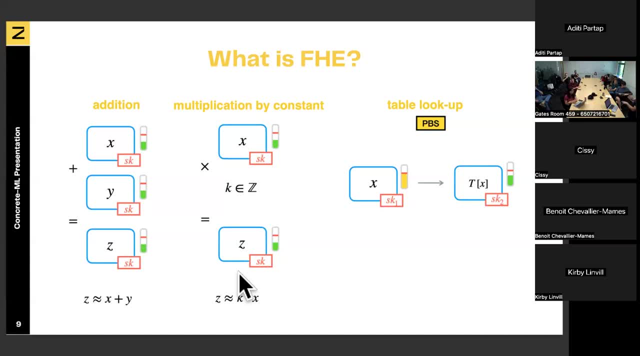 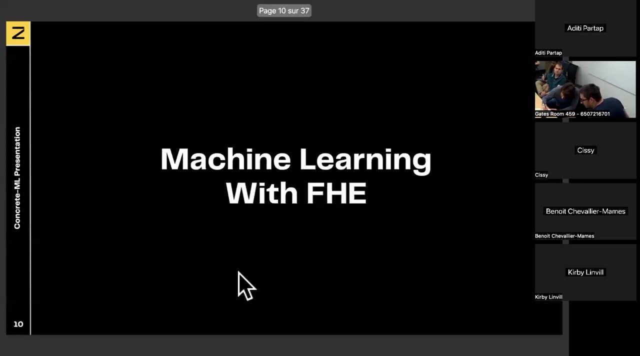 So we are going to see. this is the magical weapon which is used in ConcreteMN And, let's say, in all the tools that we are doing at Zama. it allows us to replace anything which is not naturally FHE friendly. OK, so now that we've seen the few operators which are available in FHE, 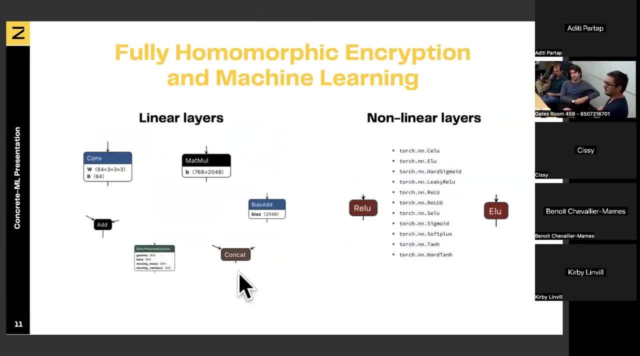 let's have a look to what it gives us for machine learning. So if we have to divide the operations in machine learning, we can more or less have two categories. The first one is for the operators, which are more or less additions of additive nature. 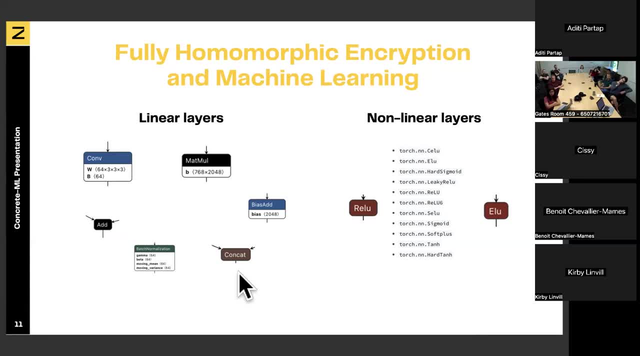 So here you have the convolution, the matrix multiplication and so on. So here, more or less, it just directly applies the same operation on ciphertext and it will work thanks to the homomorphic properties For non-linear layers, like activation. it's another thing. 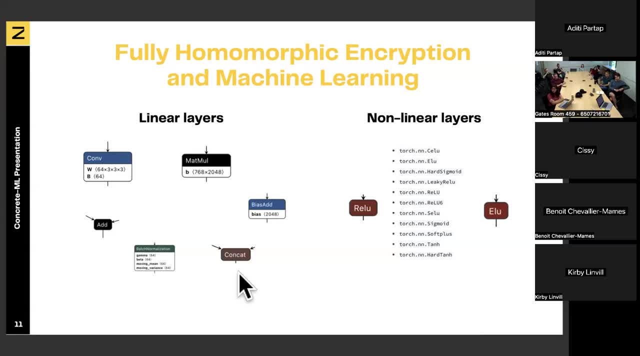 So what we are doing at Zama is that we are replacing these operations by the table. lookup the PVS programable bootstrapping in FHE. So you just have to, let's say, when you compile the program you have to compute or to measure the range of the inputs. 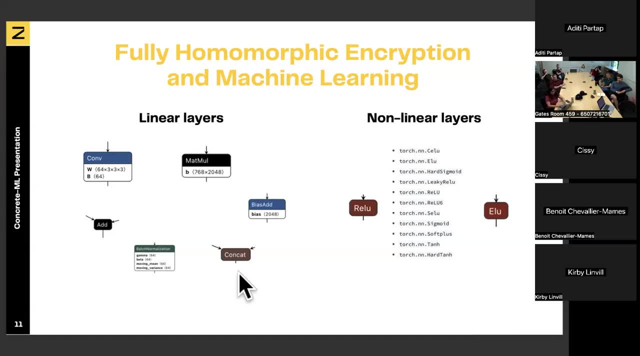 so that you know the range of the input of these activation functions. so you can pre-compute the table lookup corresponding to this range of inputs and you just replace the activation function by this table lookup. You tell me if you want to, if you have questions. 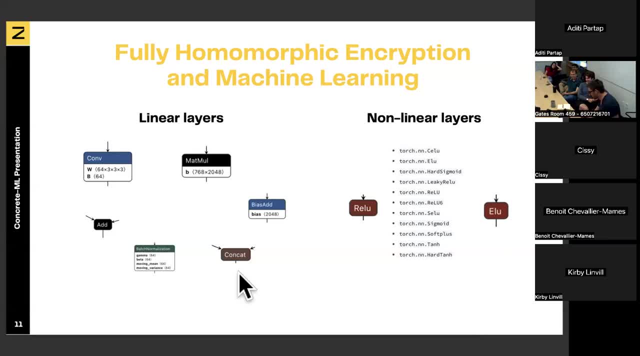 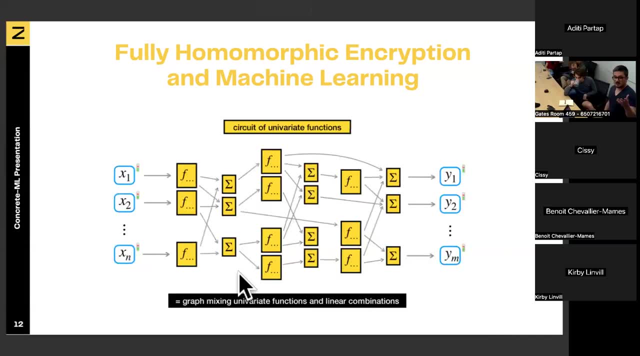 that's our studio, the CAHPS team, so I'm interested in the performance. Yes, we are going to go to this afternoon. Yes, So at the end, we have taken our machine learning model and we have replaced it by something which looks like this: 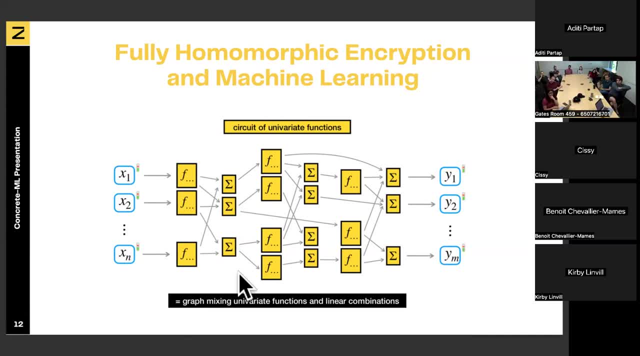 So you have the linear operations, which are the stigma, which are the same linear operations and other data, And then you also have the activation functions, like the overview or so, that you have replaced by the PVS. So it's possible more or less to replace not all. 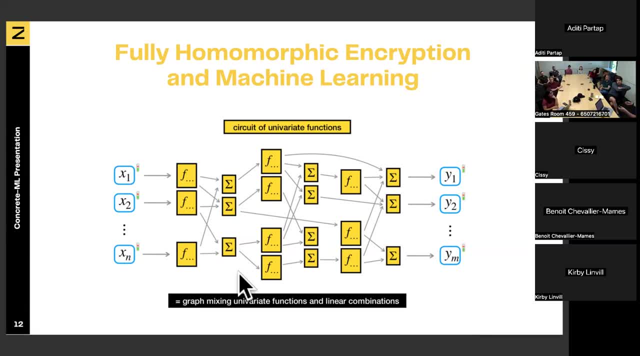 but really most of the machine learning models, And it's just a matter of, yes, of performances. So PVS is great, but it's not free. So if you can, you try to have less PVS or maybe a PVS of a smaller size. 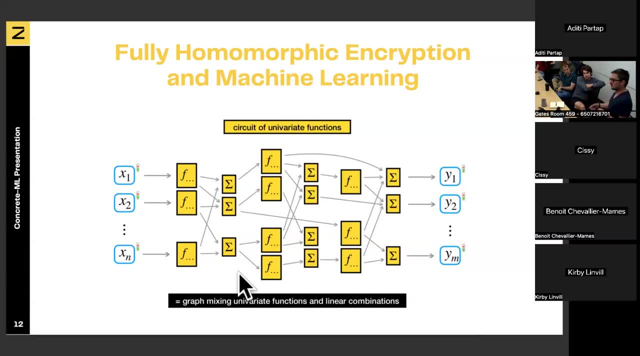 So you are going to see this when Jordan speaks about trees, for example? Yes, Go ahead. I noticed on the previous slide. for the programmable bootstrapping, the secret keychain is from SP1 to SP2.. Yes, So for every PVS or for every table, lookup. 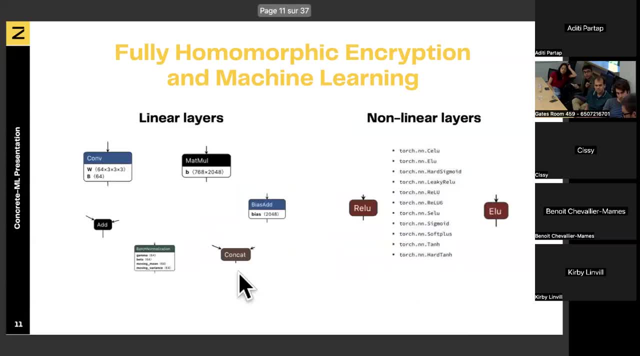 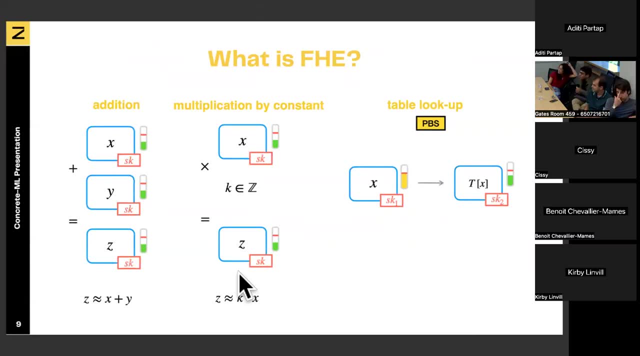 will the client have to generate that many keypairs? How does that work? It's a reentrant, So it's reentrant Whenever you, When you do a PVS, So actually the PVS is composed of several ingredients, So you go through like a key switching operation. 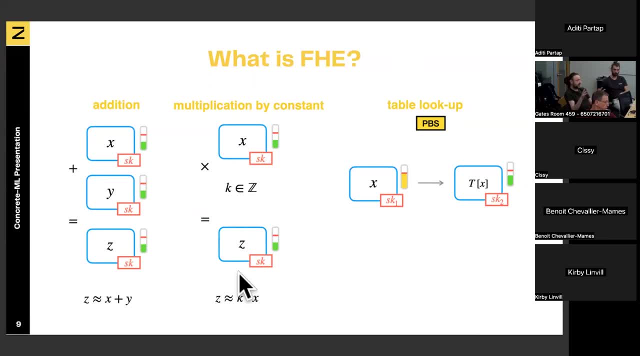 and then you go through a rotation which is a bit like specific to GFHG and other schemes like FUE and schemes that use like line rotation, well, multiplication of a polynomial by a simple polynomial. So when you do the key switch operation, 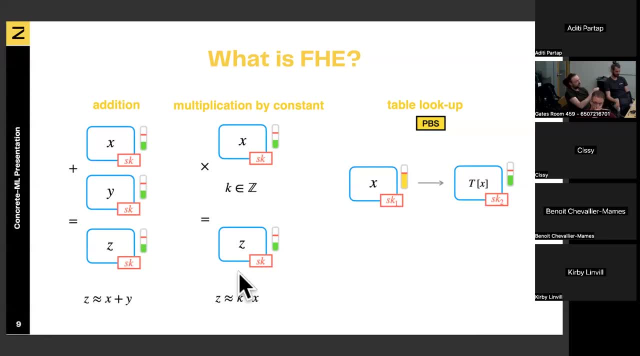 you're actually switching from SK1 to SK2, and then, with the line rotation, you're actually moving from SK2 to SK3, but you make it reentrant, meaning that SK3 is actually SK1. So you call PVS the whole thing. 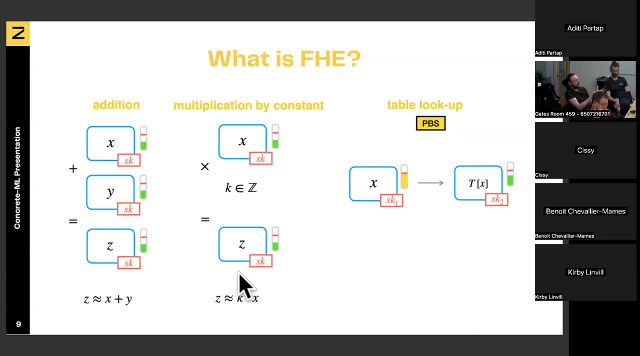 and then you're encrypted with the set parameters both of the input and output. So you use the same Yeah key to add the concept Yes. So you can do everything with like one unique key switching key, one unique line rotation key. 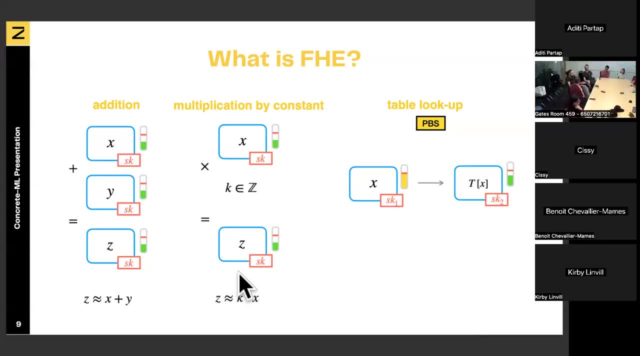 But you could also. You're not forced to do that. I mean, this is what we're doing right now because it suits. you know, machine learning models. It's very easy, you know, just in your layers, and then you've got the execution layers. 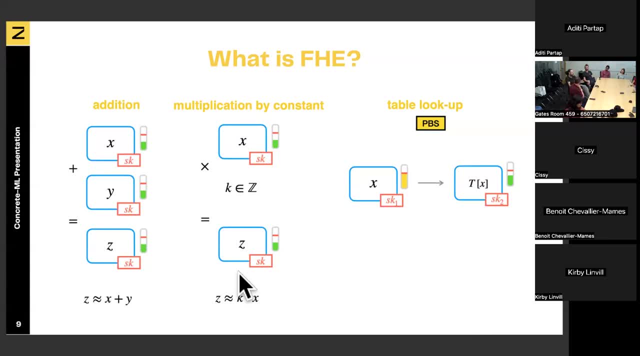 And so it makes sense to do things like that for machine learning, but for other applications, if you want to like handcraft specific circuits, you could play around and not force the PVS to be reentrant. You could have like. 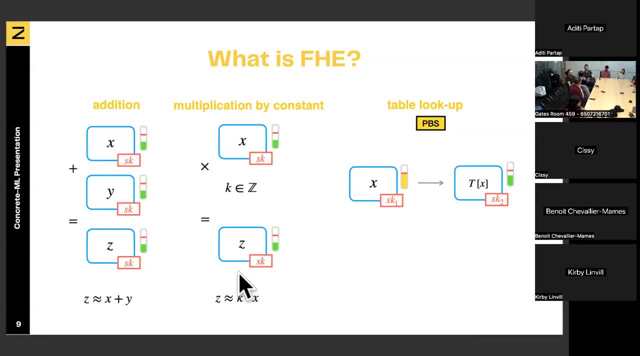 a chain of keys and it's up to you to find, like, the optimal parameterization so that you can save the problems. So does this mean circular security? Yeah, At some point we need these kind of solutions, And so this depends on. 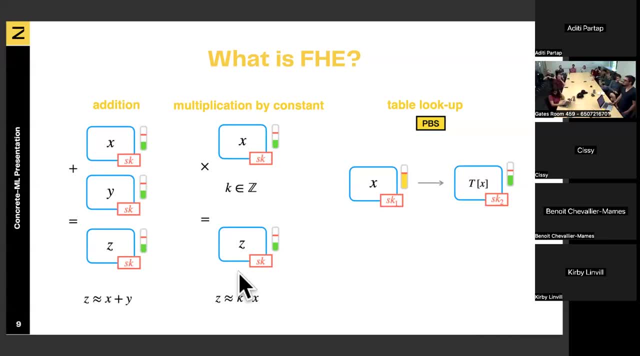 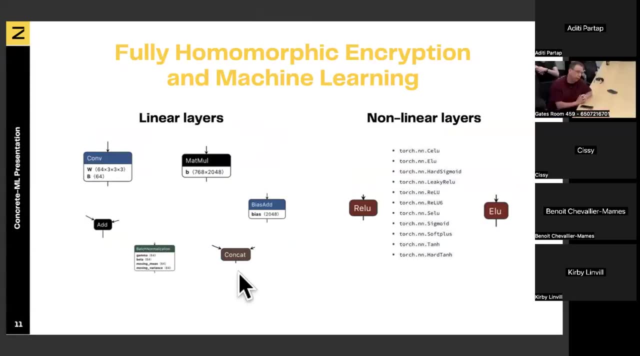 the limited precision needed for machine learning. Yes, So yes, we're going to think about it in more context, But actually before you There's one important point that I think you should say, just to make sure it's clear to everybody. 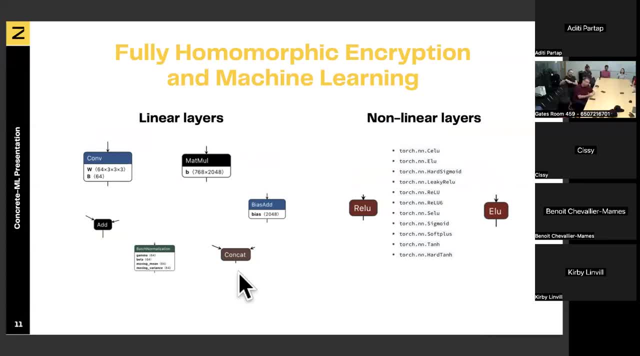 Like in the demo that you gave about inverting an image. Yes, I could have just inverted on my phone, I didn't have to send it to the server. Oh, yes, And here the server could just send the model to the phone. 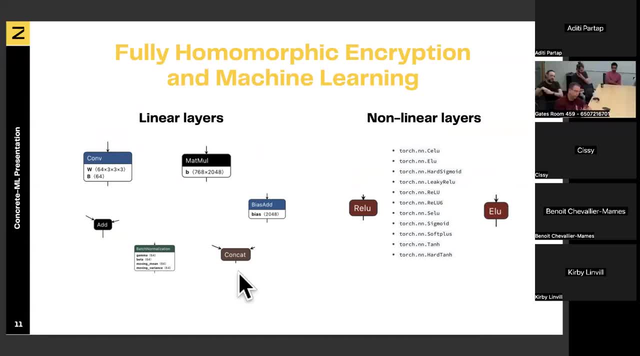 Yes, And the phone could just evaluate the model itself. There's no need for FHC. Yes, So where? Maybe you could just say where does FHC come up? So, for example, if ever you want to protect the IP of your model. 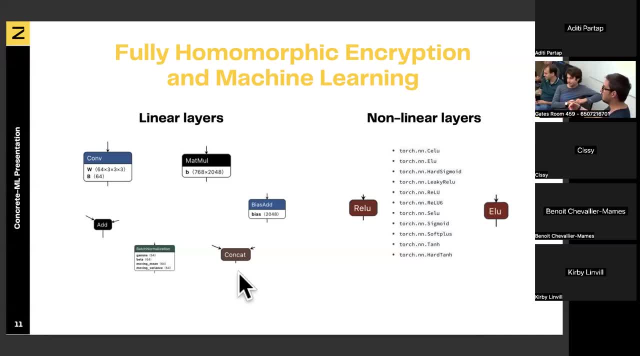 and you don't want to share it on the device because, I don't know, maybe you are Microsoft and the device is an iPhone. You don't want to share it, So you can run it on your own server and by keeping the privacy of the user. 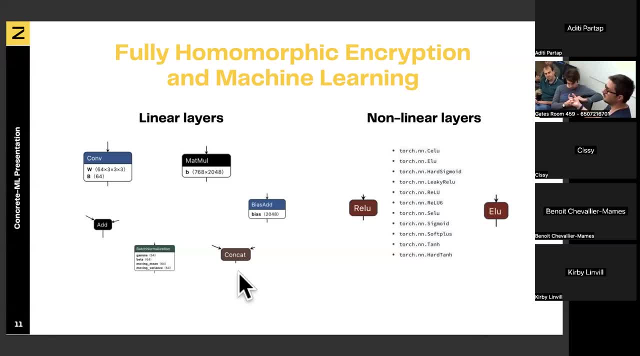 So both of them are happy. They just have to wait a bit longer, But I'm not going to let you have to hook that. Yeah, As a malicious user, I can send you a bunch of data and see how your model works on that data. 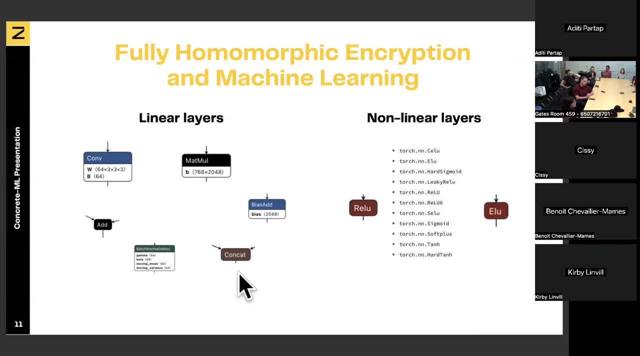 Yeah, sure, And then I will just extract your model from the server. Yes, Yes, directly. So actually all the machine learning attacks that you have in the client, I mean, FHC is not protecting against it. So what you have in the client exists in FHC. 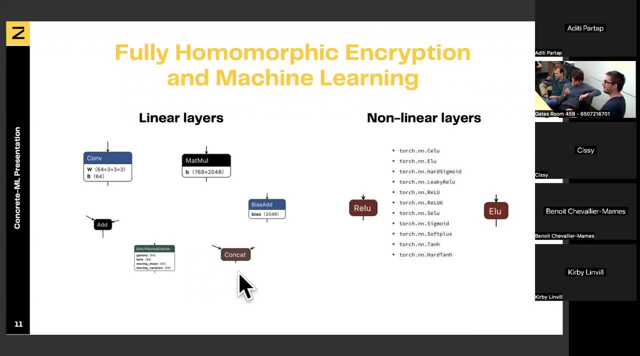 The other use case, though, is if you and I both need to provide some input. we don't want to reveal it, Yes, Yeah, but under repeated allocation. So, yeah, FHC is not going to protect against that analysis. And also what? 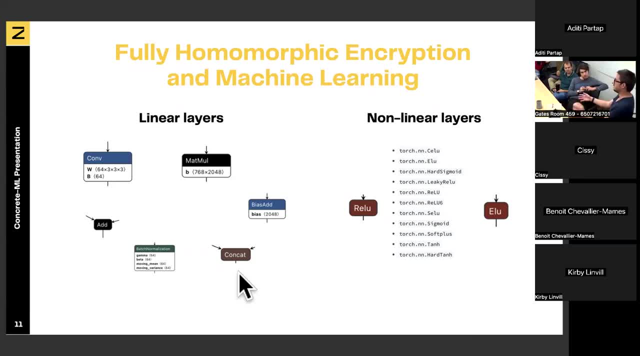 Okay, what we are presenting here is also ML case, but it's What we are doing at. Xamarin is more general. So, notably, we are working on something which is called Concrete Python, which allows you to return any Python program to the FHC equivalent. 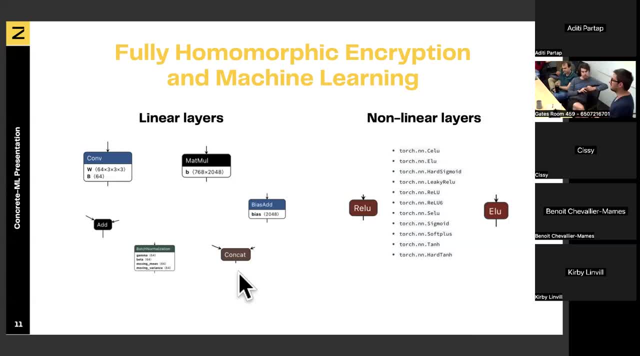 where maybe you don't have that kind of problems. Yeah, Are you happy with my question? Yeah, very happy. Okay, So you have your first Great, Awesome, Thank you. A follow-up question? Yes, Even more directly. 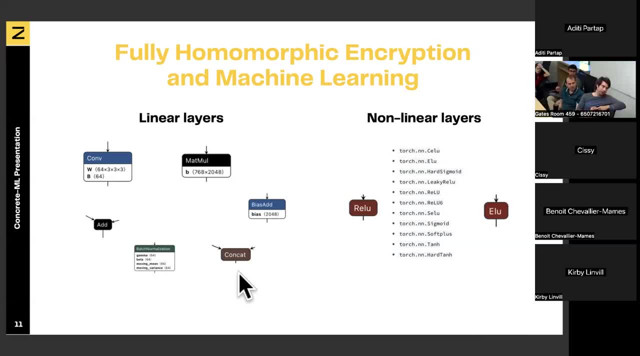 does the FHC game that you guys are building not provide function privacy? Function privacy- I'm not sure what. function privacy is Not natively, but we can build function privacy on top of it. That's not something that you're doing right now. 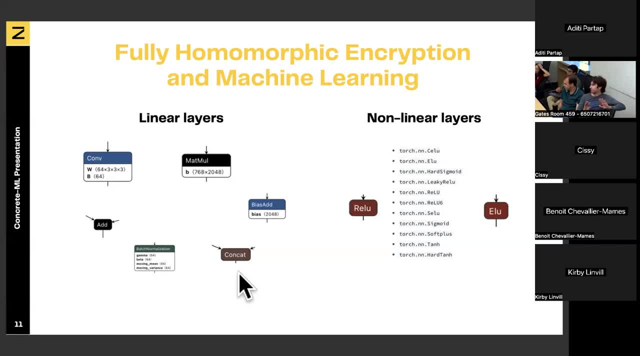 No, we're not working on this because this is not like the most urgent, of course, problem to crash, but we know we can get there. We can go there to work. yeah, So function is privacy when you want to obfuscate the function. 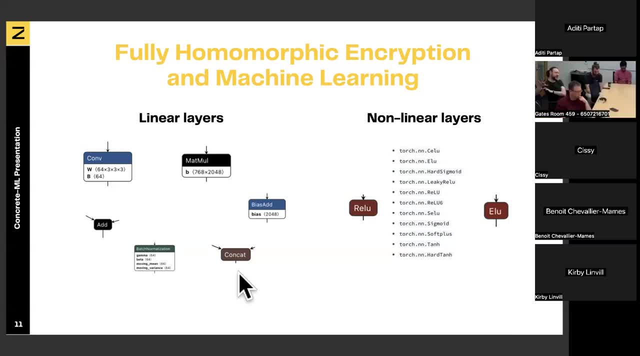 The function definition, The server itself will know the function. Okay, yes, So, yes, it's doable, So it's doable. So, for example, one thing which is quite easy to do is to encrypt the weights, So you don't protect the backbone itself. 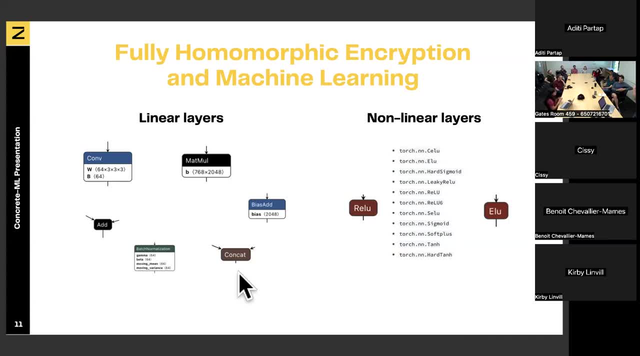 so the structure, but you protect the weights, But it would make FHC inferences much slower. Sorry, That is interesting. Well, that's not what I meant to ask about. What I meant to ask is there, I know where to work. 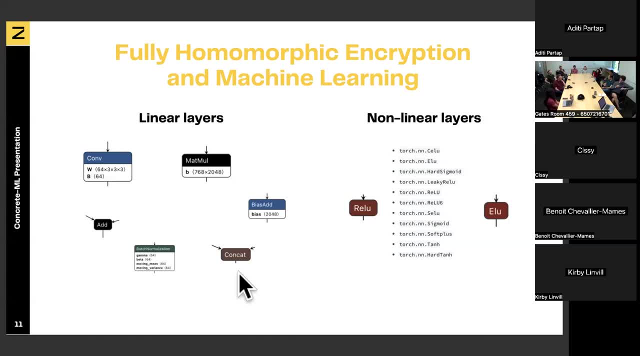 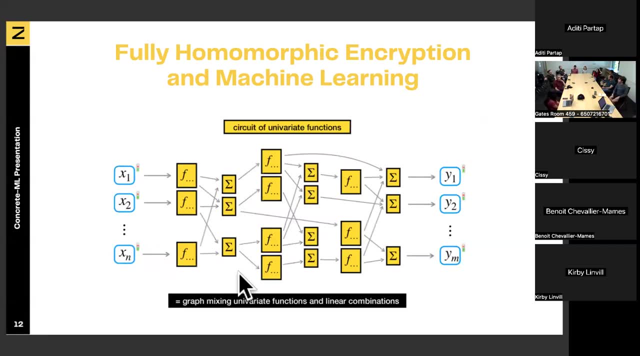 Okay, But the answer to that is also no. Yes, Yes, Absolutely. But I mean, if we're, In the end, all the computation has to be oblivious to what's the input, So you're kind of forced to use the circuit-like representation. 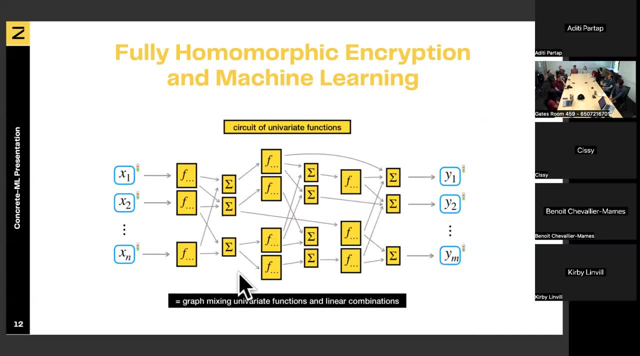 of your function And so you can have like- Because you could have like- a universal circuit and then provide an encrypted circuit as an input together with an input coming from the user. You can always research that, but of course there should be better ways. 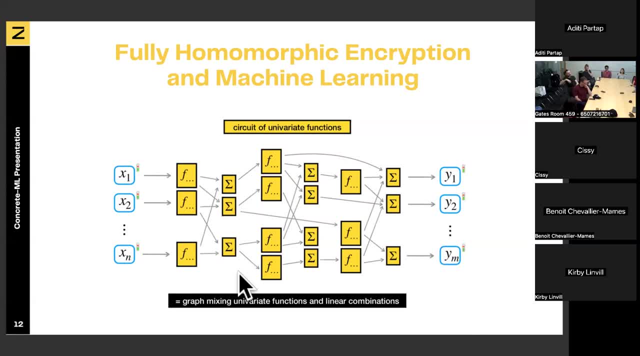 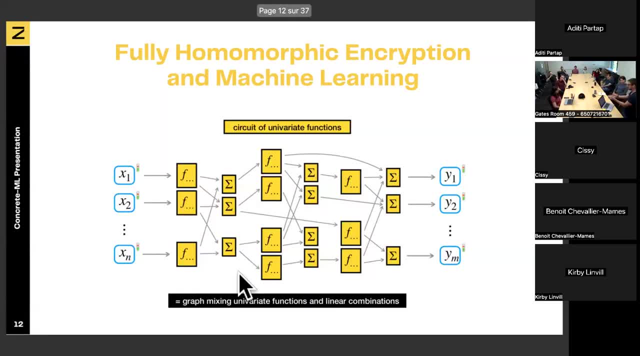 Sure, Sure, Okay, So now. so, as you can see, if you can imagine, this is a bit complicated to use that by hand. but we have explained, we'll have to do this, but you don't want to do it by hand. 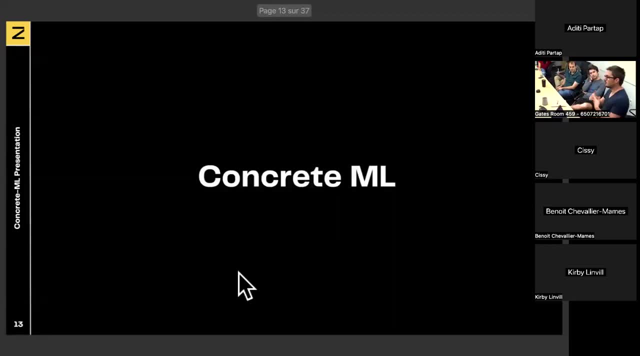 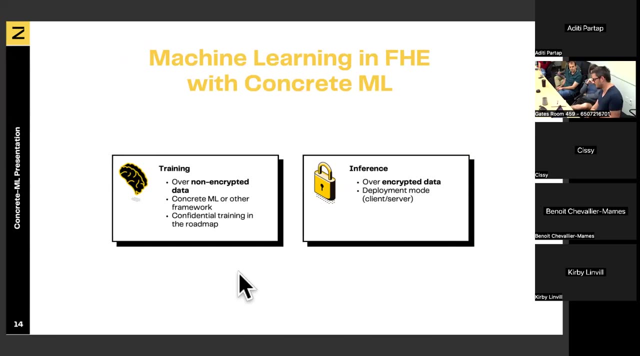 So we've done a product which is for the users. So our users are actually data scientists, Because maybe not- Okay, I will say just after, but maybe just after- what we are focused on for the moment is the inference, so we are protecting the inference. 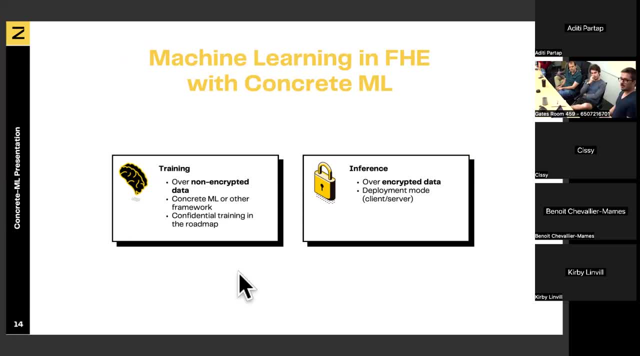 we are protecting the data of the user and we also give some functions to deploy this if you want to go in production or build your own company of values. and, notably, we are not working on a training for the moment for financial training, and so it's in the roadmap, but we have 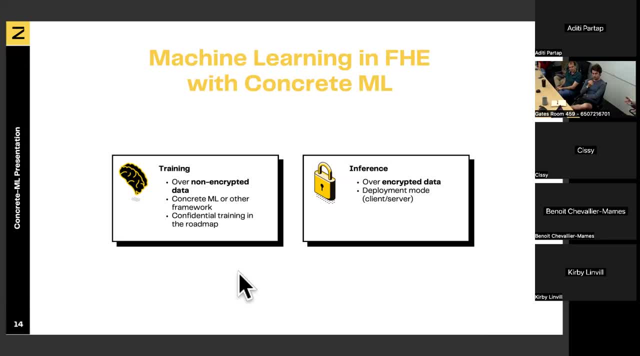 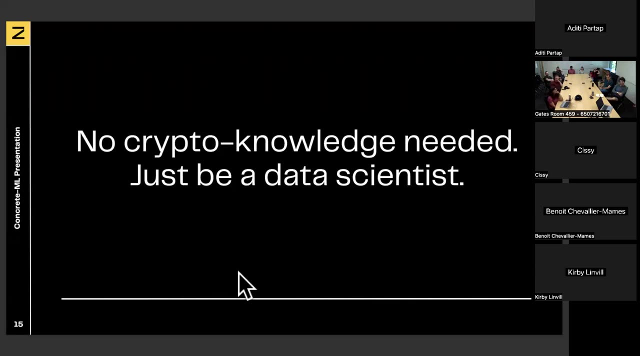 to choose a bit what we work on, but it's also possible in apache to do some training. it will also be quite long, but it's so. yes, sorry to say this. yeah, i mean, we want to make a product which is easy to use for the users, and the users are data scientists. 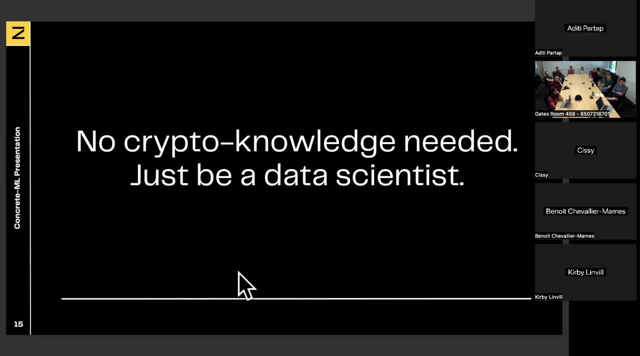 so we want them to. we want to blind the crypto for them. we don't want them to make mistakes. they shouldn't know what the pbs key or whatever. so more or less we just tell them this is included in that thing. so it will go into the details of the api. 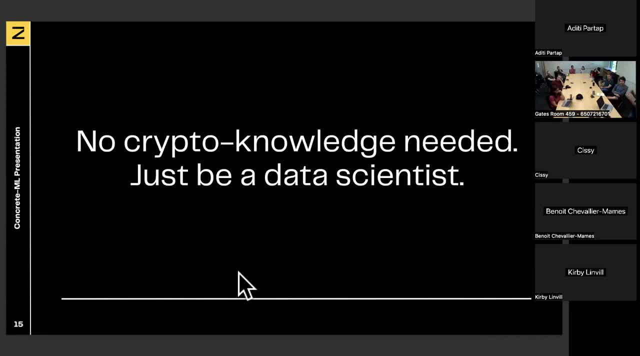 but you will see that it's quite easy and also it's not possible for the user to reduce the security parameters. obviously they they don't know. they would say it is going. it is much faster if i said just security. we don't let them do that kind of mistakes. um, also, so our users are very familiar. 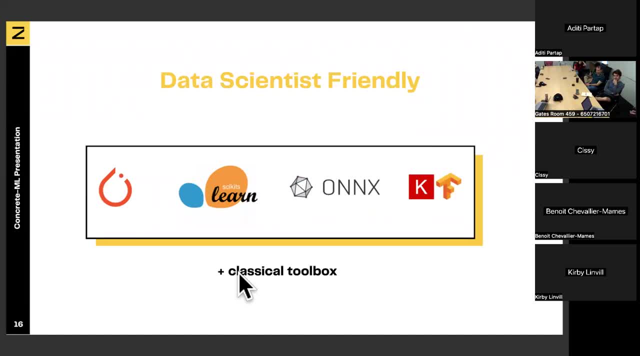 with terms, with psychic learn, with the analytics and the class and software. so we have made apis which are very close to them. uh, so if you have already done machine learning in the past, you are already able to use complete ml, and i'm not playing, so you will try and you will see this. 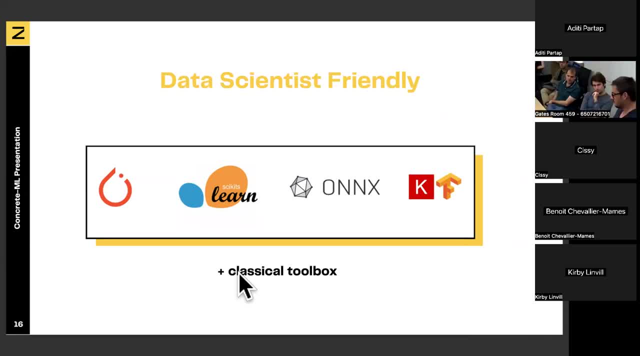 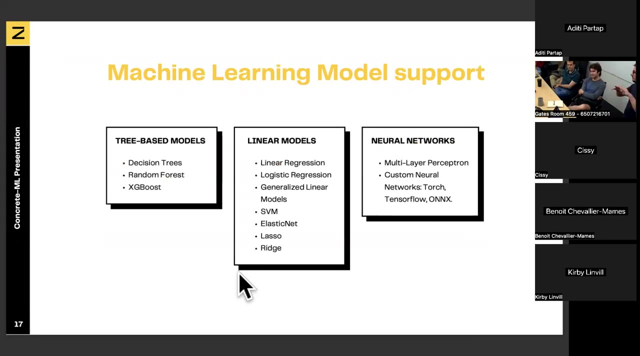 so we, we, uh, really the, the apis that we have are the same ones, and, for example, even for the feet we are using the speed of our system and my last slide before i let jordan. and so we have divided. we have divided the models into three categories, and so there is a linear model category, which is the easy one, so it's a filter. 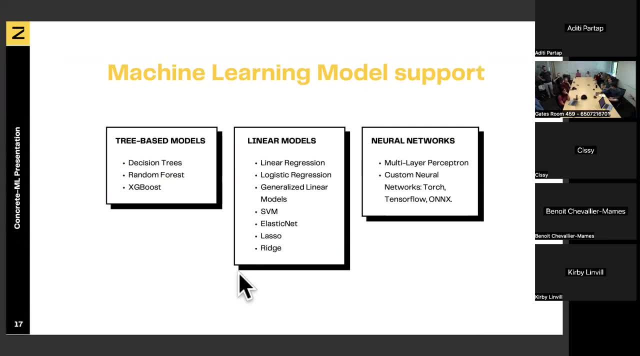 imaging that you have seen. so it's not really machine learning, but it's something which is linear. so same thing for machine learning. you have been in your impression and so on. this is very easy to do in fhe. there is no pbs, so it is very fast, it is very precise. 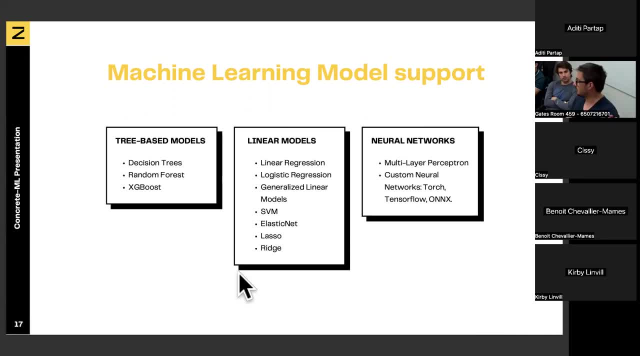 um, go on. then you have the three based uh models, so random forest issues. so it's another story. it's a bit more complicated. uh, there are some pbs there, so things that will be a bit slower. so it's not that slow, it's a matter of seconds maybe, which is much slower than in the clear, but it's uh. 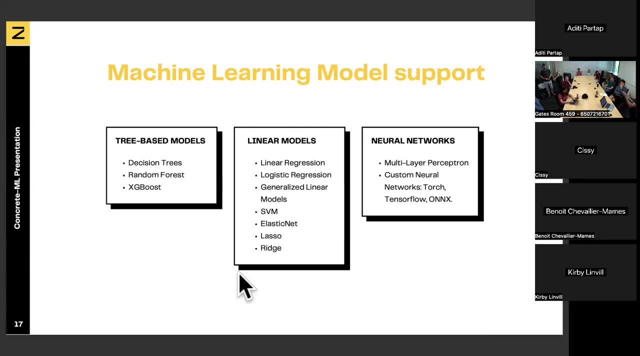 okay, and then in the last category. so it depends really a lot on about to um a data set, but if you are classifying something with a big data set, this is going to be a very long in a fish um. now jordan will explain you the details. 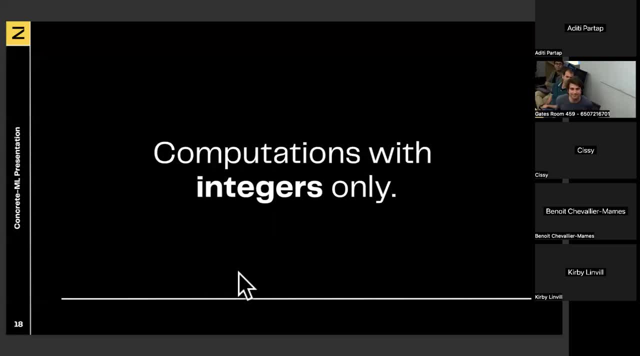 right. so yeah, so i'm from the machine learning side, so i'm going to be maybe quicker than i usually do here. uh, so when i joined them, uh, i'm basically in tall to uh um. so essentially to do in your classroom, where you take the data to learn to do uh what you've heard, uh fhe can essentially do anything, so it should be easy to remembergl. 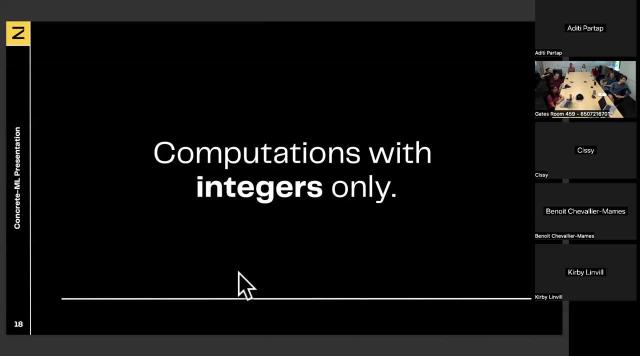 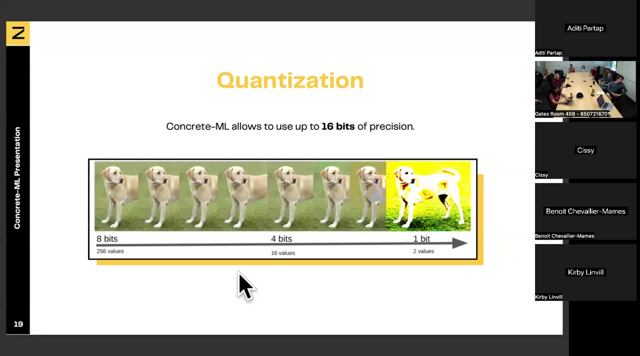 integers. So every single parameter in the model must be an integer And your variations, they must walk all on integers. So we basically have to map the floating point to the integer wall and make the model keep the same accuracy. So there is a domain which is taking off right. 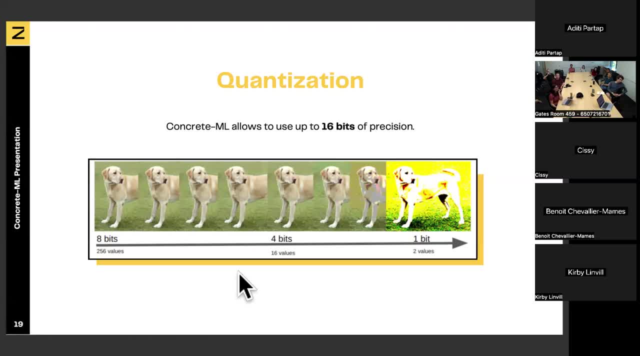 now, because of all this craziness about language models, It's called quantization. So essentially now, because we have billions parameters, models, people want to cut the cost of running those models, but they also want to run these models on standard hardware. So what happens is that 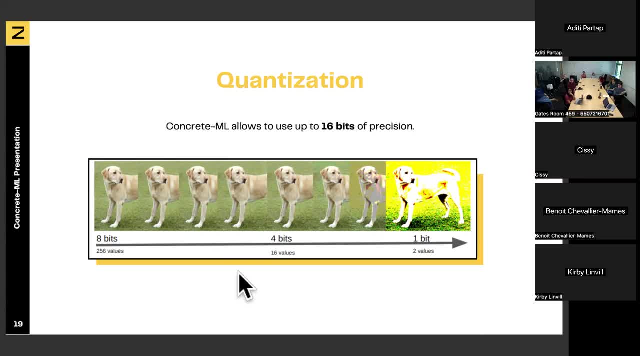 if you take this picture of a dog, a picture of every single pixel is represented with 256 values per channel, so RGB. What you can do is decrease the number of values per channel, so RGB. What you can do is decrease the number of values per channel, so RGB. 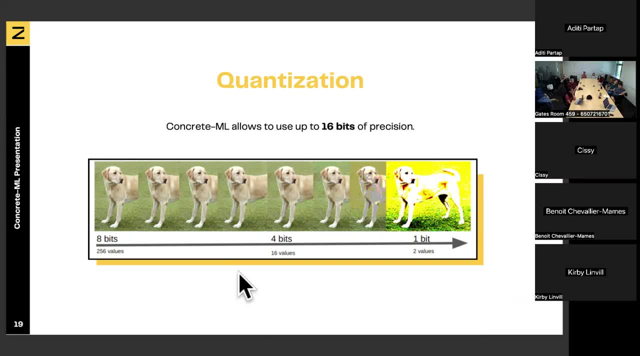 What you can do is decrease the number of values per channel, so RGB. What you can do is decrease the value available in the picture down to four or three bits And it takes quite some effort from your human eyes to see that there is a difference with the eight bits. So actually people realize. 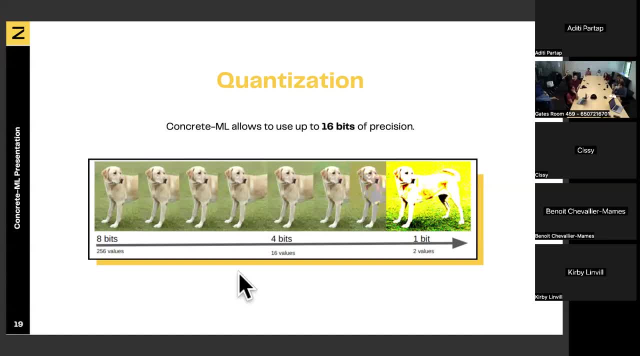 that machine learning models. they don't really need 32 bits floating points And you can essentially just decrease the precision quite a lot and the machine learning model can still behave properly regarding the accuracy. So that's a great part In concrete. so a year and a few months ago we had like six or seven bits of precision. Today, 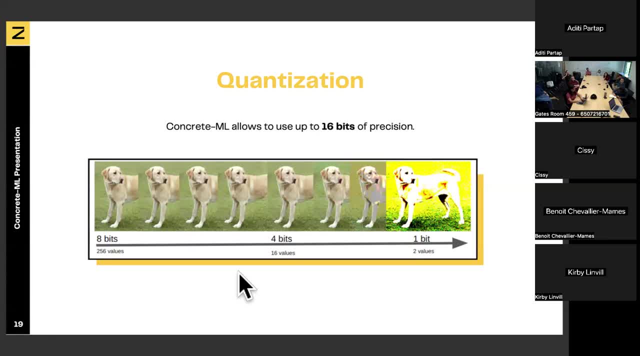 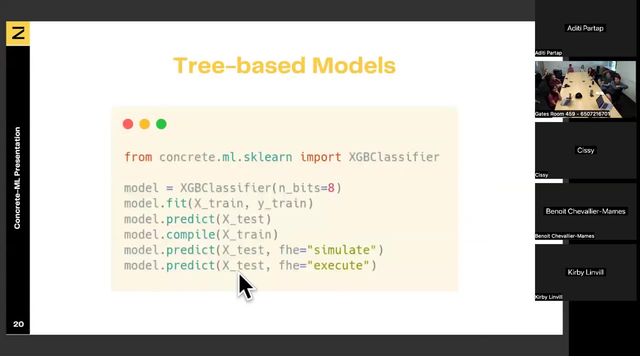 we are at 16 bits of precision, meaning that we cannot go over that threshold. That's the upper limit for now, for when there is a PBS in the circuit. So now let's look at the API, and I'm going to explain a bit. what are the specificities of this code? 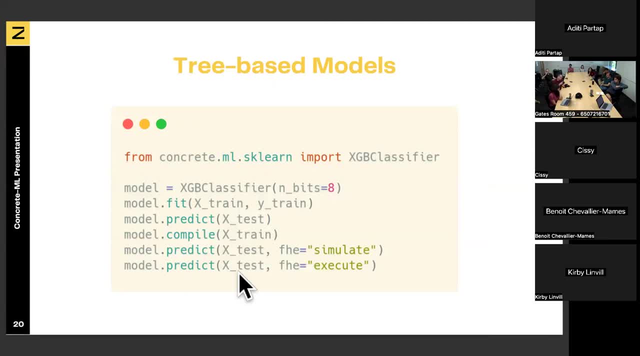 Actually, just to be clear, when you say specificity 16 bits, you mean that there's a wraparound if you go beyond. So if you add three 15-bit numbers you'll wrap around. So I'm not sure if it's a regular overflow. I think it's a negative. 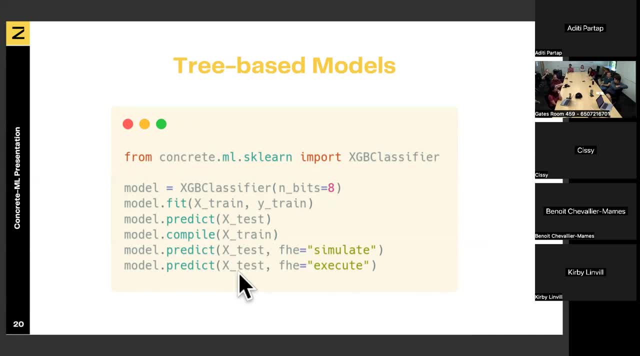 overflow. It's a saturated, isn't it? It's not saturated, It's not saturated, It's an overflow, But actually it's a compiler. So what we are doing, what you are using below it's undefined, So you are not supposed to overflow, Yeah. 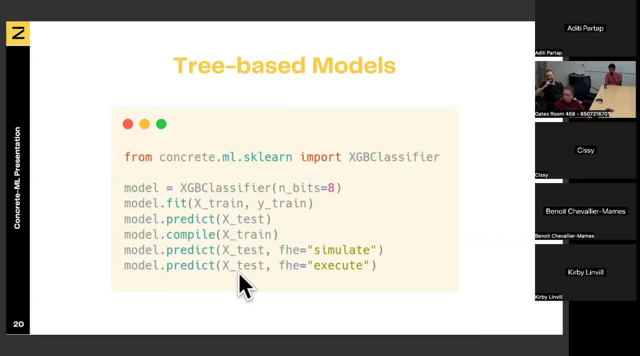 Oh, so, if I know it for real, Because there are different kinds of PBS, one with a bit of padding, one without, So you don't know what kind of PBS you're going to use, And if you have a bit of padding and you override it, 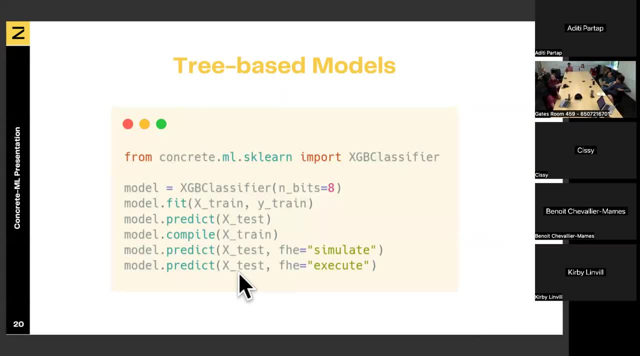 that means you have troubles. So it depends where you're overflowing in the circuit. But if you do that, when you are just doing the linear stuff, yeah, it's a wraparound, Because everything we do is modular power of two. So in the end you're just wrapping things around. But if you do that in the other part, 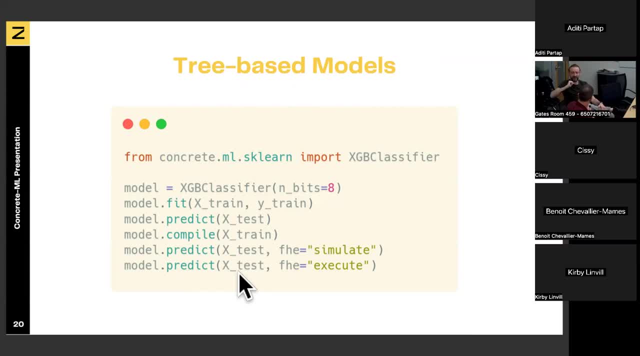 of the circuit. that's why we kind of force the fact that it's undefined, Because it's very hard to predict what's going to happen. So when you compile, we make sure that this never happens. And this is only art or morphic computation. 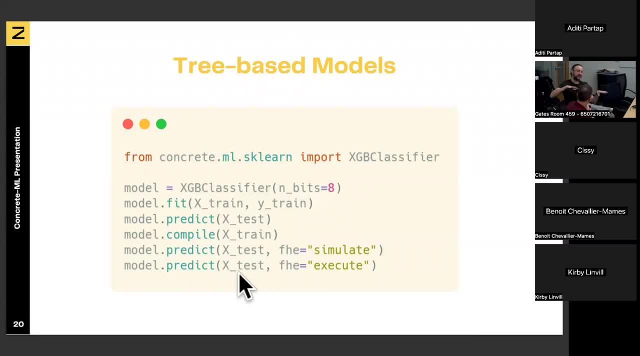 making sure that you're always. you're never losing the consistency of what you're doing. So when you go to undefined, when you decrypt, you actually Yeah right, You get undefined. Yeah Well, essentially you actually don't expect your production. 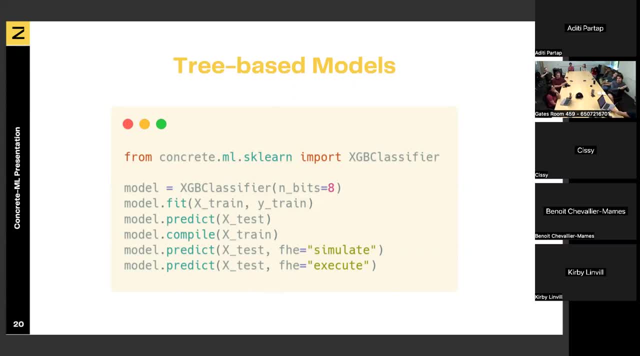 environment to be distributed similarly at your training. Hopefully this is what happens, And basically any theory. machine learning theory is then a chance, if you don't assume that, So yeah, So here, it's basically an API to call. It's basically an API to call. 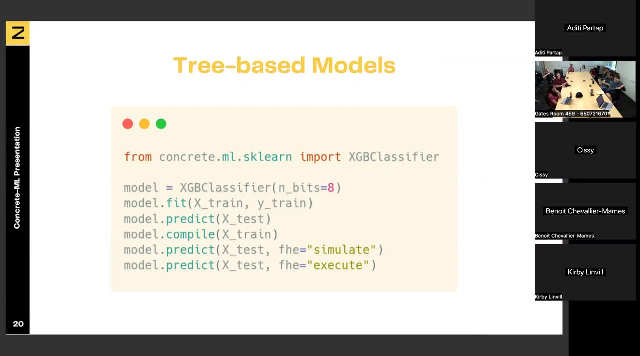 the gradient boosting. so it's essentially an ensemble of trees, lots of trees in there you can basically use. if you have used circuit learn before, this is very similar. the only thing that you have to do here is to set the number of bits. so you have to basically say: now my input. 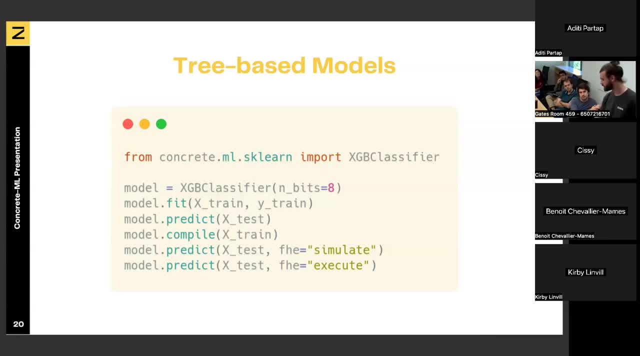 is over 8 bits and this number of bits is going to be important later. so here you have the predict function so you can test what happens. but you can, once you're happy, you can actually send the whole model that you trained and combine it to the hd equivalent, and here the the x train that you're. 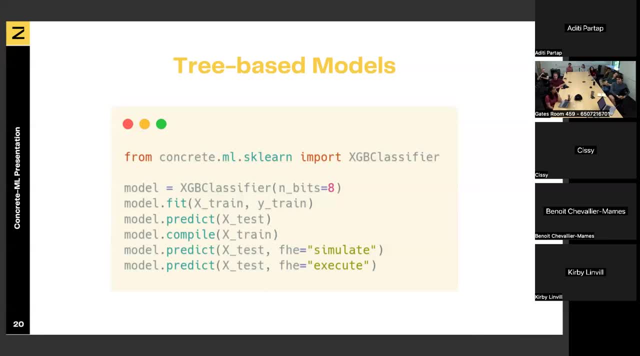 passing. the combining is basically going to be: all the ranges, uh, for the precision in your circuit, uh, that you don't want to, uh is 10 bits, a power of two or kind of arbitrary value less than 60. this is and this is going to be like to the power of eight. 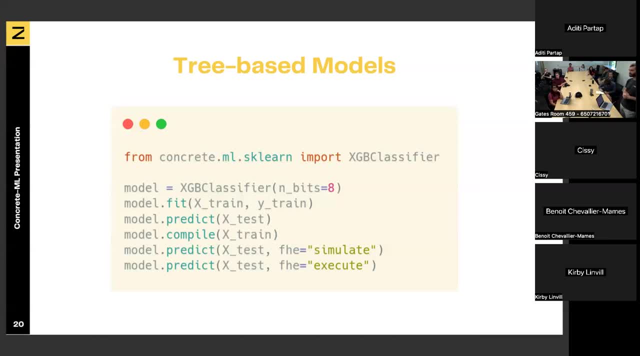 yeah, so this is the x one. yes, okay, yeah, yeah, exactly, uh, so here you're allowing the input to have 256 per feature. um, so, once you have compiled, you can basically, uh, we build this simulation because, uh, if you are benchmarking your model, maybe you don't want to pay the cost of fhe here. 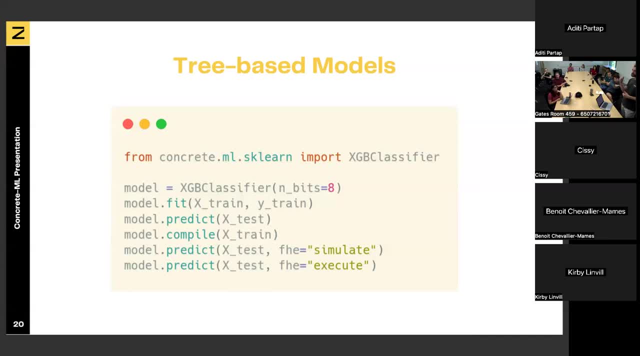 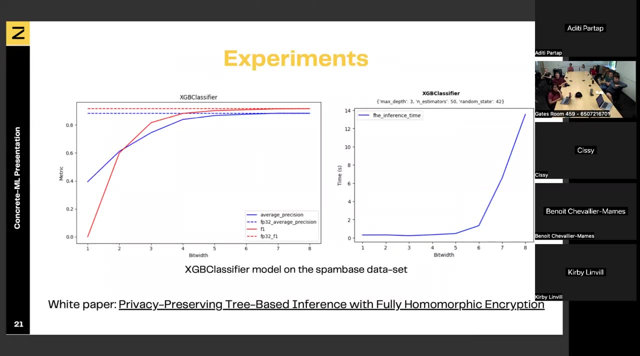 but once you're happy with that- uh, with the simulation, you should go into fhe, check the time- execution time- and the results are going to be the exact same as the simulation. so this number of bits is quite important here because it's going to be a trade-off between 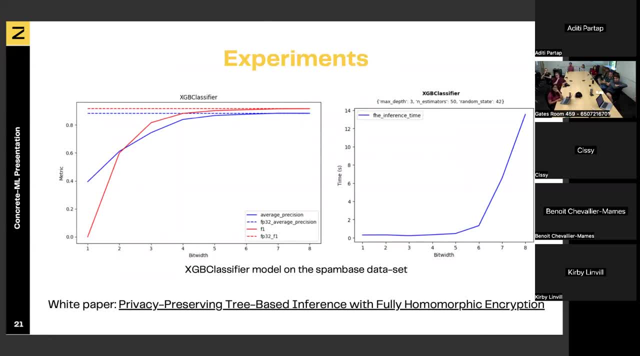 accuracy and execution time navigation. so basically, on the left figure you can see that we start with a bit width of one, just one bits of precision. random is pretty much random. uh, the model is pretty much random here, uh, because it doesn't have the input, doesn't have any of. 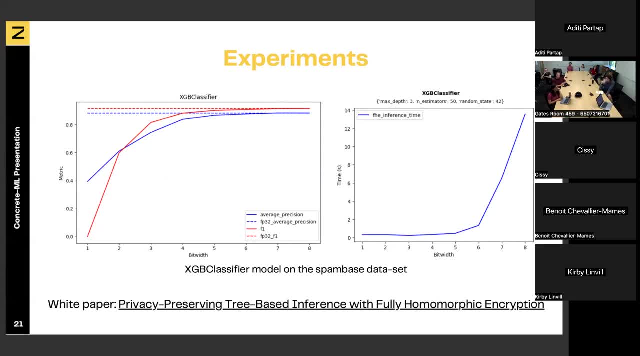 expressiveness to the degree achievement, uh. but if you go like, for example here, up to six bits, here you achieve like 99 percent uh match with the focal point mode. if you look at the right shot now, up to six bits, you are below the two second mark. so the whole model. so here it's like 50 trees with 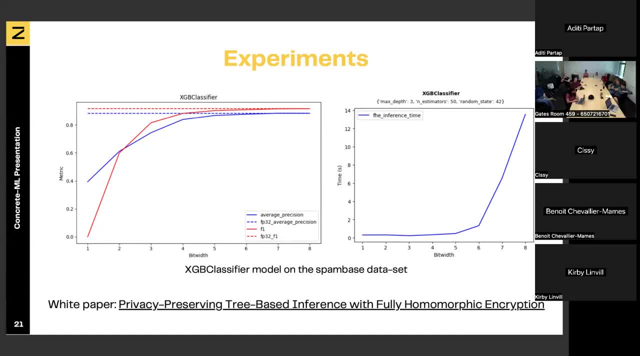 a depth of three and the whole model brain fhe under two second mark. if you want more inputs, uh, more bits here, uh, you can go all the way up 16, but you can see that execution time uh is going to increase. uh, quite a lot. is the algorithm paralyzing it is. it is so here we are talking about a tree. 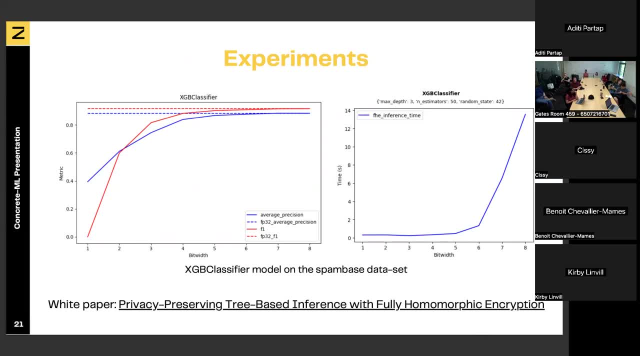 a tree is massively, uh, paralyzed, you can basically we have basically two steps of pbs so you can distribute everything, uh, and you have basically only two steps to do um and these. so about trees here. so we have a white paper where we explain how we do it. 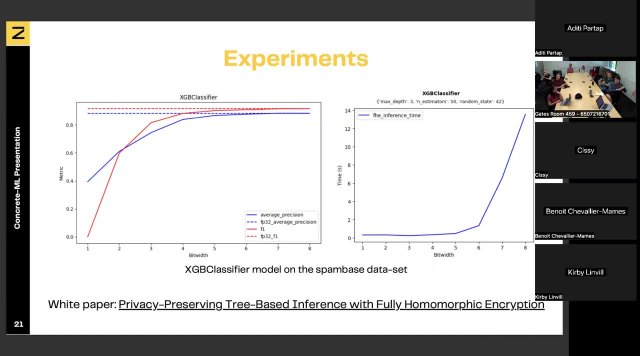 but essentially trees. you can't uh do the standard uh tree traversal, right the condition. if the condition is much, you go right, if the condition isn't much, you go left. this is not something you can do in fh, right? you don't know what's the encrypted inputs and you don't know 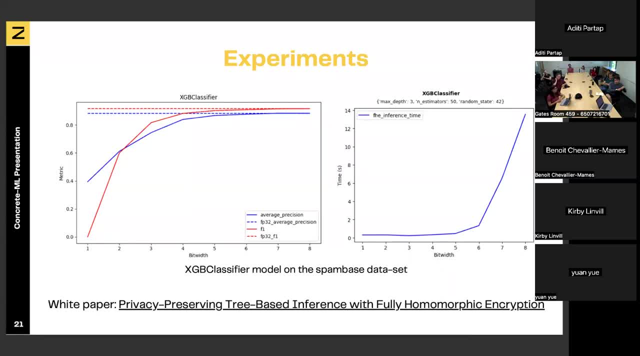 what's the result of the condition? uh, right, so what we do is to transform the tree traversal into serial matrix modifications, and what this implies is that you have to execute all the conditions from all the trees in your ensemble. uh, to actually know what's the answer, whatever it is. so now comes the linear models. 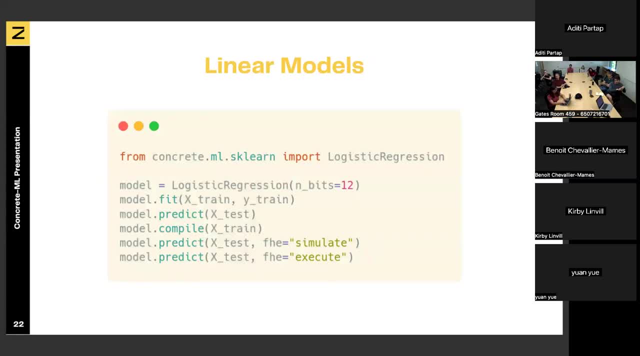 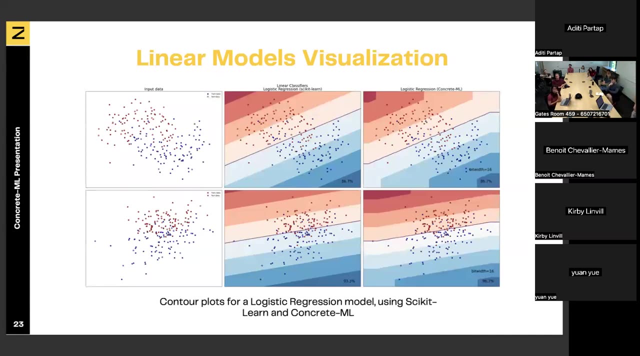 so, as bono mentioned, those are pretty um easy to to to run, they help superfrost and you can set more number, more bits than in any other model, because there is nothing to see. and, yeah, some visualization. so here are two random data set. you can see the floating point model. 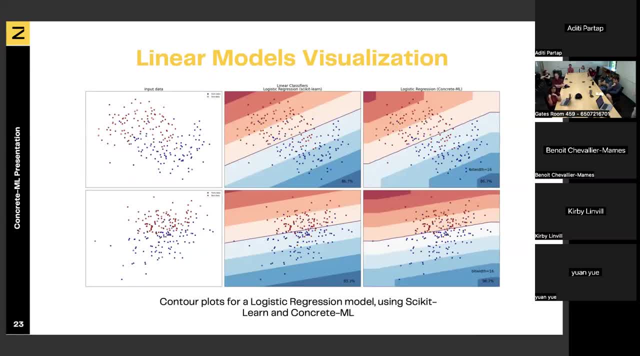 on the middle, uh, and on the right you can see the concrete ml linear model, which is a logistic regression here. um, so it's essentially equivalent in terms of accuracy, and you can see some artifacts which come from the fact that we are now using quantization and the model cannot predict. 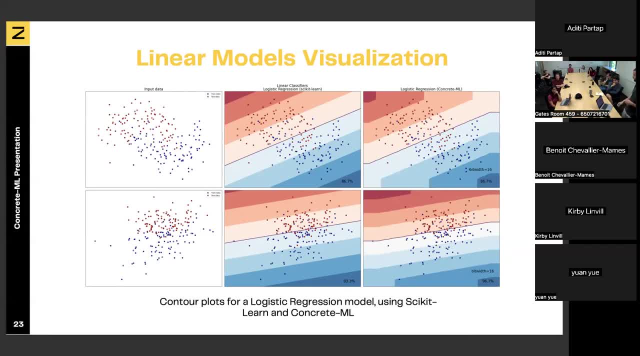 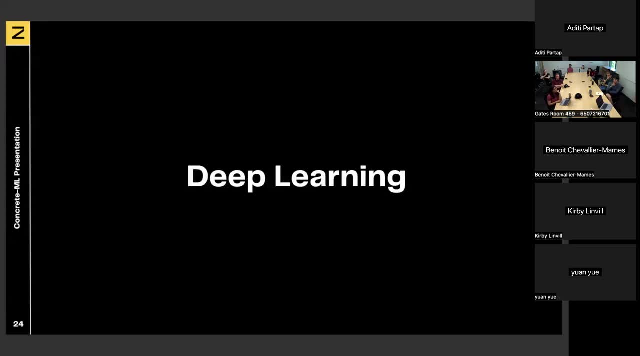 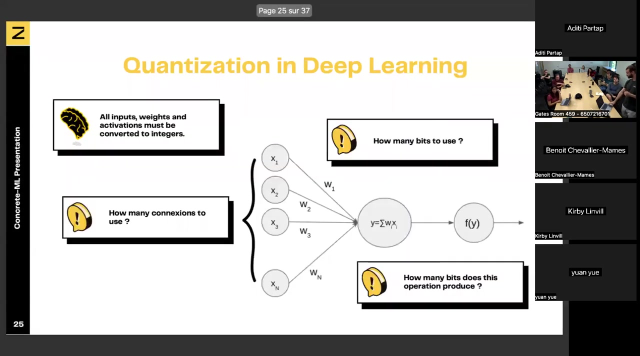 outside the boundaries, you get in the training, great. so the two models i presented: they are pretty uh fast, let's say in fhe linear on superfast tree based around the second, and uh, they are as accurate as the body points. now comes the deep running problems. actually, you can ask about trees, yeah. so if i understand, correctly. the the numbers you showed was 4.5 Axial이었 at some point and then they became 4.1. asal diagnoses on and on and the stick quarantined some consistent tree through. yeah, and everything's helping. but comparing thechw Interversal headaches and höhnle выше. 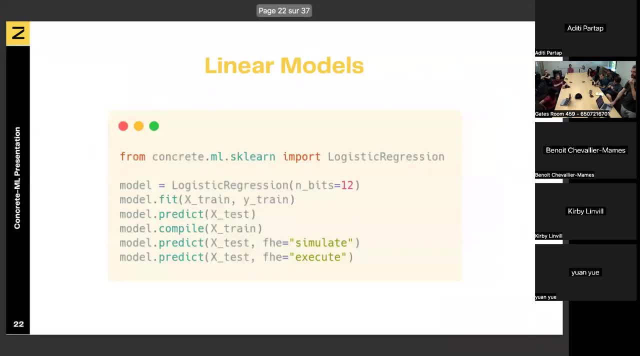 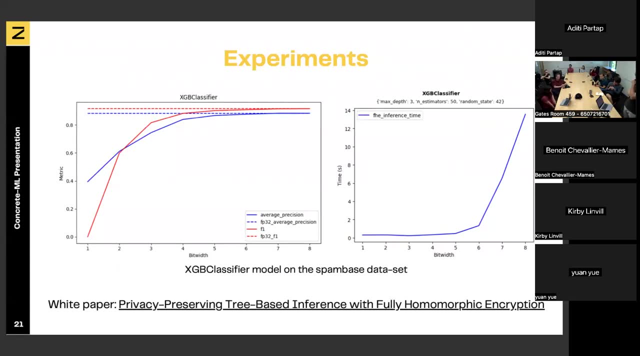 the boundaries and whatꔼ prays to manufacturinghorizontal defenses and deep learning button. so here's the keyы trees of depth three. Yeah, So trees when they're used in practice for data science. how big are they? Yeah, so here it's an XGBoost, so it's a gradient boosting classifier. 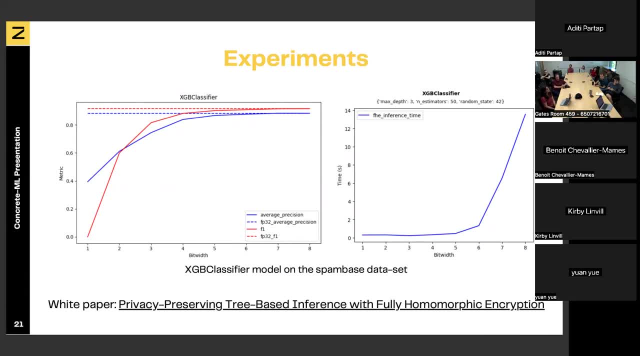 and in these ensembles, trees are not deemable. You need small trees but a lot of them, 50-100, like on the like, random forest, on the compulsory, Like they are. they need to be very deep and you need also a lot of trees, A random forest. you would pay them more, like basically: 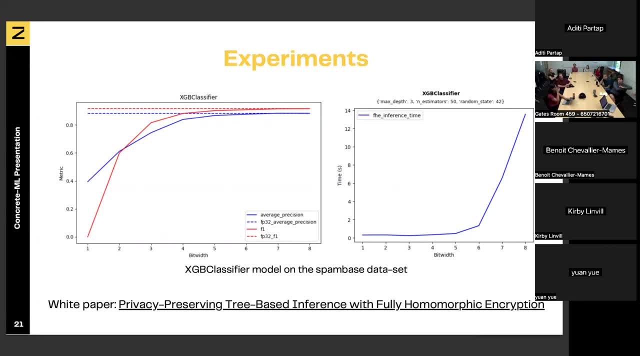 in FH, you wouldn't use a random forest because they are super costly compared to gradient boosting, which achieve, and gradient boosting has been proven to be like the reference in terms of machine learning based on trees. So you would. we use gradient boosting here, Yeah. 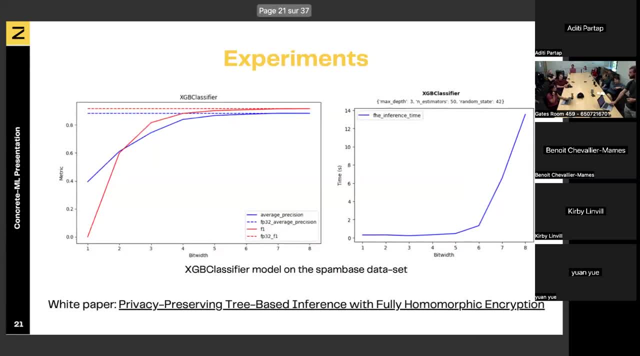 That's that. And light GBM is also based on gradient boosting. Sorry, Light GBM, Light GBM is exactly. yeah, It's gradient boosting. It's gradient boosting. Yeah, cool, Exactly yeah, Awesome, Sure. 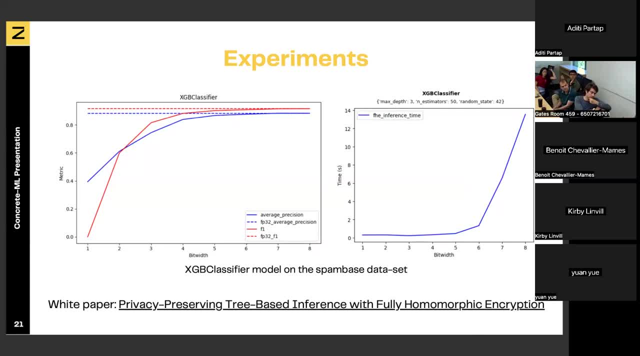 If you were to make a graph with respect to time, would that also be exponential? Yeah, so basically because you have, like, a number of tree which are a lot right, And because each depth is increasing by two nodes here, then because we are doing matrix multiplications now. 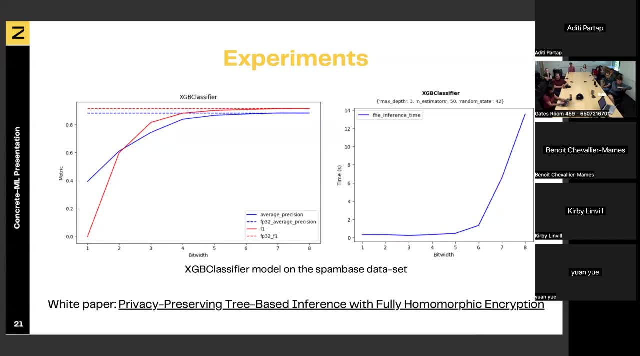 and not normal tree trodders. the matrices increase on both sides. Yeah, there's no pruning that you can do in the search. Yeah, yeah, And basically the matrices are full of zeros. But yeah, and zeros in FHE is as only a random number. 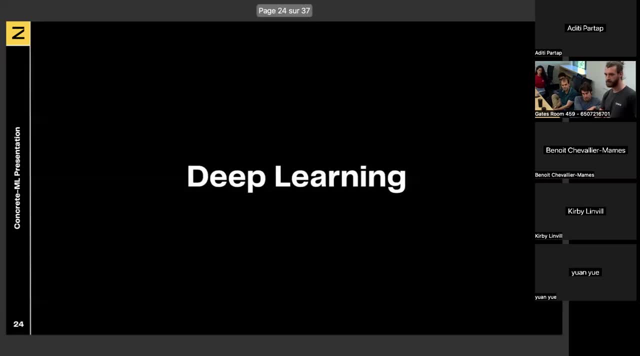 Okay, Okay, the normals. So on the tree, you can't use the shape in any sense to know that there are zeros As opposed to the data. I'm just wondering if the zeros are coming from the data or coming from the shape of the tree. 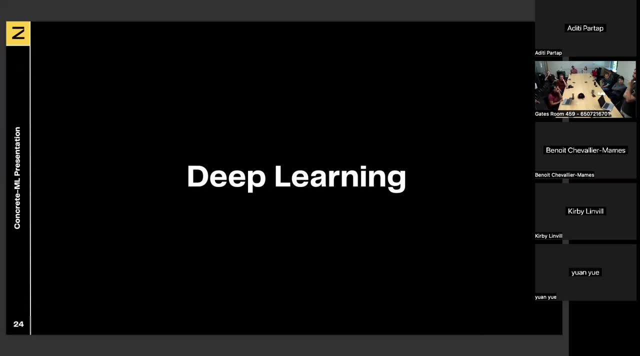 Yeah, they're coming from. you are actually right. Those are clear values. Yeah, there are clear values on this. So you could use sparse problems. Well, yeah, it's just we need to use sparse, For now we have the compiler. 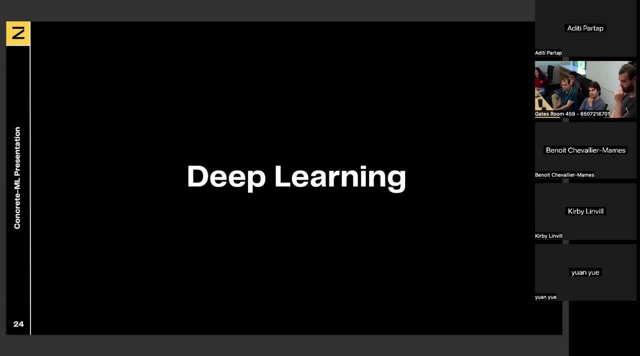 doesn't use any sparse speed improvement, but yes, at some point we should use that. Okay, Yes, Yeah, sparse multiplication in FHE would be really cool. That makes it sound like it's different. I mean, sparse multiplication is basically very trendy. 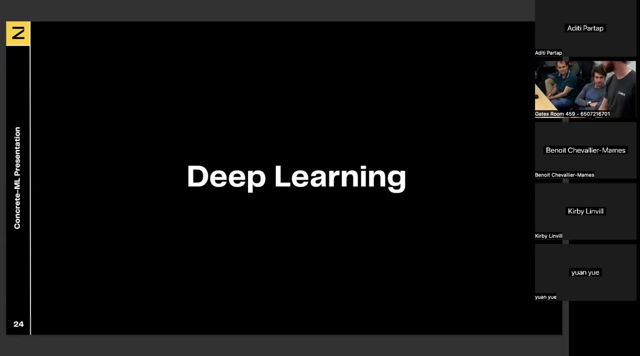 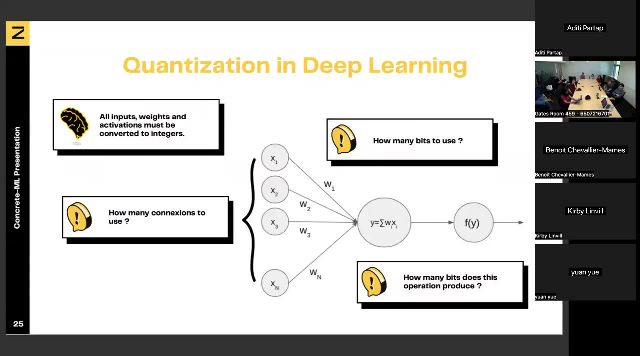 even in machine learning in general. Yeah, Because you know you've got tons of zeros everywhere. Yeah, okay, Deep learning. So why is this slightly more complicated than two previous model? I showed Well first. well, considering the size. 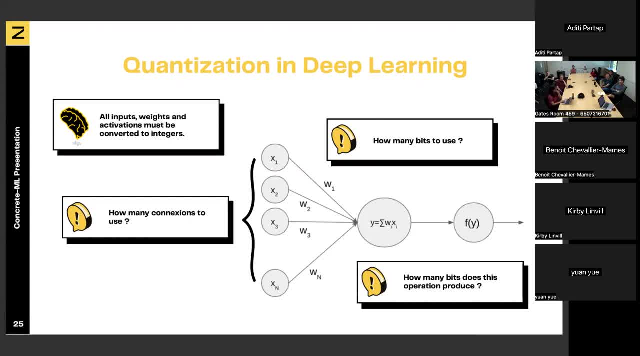 of the current machine learning models you can imagine. running them in FHE is quite a challenge but it's doable. And let's look at the challenges here. So if you take like the most simple part of neural nets, it's a little bit more complicated. 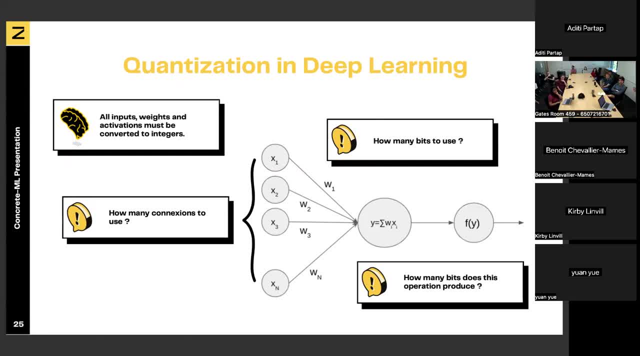 It's basically down to a single neuron, right Where a neuron is. basically, you take all the inputs attached to this neuron, you multiply that by all the weights accordingly to the connection, and then you sum everything into Y, which is now an accumulator. 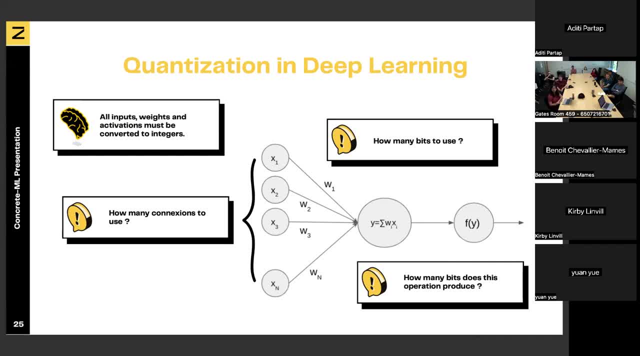 So the problem is, if you have tons of connections and you have quantized your inputs and your weights over two bits or three bits, then even though you have low precision here, this Y here is going to increase quite a lot, And more connection means higher. 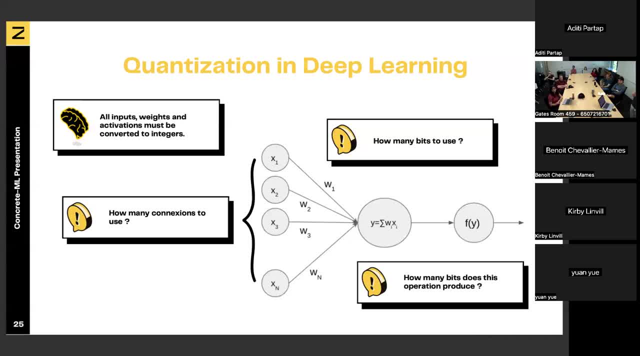 potentially higher Y data. So fortunately there is another trend in machine learning which will help us here is the pruning. So basically people realize that training machine learning models within sub-parameters generalize quite well, but at inference time we don't need these billions of parameters. 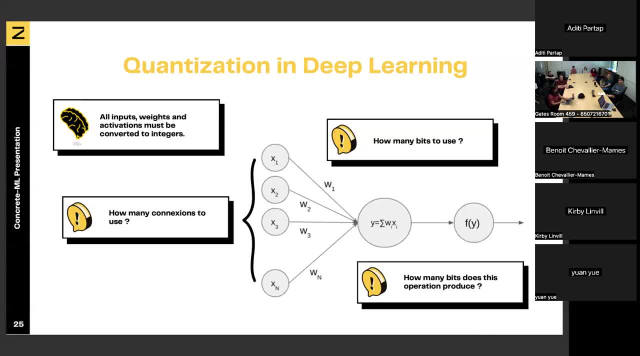 They actually like. more than 90% of those weights that have been driven are useless for the accuracy of the model, which is quite surprising. but very interesting because now you can just delete entire neurons and ease a lot the computations And this will help us because now we are going to prune. 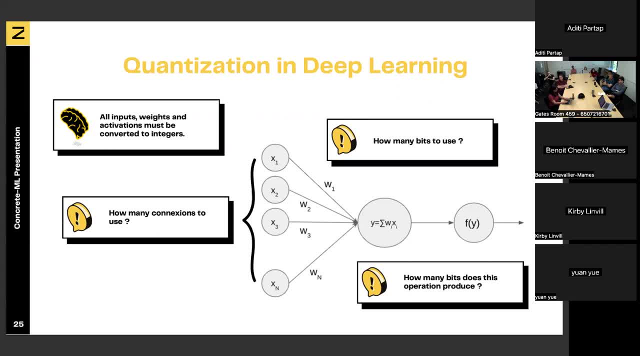 the model quite a lot, which will reduce the accuracy of this work here. But in general, a lot of them are zero. but aren't some neurons still have a lot of connections? Yeah, they have a lot of connections, but if 90% of them-. 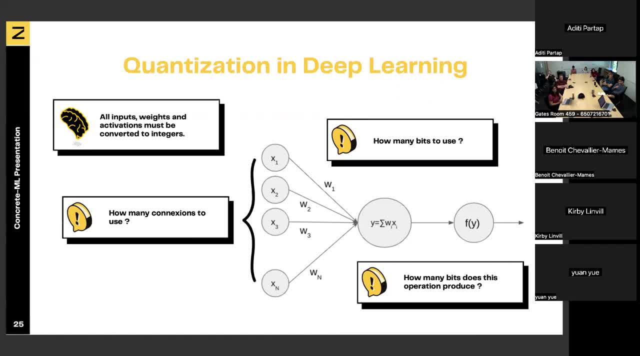 No, no, I said some of them have weight, have a lot of connections that have weights that matter. Many of them have one or two, but there will be some that will have a lot of significant inputs, And then you have the overall flow problem. 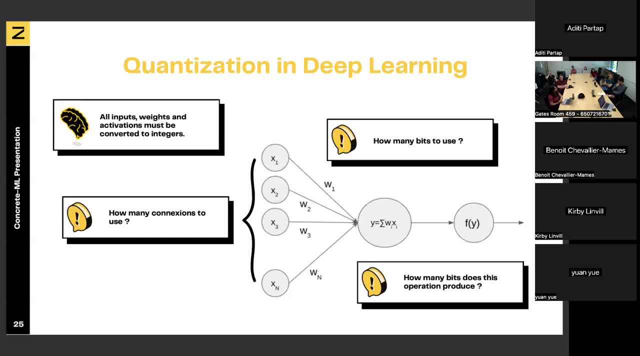 Well, the way we are pruning it is basically saying we don't want more than what we. you can compute the maximum number, theoretical number of activated weights, uh, different than zero, such that you don't want to follow it. okay, because normally you would just base it on the value, exactly. normally you would just take the. 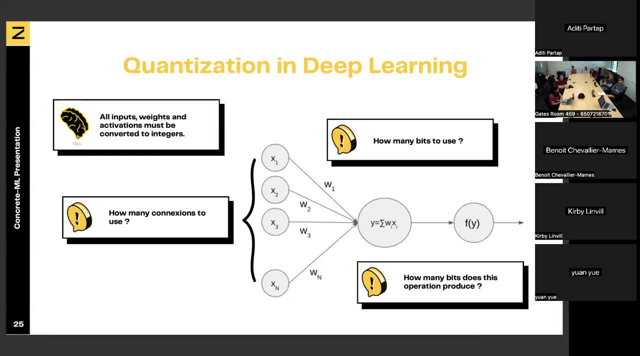 importance into account of the weights and then cut them um. you can actually do the thing during training such that when you cut our connections that are potentially more important than ours, the model can basically: uh, we train, we learn what we cut and we still get the same distribution. it's not obvious. yeah, it's just distributed over in the 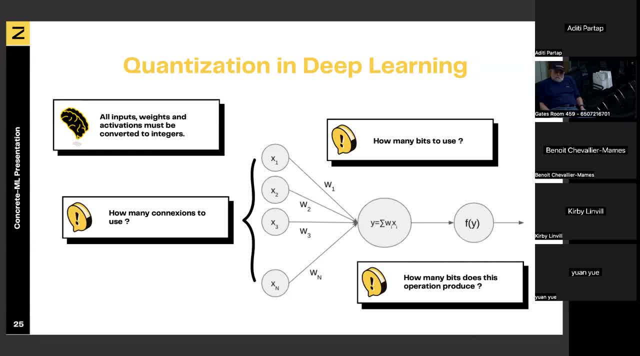 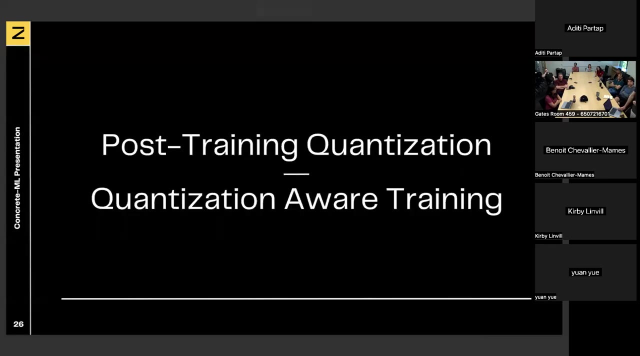 network, um and yeah so. so, yeah, there is quantization, pruning, and then, uh, basically, once y is in decent range, so basically from one bits to 16 bits, you just apply the pbs, so the f of y could be: so, yeah, machine learning. there is two ways. 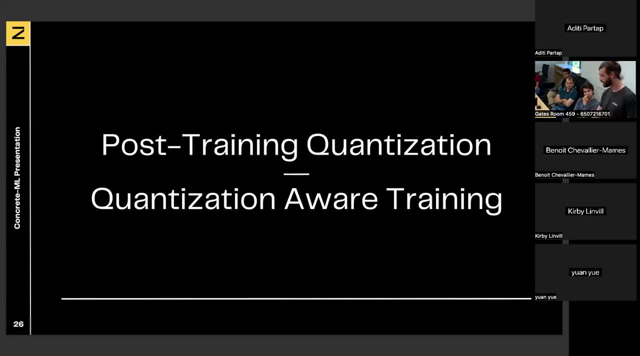 uh, into the integer ball. and the other way is basically: um, while you train or while you find your new model, you show that the model is being quantized. that way, when you back from packet, when you update all the parameters, then the updates take into account quantization. so you converge, your model converge. 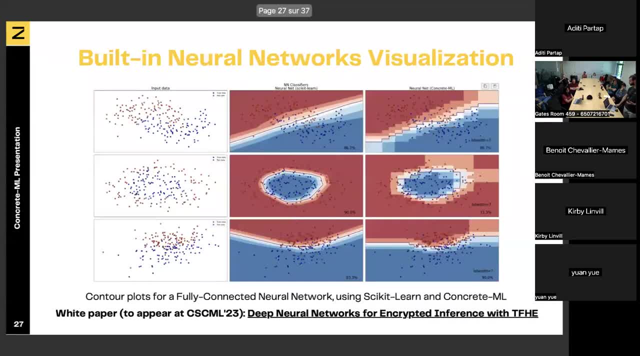 to a much better solution: quantize solution. so here just a visualization again. so you have in the middle the four points neural network, And here on the right you have the concrete neural net building which basically you can just start with two lines of code. 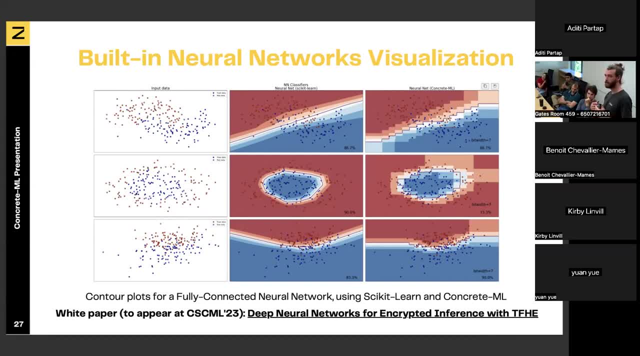 And here you can see that there are some quantization artifacts that are more present here. Because of this accumulation we had to reduce the number of bits in the inputs And in a way it's also to some degree. So you can see that in this text from quantization. 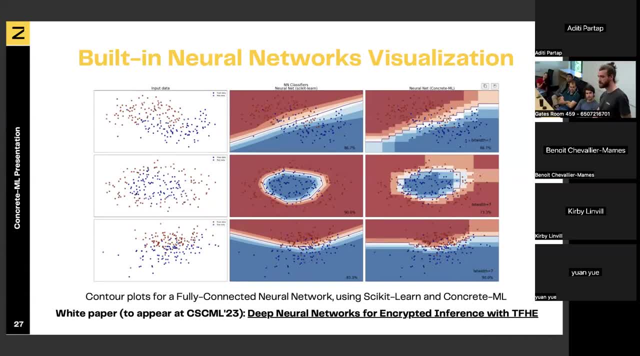 So the accuracy is pretty similar, but sometimes there are some jumps where you lose Right Because you are so low in order of precision. if you miss by a single value, sometimes you can impact the accuracy right. So there is a paper on this to explain. 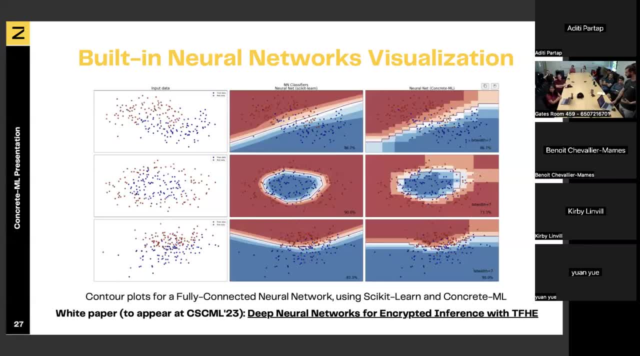 how we basically build them, all these VBS, and confuse them together. You can check it out. What were those percentages? accuracy numbers On the bottom right. yeah, it's the accuracy number. Oh, wait, It increased in the last case. 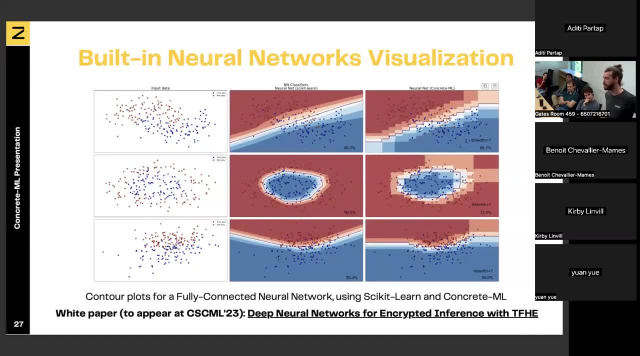 So there is a funny thing coming with quantization, which we did not want at first, but it happens. It's basically how it's: regularizing the model, Because you are quantizing, the model cannot overfit as much as it could before. 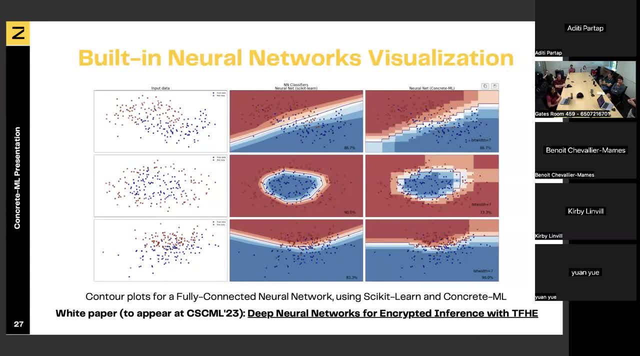 And suddenly we have some kind of yeah, but this It's not something we wanted to do, but sometimes it happens. Now, do you adjust the tables to account for the discretization effects, or just their straight calculation? Yeah, discretization and quantization: yeah. 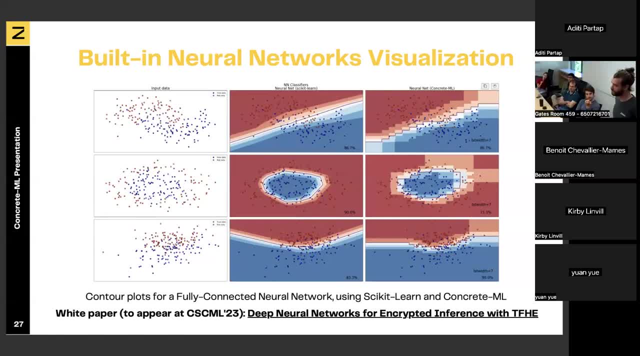 In the VBS tables. Yeah, yeah, You could adjust for known quantizations that were going to happen. So if the exact value would say it's this value, you know, because of quantization, you'll get a better result. You can make it slightly different. 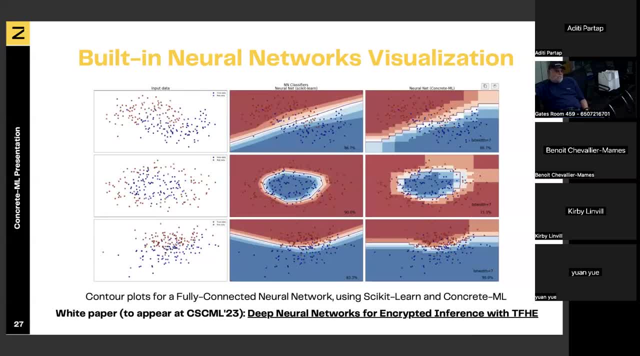 Can you do that? Yeah, yeah, Exactly. we do this. Yeah, We quantize, We put everything in integer and table lookup that is created is exactly what you want. Stanford Security's meeting is saying that when you do AI. 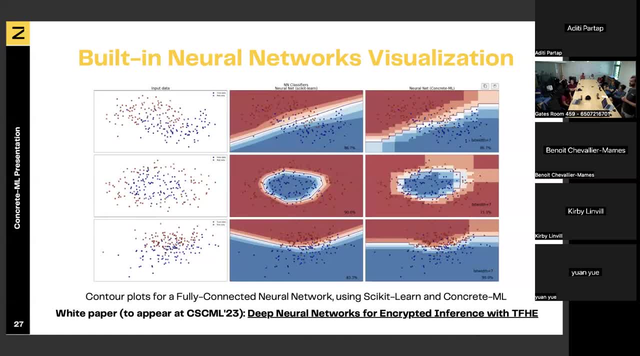 you can first encrypt the data and then do AI. Do you think AI needs to do a lot of calculations? How would you know what to do if you don't know the original data? You can encrypt the data and then it can do AI. 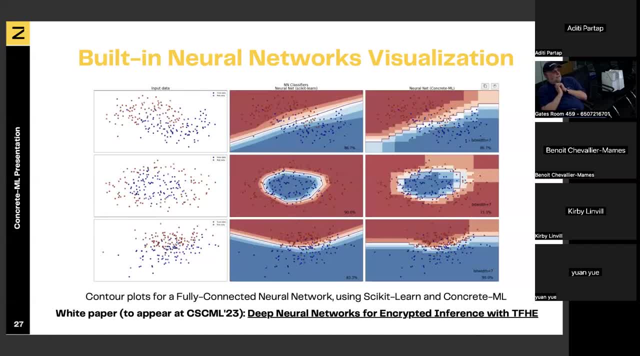 Yeah, And then you can make the first guess worse and then you can get a better result. One interesting topic is actually learning this table, But this is another topic. OK, yeah, that would be interesting. Yeah, I wanted to mention quantization-aware training. 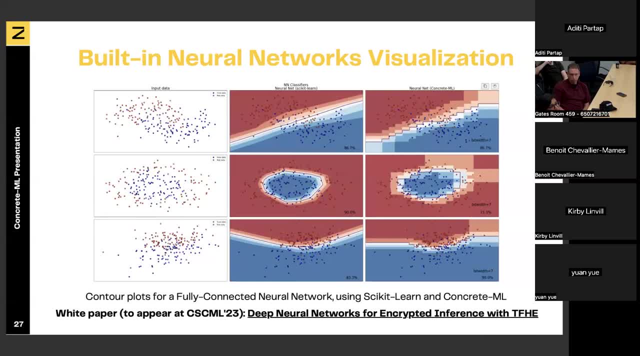 right, Yeah, Yeah, I'm guessing you could potentially learn the table that way, right? Quantization-aware training, I guess in some way, is sort of learning the table in some sense. right, Yeah, yeah, exactly Yeah. 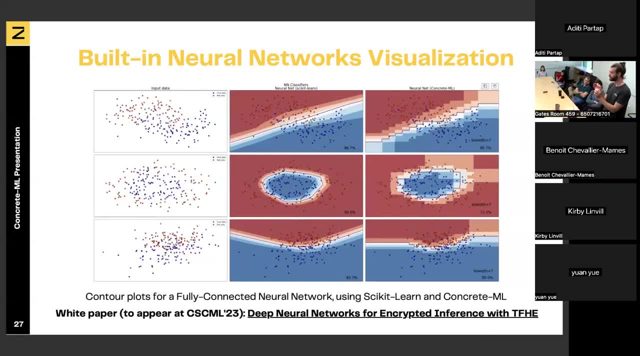 But sometimes maybe the table. when you're on the border you can quantize one way or another. We don't account for this kind of mistake And if you have a lot of you don't know where to go, then you could make some losses here. 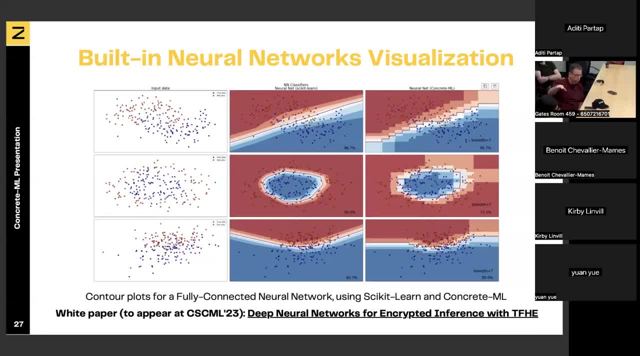 But the training that you do now is full floating point or you train with quantization-aware? Yeah, so the full training is at inference time. we quantize everything And the training time At training time. yeah, So you do the inference right. 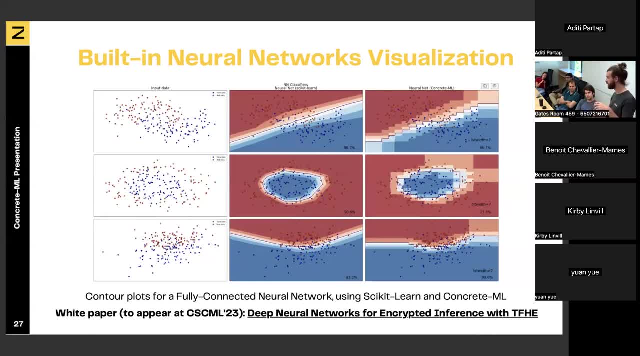 Everything is quantized. You do the inference and then you get some right. You can compute all the gradients. The gradients, you apply them to the floating points. So you keep the floating points in the model right And at each inference you basically apply quantization. 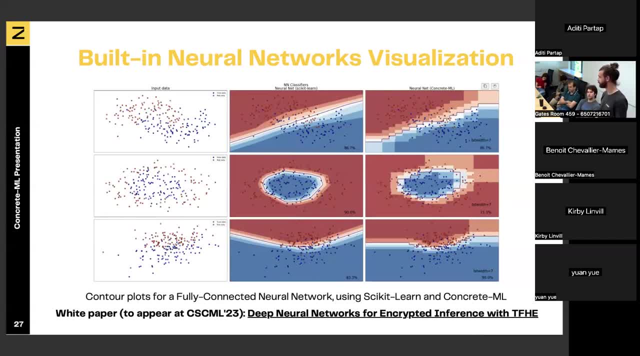 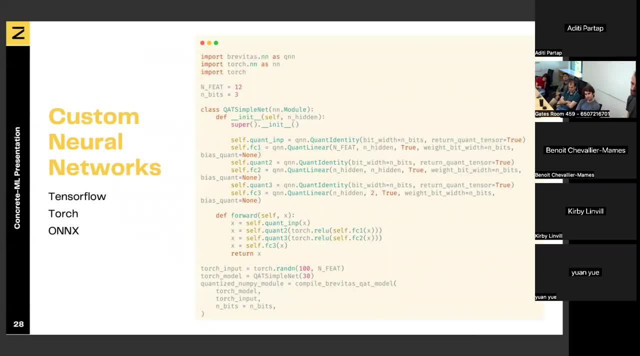 and you show: OK, you're going to be quantized like that: Adapt your weight, Got it OK. So the final thing is: well, if you are feeling well with the torch libraries, then of course you can build your own neural net. 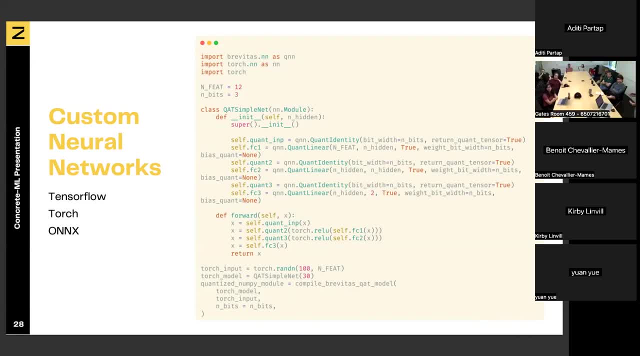 So we are friendly with a library called Gravitas which does quantization-aware training. It's basically just specific layers that allow this quantization-aware training. You just set a number of bits and then every inference, everything is quantized with the number of bits you put there. 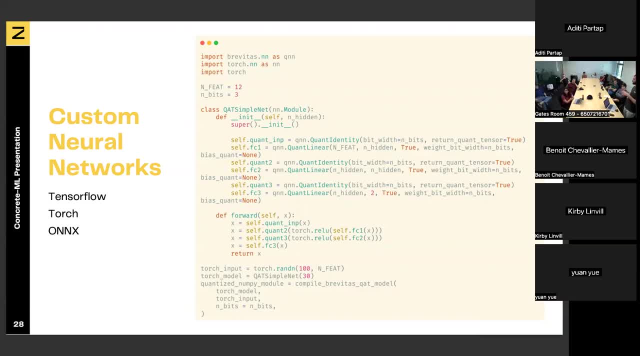 And when you backpropagate, there is some tricks, such that you update the floating points and then you can go on. So once you have done this and you have your model ready, now there is nothing that should change from this model that you built to the FHE model. 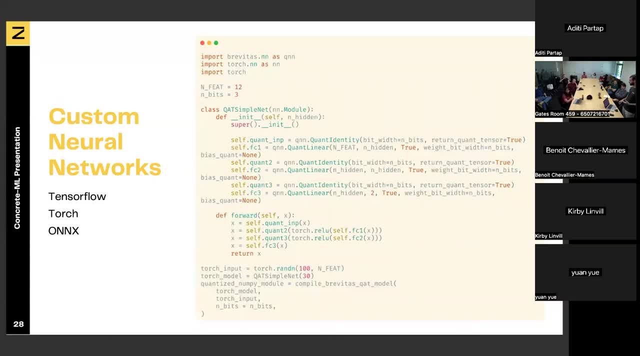 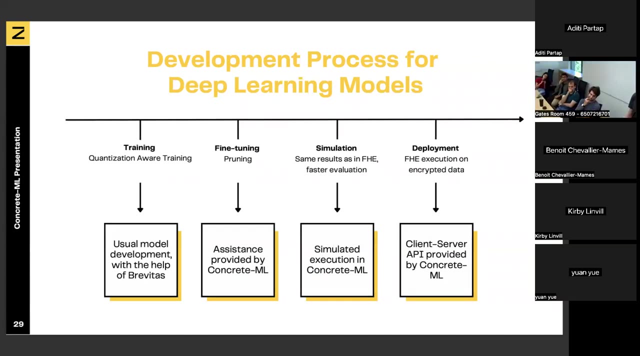 You can just call the function, put your torch model there, some inputs to represent all the boundaries in the model in terms of precision, and then you get the FHE model. Good Yeah, so the development process for different models. essentially you just, or you can train the model yourself. 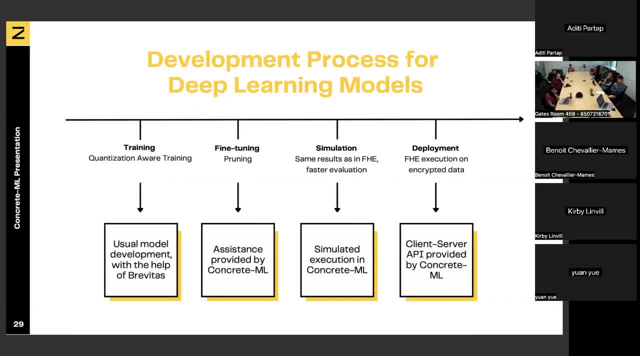 with quantization-aware training. But you could also just take a pre-trained model on the internet. So we have an example of this in the repo. Basically, we pull a model that does well on ImageNet and we fine-tune it with quantization-aware training. 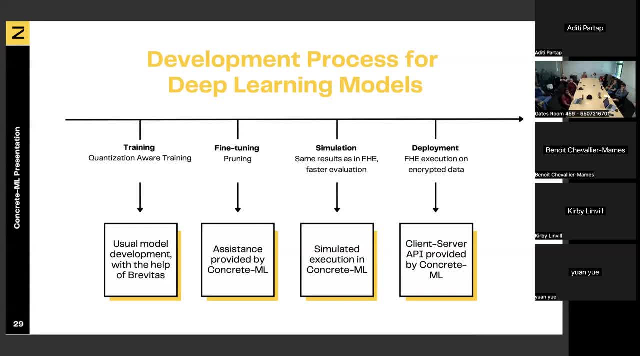 on another task And in the end you get your final model that runs in there. Good, So you can do simulations. Simulation is very important because once you want to check the accuracy of your model over lots of data points, you're going to have to do the simulation. 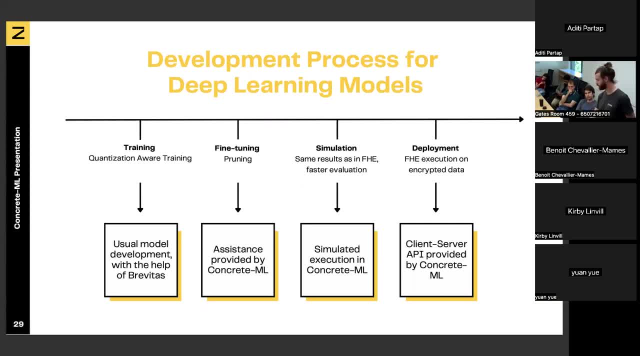 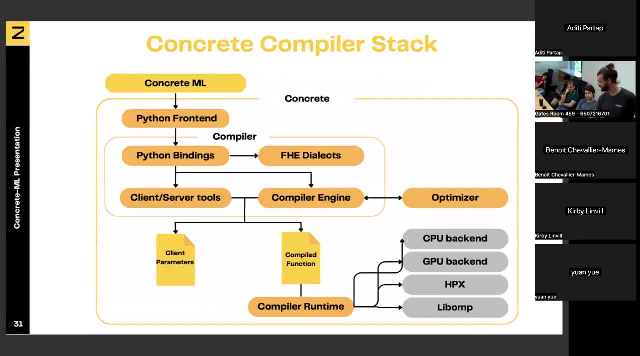 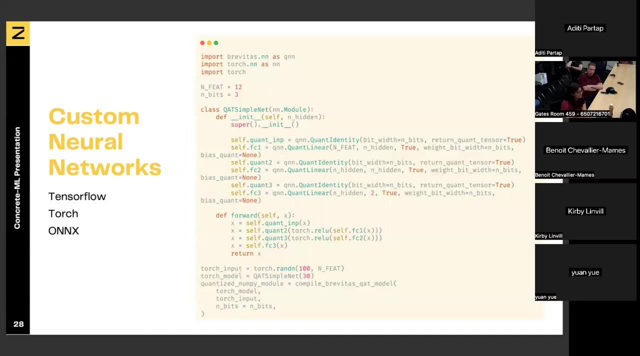 And then you can basically split all the client-side stuff and just go through the files. And there's a question from Isaac May. I know if the input data is also quantized during inferencing. The input data is always quantized. But yeah, in FHE the input data is always quantized. 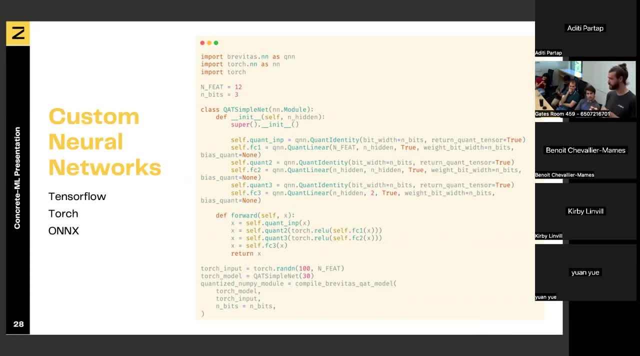 But this is done in the client part, right, We have some pre-processing. Basically, we take the voting points from the user and we transfer them to the integer, And you need to stop before the encryption. Exactly, The encryption is done over integer. 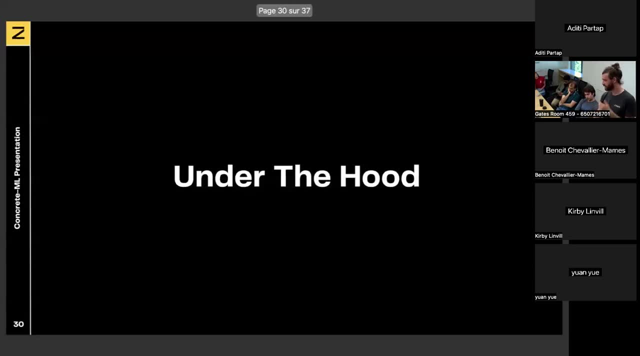 so it must happen on the client side. So how does the performance scale with the number of bits? if I went from 8 to 16 and then 16 to 32.. How would it scale The performance or the occur- Yeah, the runtime of a given. 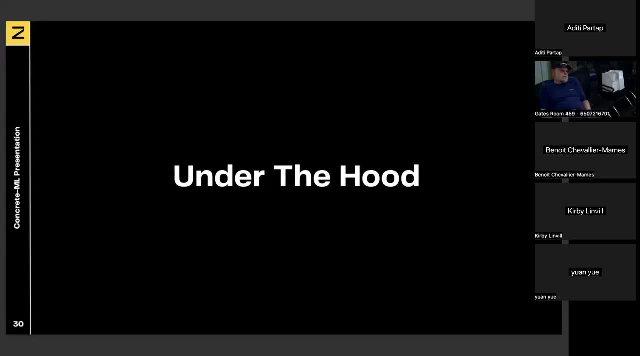 Yeah, so it increases quite a lot, especially when Exponential. Yeah, I'm not sure about this. It depends on the model, because we will have models that basically, you cannot distribute them completely. So, yeah, what we see is that if you are under 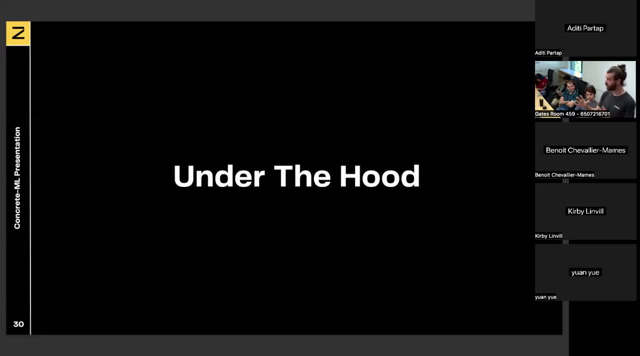 this seven bits of precision max in the whole circuit, then it's very, it's kind of stable, right, But then it goes, it increases quite exponentially. yeah, So you want the lowest bits, OK, so back to the last few slides. 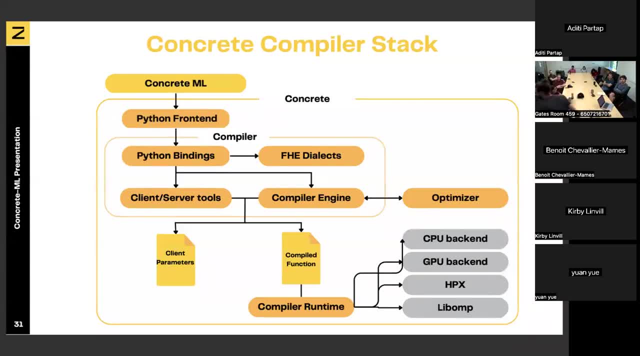 So how does it work? And I don't Oops, So how does it work under the hood? So in the company we are making a few tools. So we have many spoken about Concrete ML, But actually Concrete ML is just one thing. 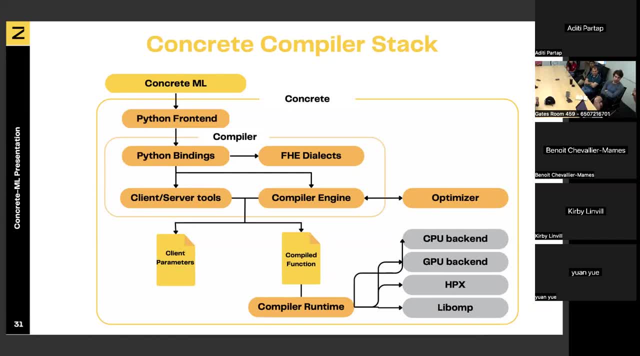 And it's built on another big thing, which is the concrete. So concrete is more or less two things. So let's start with the compiler. So it's a compiler made with MLIR, So maybe you know what MLIR is. Or if you know what LLFVM is, it's about the same thing. 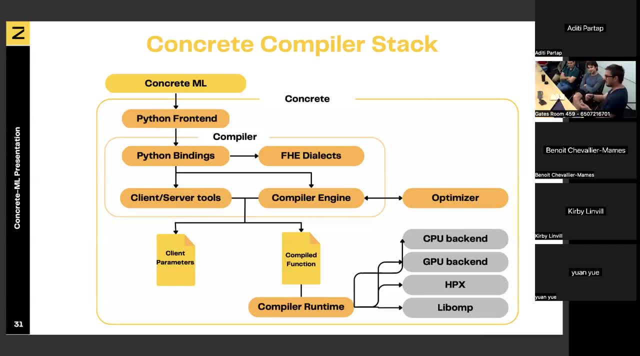 So there they are turning some program into the FHC equivalent, with some steps. I don't know the details, But maybe if you have questions, ask them. Then there is an optimizer. So here they give the program to this optimizer. 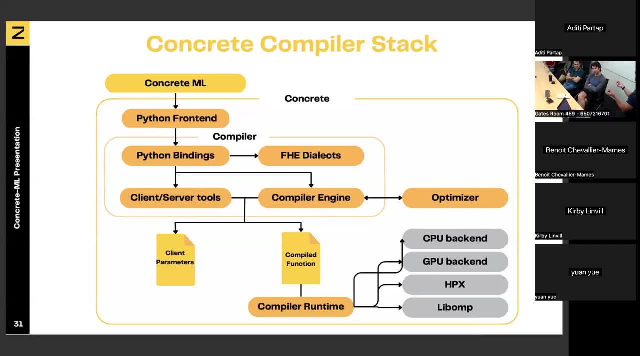 which is responsible of finding the best cryptoparameters. So they are going to search, OK, OK, In the possible parameters, only the ones which are secure. So they ask the lattice estimator to know what are the possible secure parameters? And there with some estimation of the cost. 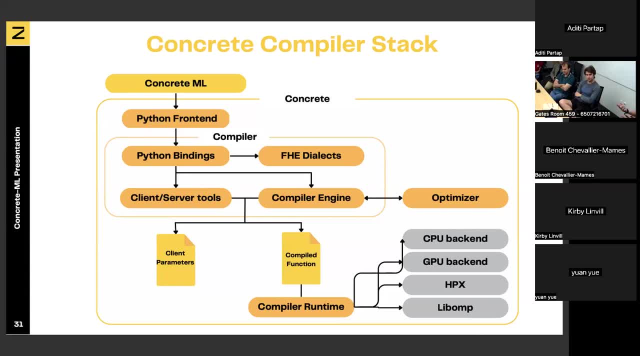 I mean execution, time, cost. they take the best choices, So that's the compiler. But as a human, you don't want to speak to the compiler, So you have a front end. We have a single front end, which is a concrete Python. 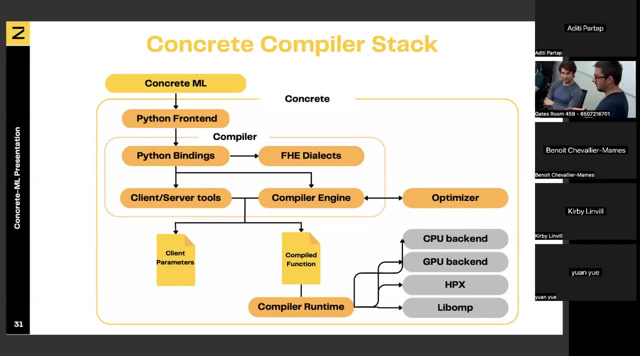 So here you write your Python program And it's compared to FHC. And concrete Python is actually what we are using in Concrete ML. So Concrete ML: we replace your model, We quantize it, We create a function in NumPy. 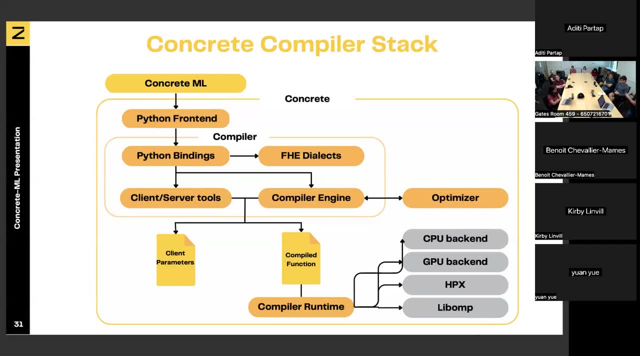 And then we let the artwork done by a concrete Python. So your example is also simply calling functions. Yes, Yes, Yes, Not doing computation between the calls, But presumably I can write an arbitrary Python. Yes, Yes, In Concrete Python you can write: 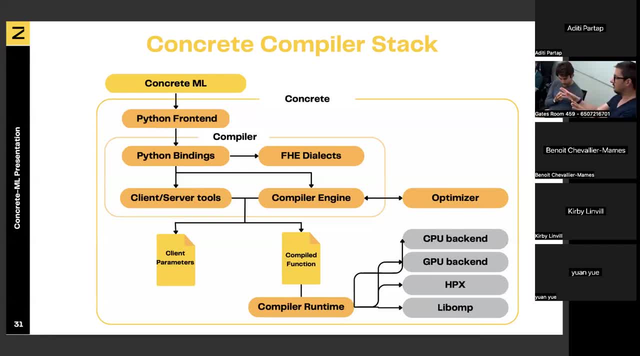 So there are still some limits, So integrals, for example, and univariate functions, things like that. But yes, you could more or less write anything you want. And notably also one thing that we will do at some point at Xamarin is a collaborative. 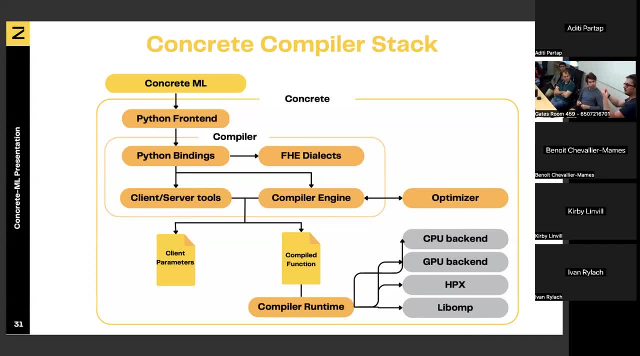 computation where you have a function, which is always some inputs, which comes from different entities that don't want to share the data. So we will write this in Python and compile it to FHC. And one quick question: I don't see a debugger. 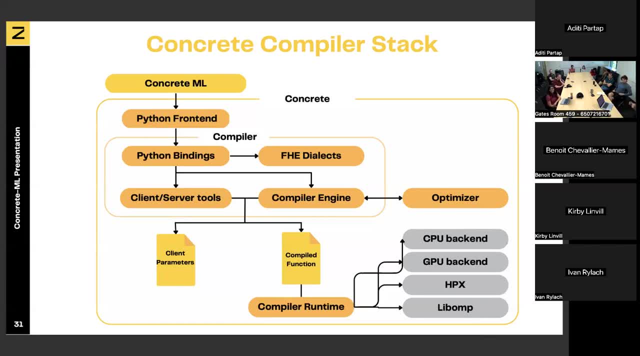 Debug? Yeah, What are you doing for a debugger? Yes, So when you have a bug, it's not that often, But so a bug, for example, might be. I don't know if it is a bug. If you take too many, you are too optimistic. 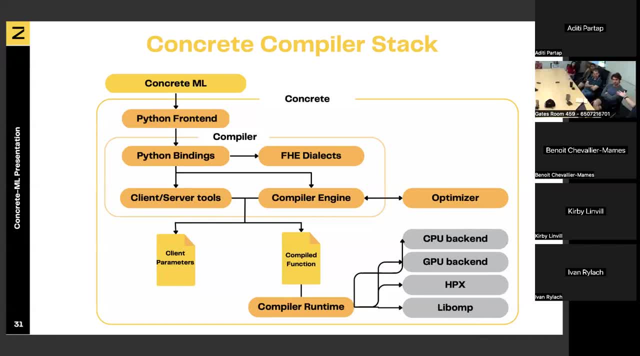 you take too many bits and then at the end of the model it takes too many- I mean it says it is going to break- and tell you: this step has 23 bits, which is more than 16 bits. Do something. 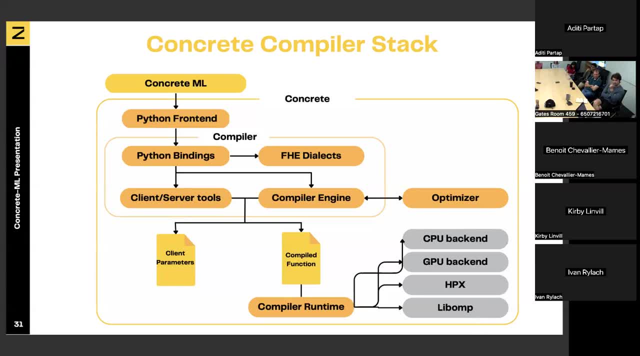 Yeah, no. no, My bug is normally I put plus when I should put minus. Yeah, but I mean you have to read your stuff. No, I use a debugger to find this. to do a single step: look at values. 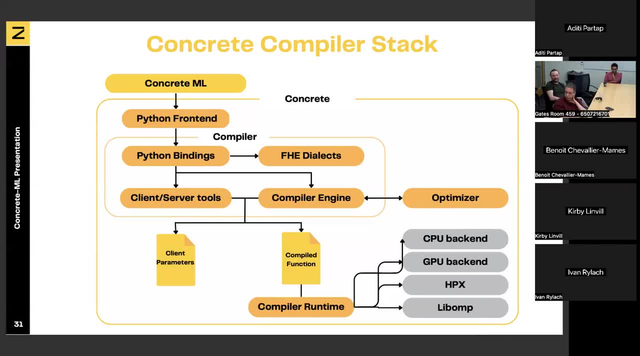 So there is simulation which may help you. OK, I've noticed that You certainly don't want to debug things in FHC. No, The simulation is normally very equivalent, So it does the same computation, but over without the FHC. 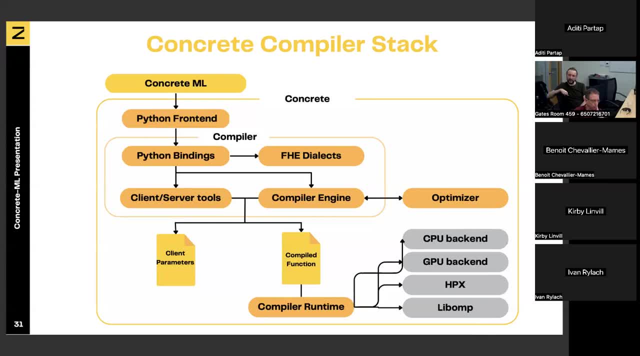 So debugging that? Yes, But you mean debugging the output of the computation. No, I mean just debugging the compiler. Oh, but then you debug it as you debug a Python. Yes, So you write your Python, you make it work, so it's your work. 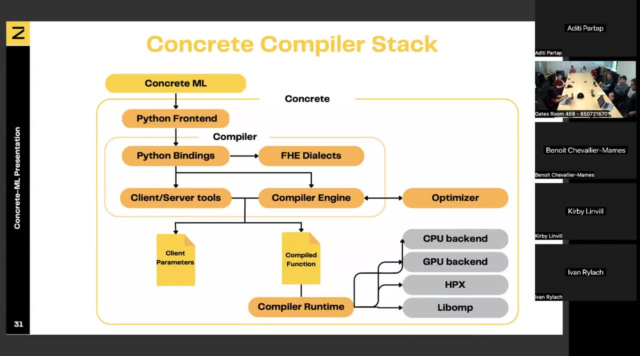 and then you can turn it into FHC. OK, got it. Yes, That was it. Yeah, But how do you deal with the compiler? Debugging the compiler is an adventure. No, you don't. If we really wanted to do things well. 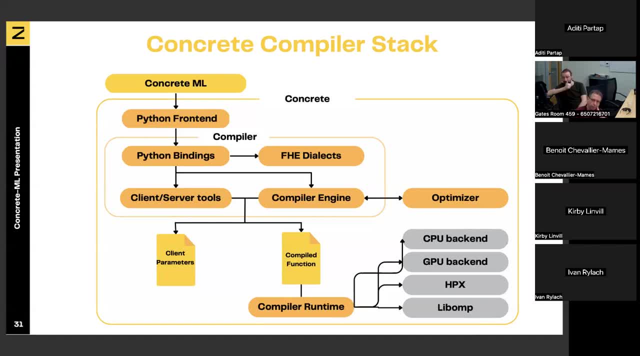 we would turn to formal methods and try to improve the compiler Correct. So what you do is you have a bug in something in some products that we have compiled. You just go to our support. So we have a support. We have a forum where you can ask your questions, like Stack Overflow. 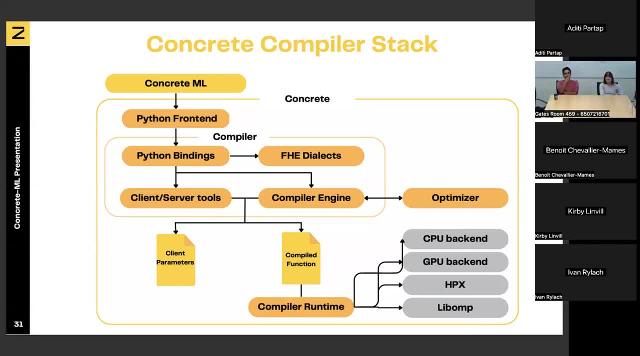 We also have a Discord where you can ask your questions but also discuss with other people who are working with FHC. So yeah, you ask and we're going to help you for free Then. so at the end of the compiler, so it creates the client parameters. 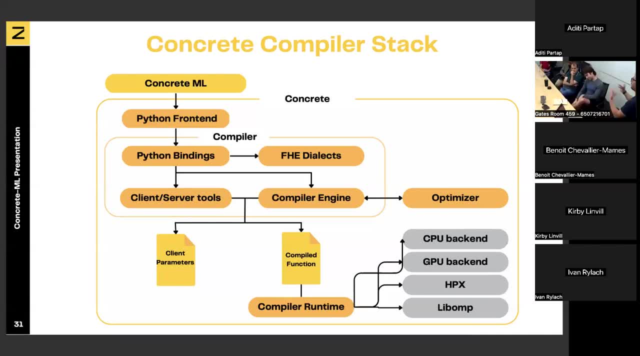 which contains in the database the crypto parameters. So if you have a crypto browser and you want to check what Zama is, It tends to be secure. Yes, you can. You just have to look there, You check with the latest estimator and then it looks fine. 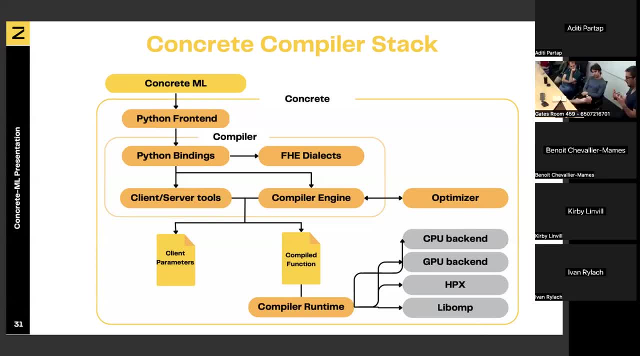 And then the compile function at runtime is going to use the backend. So for now we are mainly about CPU backend, which explains a bit why we are sometimes slow. But we are also working with either internally in the company or also outside with some big companies to have hardware accelerators. 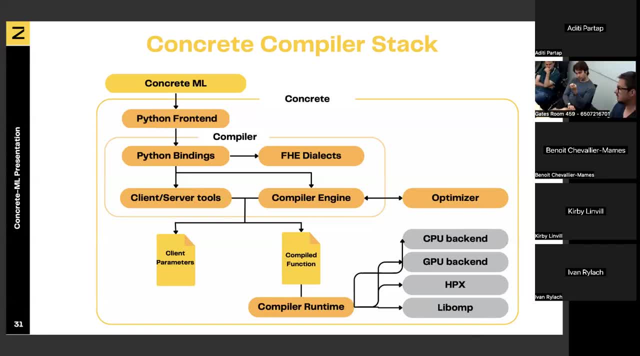 So GPU is something which is going to come very soon, Then FPGA, so it's a bit longer, And then ASICs, So we will have a lot of improvement speed up by this, but it takes years to have it And it's not done internally. 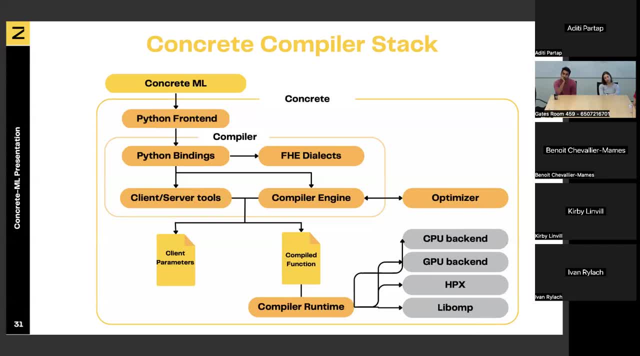 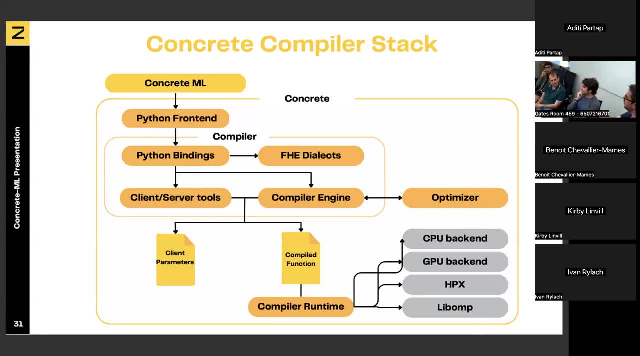 so Pascal said that every year we multiply the performance by four. Every couple of years there is like a 4x improvement. But what we need right now with hardware acceleration it's closer to three to four orders of magnitude And KUL. so people in Leuven are actually 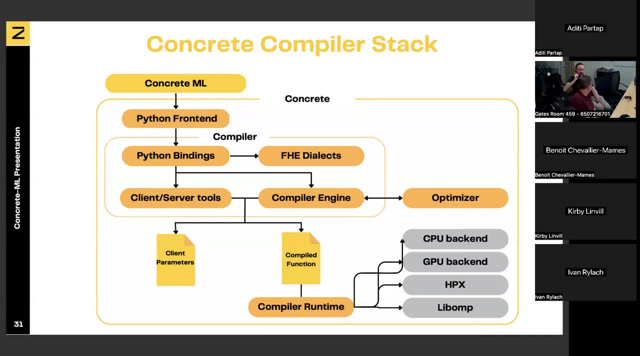 working in a great group, a very well-oiled group, that are actually building. I mean, there are several teams and several projects prodded with that kind of stuff. There's like a project with Intel, with other people building some hardware. 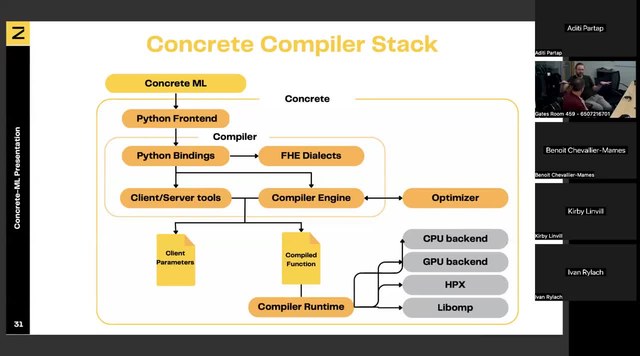 But right now there are like six, seven different groups of people that are actually building hardware acceleration for FHE And KUL. so they in Japan. so about when was it? Weeks? Weeks, Yes, They were there, right. 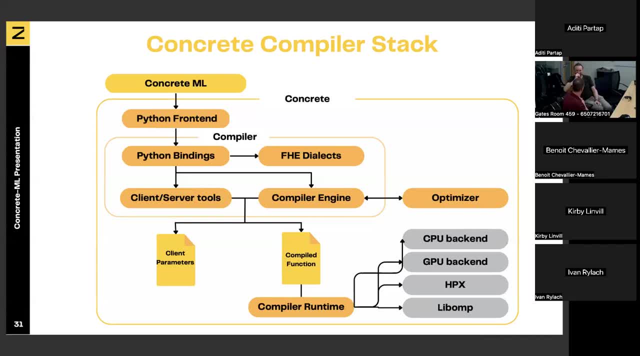 I think I remember, And so the guy from Leuven, he actually did the presentation. It was awesome. Yes, And they have like a factor, a speed of 4,000.. And they're very- In FPGA. They hope with an FPGA which means the day you go to the. 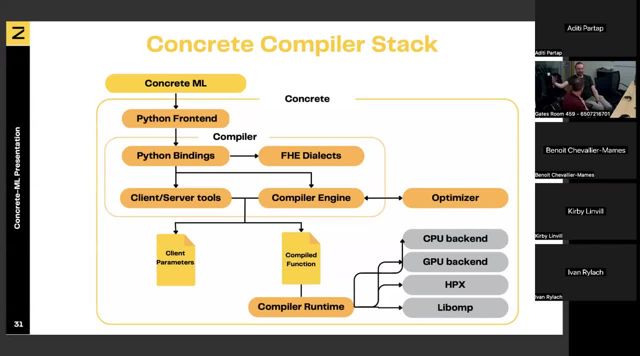 all the way to the exec. it's even better because you have less power and you benefit from really doing like a lane. Yeah, It's amazing, But it's so. it means that we're very close. We predict, like by 2025, actually, there's some snags of it. 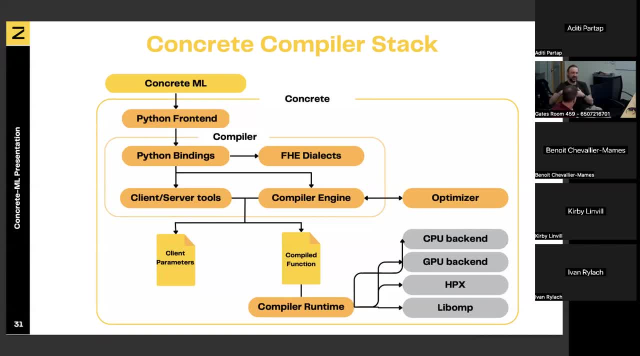 It will happen sooner- 2024, by next year- that actually we have hardware acceleration And then it means you can have like a homomorphic equivalent of what you do And the worst that you would use is like the factor between the 1x and 10x, which means the crypto. 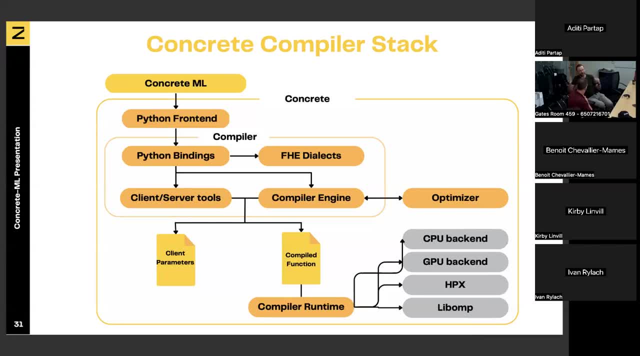 but with hardware acceleration compared to non-accelerated- Yeah Yeah, Non-accelerated non-text operations, But it means that the crypto is not a bottleneck anymore. If it cheats, at one point it could become faster. 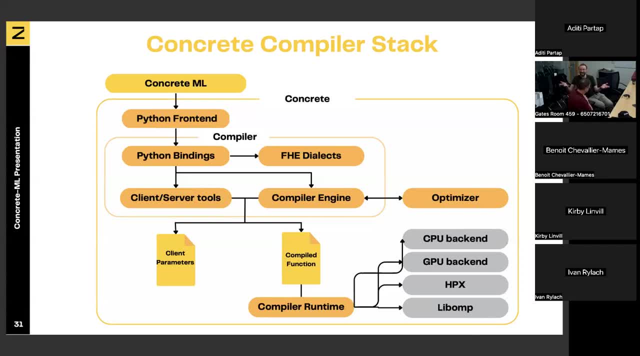 Yeah, Yeah, Yeah. In some cases actually Yes, Yeah, Yeah, Which is amazing, And there's a cap, And there's a cap, But it means that at some point there is no point not doing things encrypted by default, because it doesn't change. 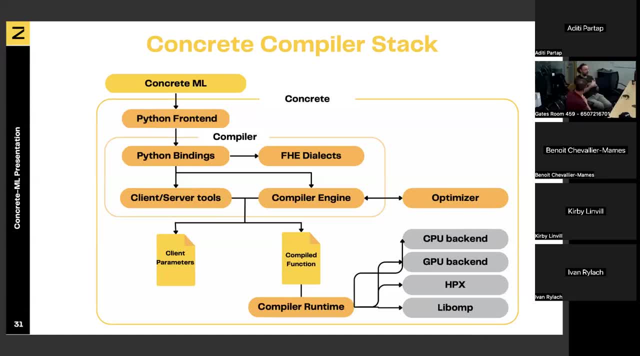 the user experience And actually you will have to explain why you actually you care, You are the data handle here Which will become suspicious. So we're coming very fast to that very exciting moment in time where everything will be fast enough. 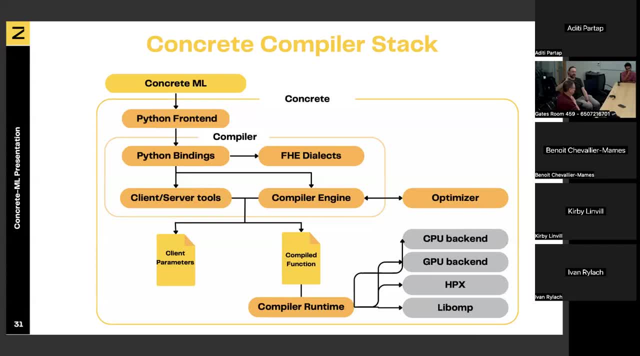 to become a homomorphic execution to support, like 80% of AI applications, cloud applications, whatever applications, Which is nice. Well, smart contracts have shown that people will put up with the one that they're in the package. Yes, Yeah. 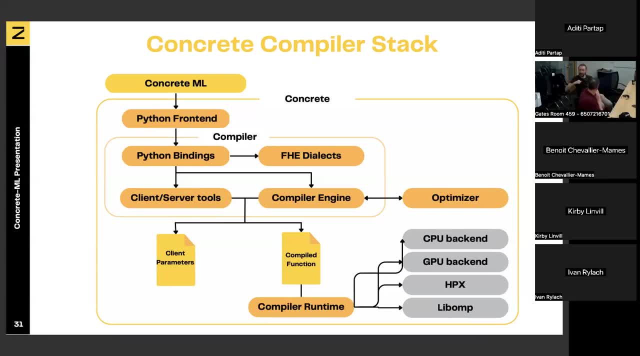 Yeah, Absolutely So. that's why we're also working on blockchains and things, Because we think right now people are not afraid of integrating advanced crypto stuff. They actually very often read the papers on their own And overnight you pop something in some GitHub. 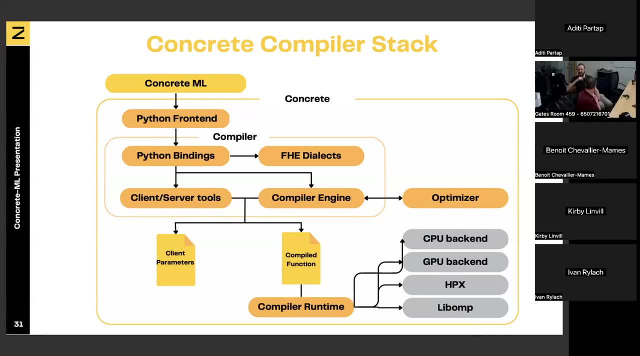 like every day or something. So they're not afraid of adopting super advanced, almost still like stuff that is still being researched, And there's a huge appetite for the blockchain for everything that has to do with encrypted applications, But that sensitivity to new stuff. 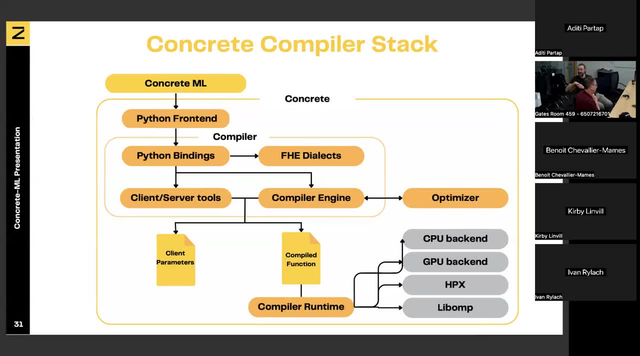 depends on the value of the smart contract. Yeah, exactly, They're very conservative for the big ones. So this year we are actually launching a test next where you will be able. So what we did is we took the Ethereum virtual machine. 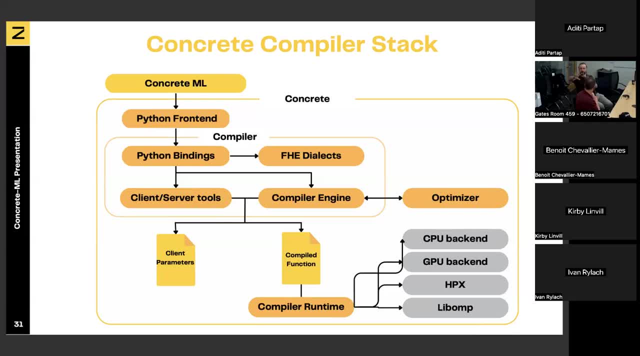 We made a FHE version of it, And so nothing to do with the distribution. by the way, This is really ML-oriented, But we have another team working on this where we're exposing solidity, like constructs that are very easy to use, where you can annotate. 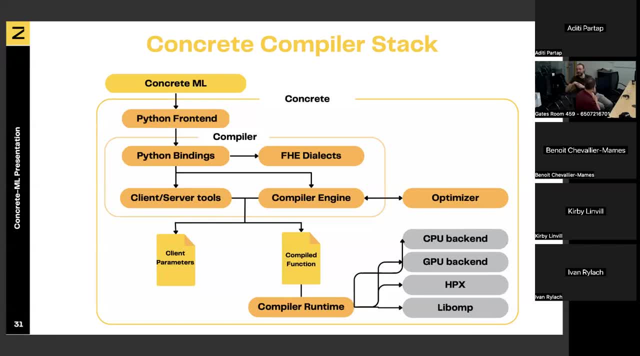 You have basically a type of notation where, for the developer who's developing the smart contract, these and these variables are encrypted And the state of the smart contract, this state machine, can be encrypted as well, And this is where it becomes important to use the encryption. 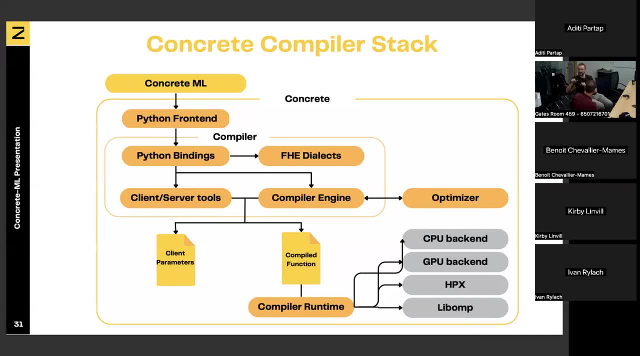 technique that we're using Because we have super-fast bootstrapping. One bootstrapping is like a few milliseconds, compared to the other crypto solutions where bootstrapping takes like 10 seconds or something. Well, it always depends on parameters. 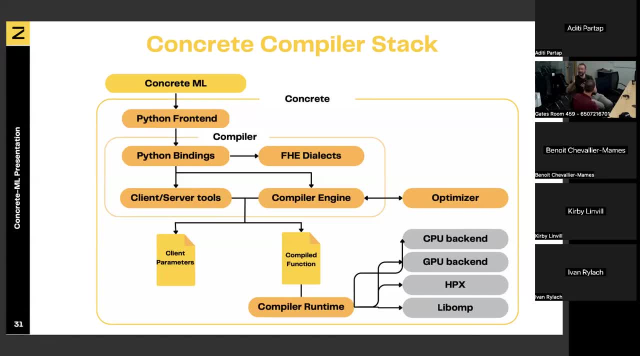 And so it means you can actually run already homomorphically secure, homomorphically encrypted transactions over Ethereum earlier this year, Unfortunately. so the historical moment happened. Yeah, It's like being it's in the works. Unfortunately, solidity is not a secure programming language. 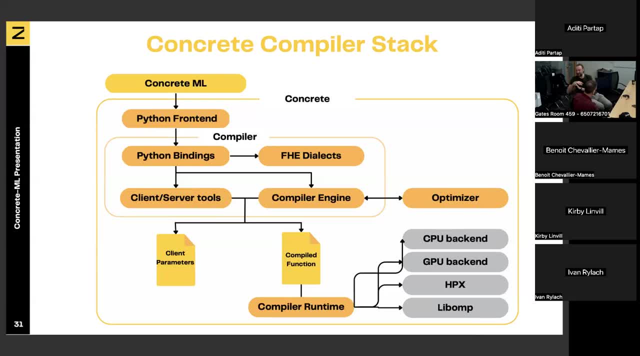 A company Agoric, a company Agoric has one, So you might want to look at them. Agoric, Agoric, Agoric, Oh, Agoric. OK, They have a secure, interesting language on top Any different topic. 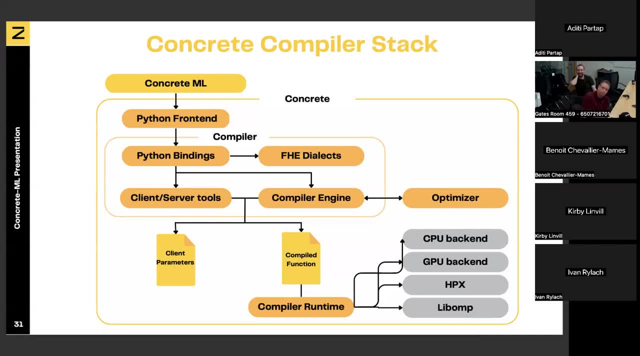 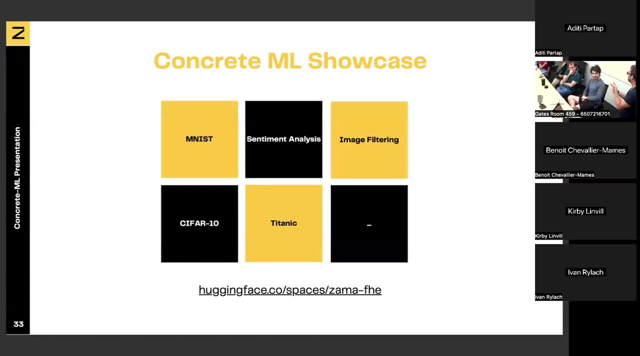 OK, back to you, Yeah, back, Yes. So, yes, if you want to try this, I recommend you to have a look to, and just have a look to, what we were able to do, And maybe you can do better. So there are the demos that we have put in the heading phase. 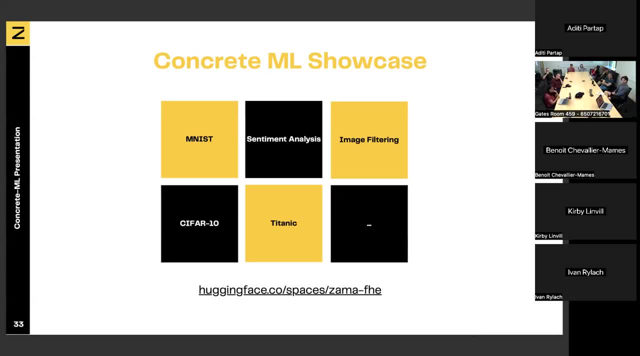 so image filtering and sentiment analysis, where we take a short message which is encrypted and tell you if it's a positive or negative message. Yes, OK, Thank you. Yes, So obviously we have a missed classification. So here it's done with the easy neural networks. 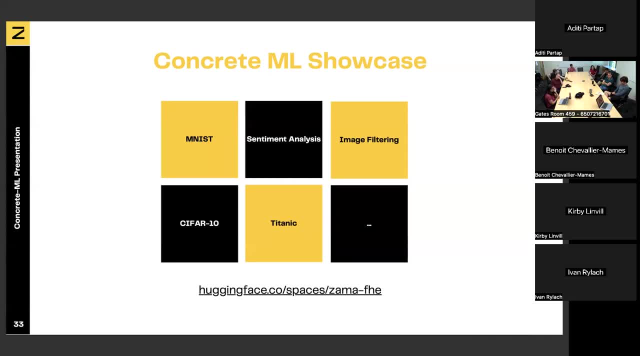 so the beating neural network that we have in ConcreteMEM, So there is just a few parameters to set. We have also a version of Titanic. So here it's only some three days. I don't know if it is random for us or you can see. 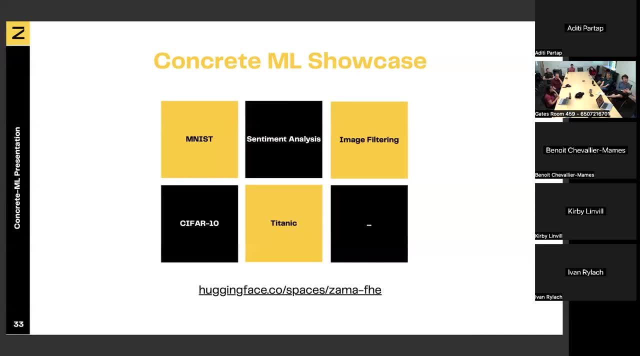 And for the most advanced examples that we have, and so we have some examples We cipher, So classifying some objects. So here it's done with a complicated deep learning stuff that Jordan explained, So with a quantization-aware training So you can see how it works and does a good 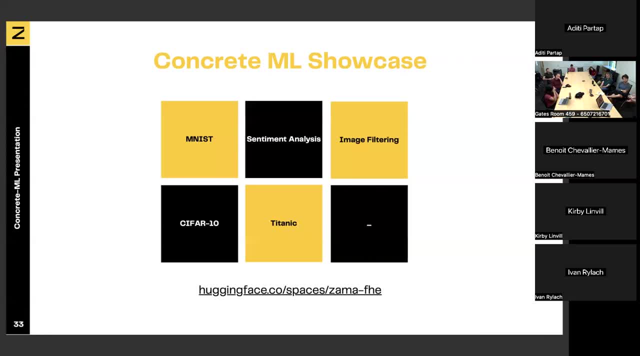 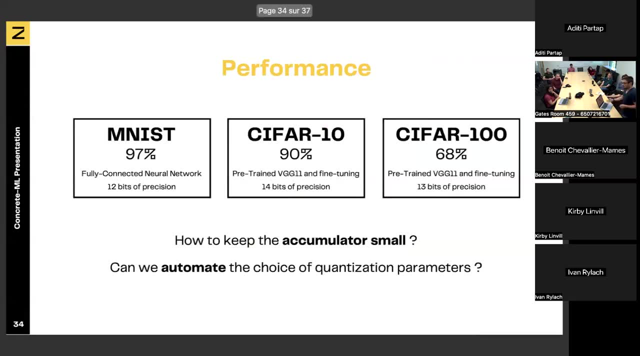 But the team was able to have very good results for cipher, but making it as small as possible. So at the end we have results like that, OK. So yeah, 97% from this, which is not state-of-the-art. 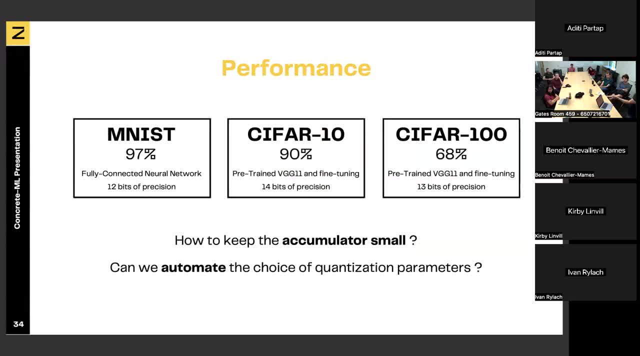 but it's quite good in FHE. So at the end you have 12 bits of precision for the integers. Then we have cipher 10, and 100, where the accuracy is also quite good. So more or less it's equivalent to VGG, a kind of model. 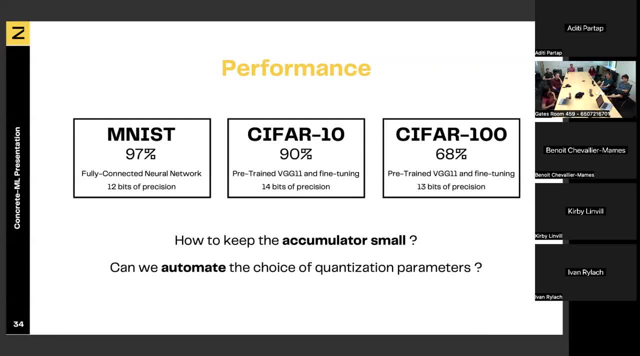 which was state-of-the-art not a long time ago. So here it's like 13 or 14 bits of precision, OK, OK, So today with what is publicly available, so it's hours of computation, just for a single inference. 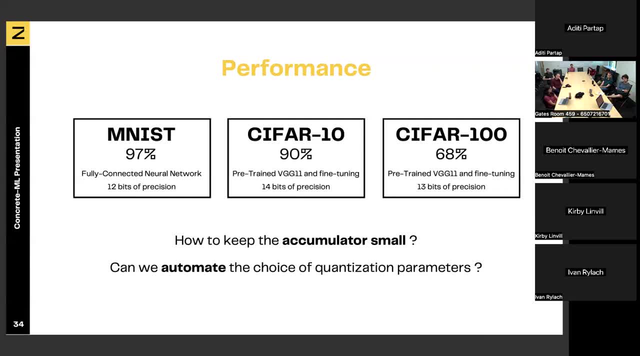 But there is something backing in the team which we are going to release which will make things much faster. More or less, when we have a big accumulator, we just take the few first bits of this And so we approximate, We move the bits of TM, which allows us to, instead of having 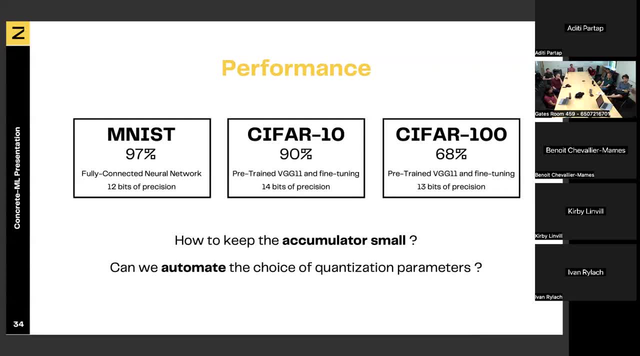 PDS of 13 bits, we can maybe have PDS of 6 bits. So obviously you are going to have the computation which are related to the speed of a 6-bit PDS. So with that, how long do you usually have it run? 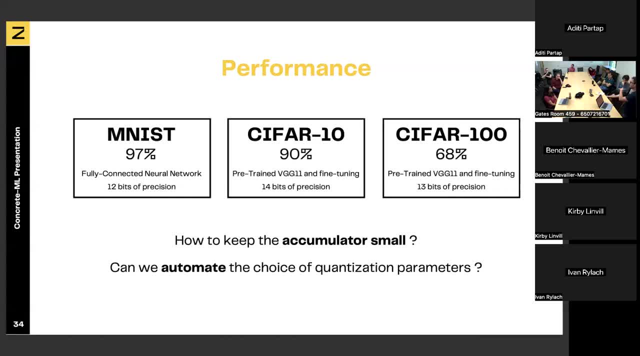 So it will be. so far it's a cipher 10.. So our estimation- because we haven't been able to run it- is that it's going to be like 22 times faster, which translates to about what? So it's 20-something minutes. 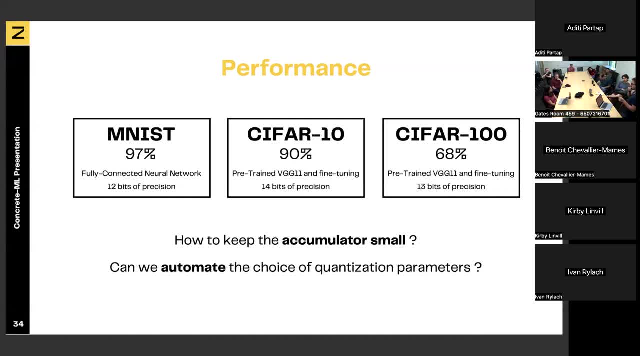 OK, OK, OK, OK. That's the inference here, which is still not very practical. So we are still waiting for the unread. Yes, Yeah, perfect. Everything will come into place without our inspiration, essentially because in machine learning, 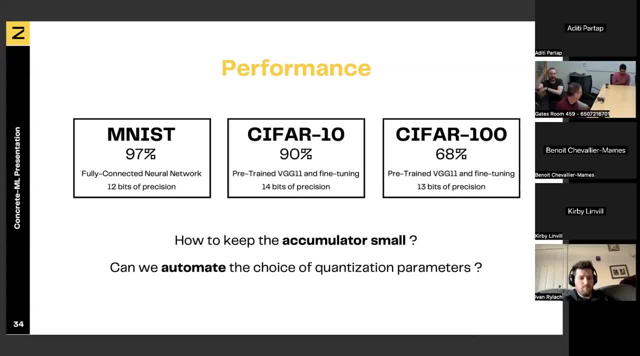 you can do all these layers. You have infinite biases And it takes just a few milliseconds with one bootstrapping You could do, and because you're bootstrapping, so the cipher types are clean, are always clean, so you can go as deep as you want. yeah, and it only depends on the number of layers. 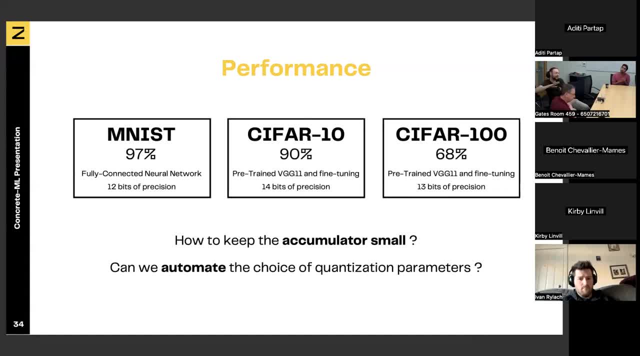 not the number of neurons with infinite value, which is which never happens. so actually, at the end in the company, we are trying to improve the speed by at a different level. so my team is using less bits of quantization. a compiler is making things more efficient and then we will have to have that submission which are going to make this? 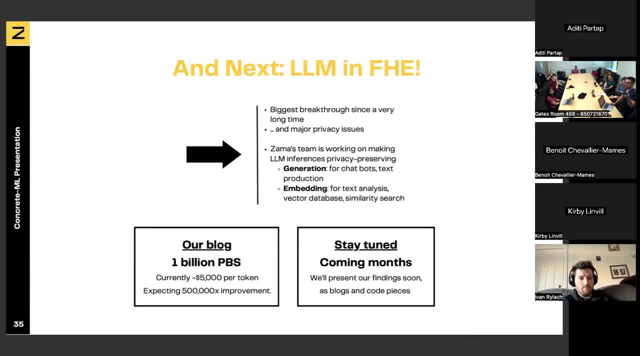 pretty fast. um, obviously, so we have to speak about them. so what when we say about lm and fhe? so you've read the news. uh, if you were asking a change, so it's very bad for your privacy. so we plan to work on this in zama. 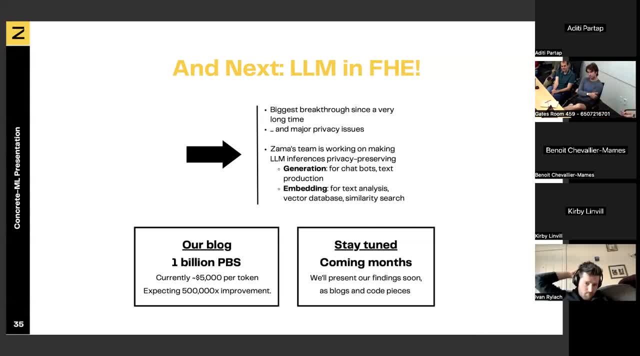 so we just made some estimations. so that would be like 1 billion of pbs for an lm, which is a lot, um, so we have given some numbers. so it's a 5 000 dollars per token, which is a lot, and so we expect we we need to have things much faster, but still we will work on it this quarter. 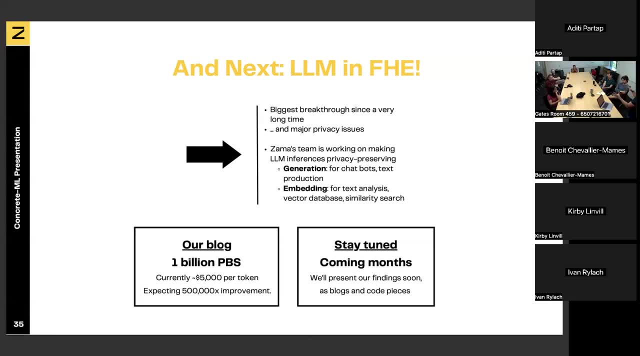 in the team and and so we will work on it at toy scale. so we'll just show you that it's possible to do it. uh, more or less, and just uh. then we will say we wait for the hardware accelerators, and just for the fun of it, yeah, and how much memory do these things? 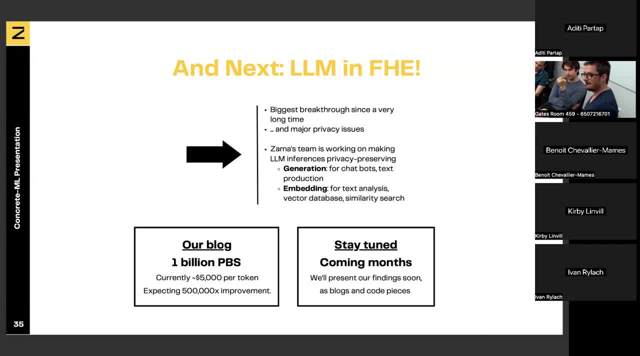 well, um, i don't know for the real ones, uh, because we don't even know what. not the lms, but the previous ones, yeah. so, for example, the, the biggest thing that we would go, it took like 11 gigabytes of ram. okay to, uh, it's, it's about one, oh yeah, oh, i mean what we say. we really run around them. so, yes, it works. 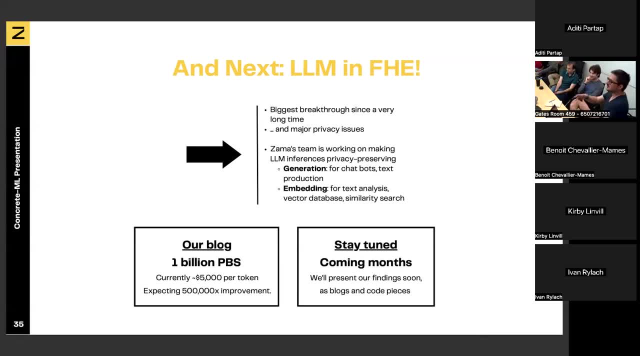 um, yeah, i don't know it works on your phone, but it's not supposed to work on your phone. that's the next model. and also, yes, one thing. so the team has many work on the accuracy to make things as good as they are in the with fruits. uh, then we will work on speed. so i told you that we. 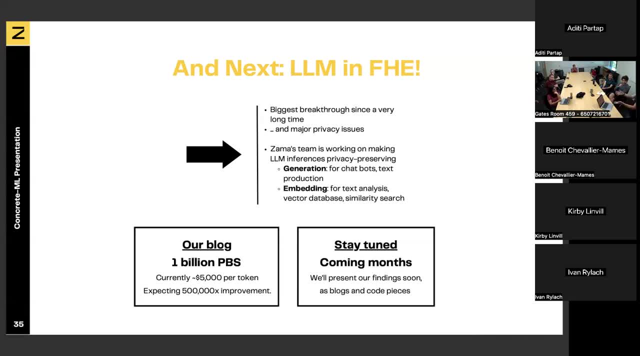 will be 25 times faster. then we will work on making things more efficient, like smaller keys, less RAM and things like that. So we know some techniques, how to compress ciphertext or the RAM and so on. It's just that we have to focus on something. 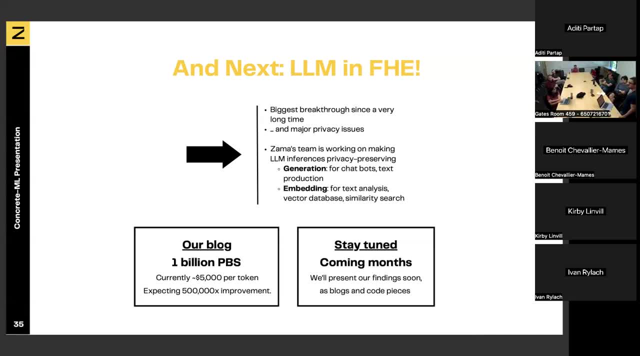 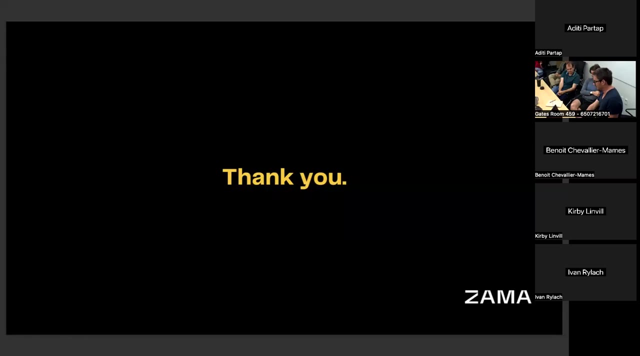 If you are interested in reading Rand, he wrote a blog about the LME FH And we will tell you what. So in three months, as you will follow the company, you will see what we have been able to do. So thanks a lot for your time. So I hope you enjoyed this and you learned a few things. 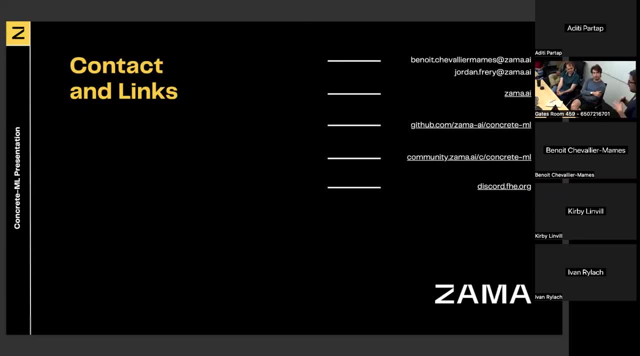 So what would be crazy for me, great for us, is that you download this and you try it by yourself, So you can try to reproduce the few examples that we have, And then- even better for us, you can try to build your own examples. We said that it's open source. I mean for our research. 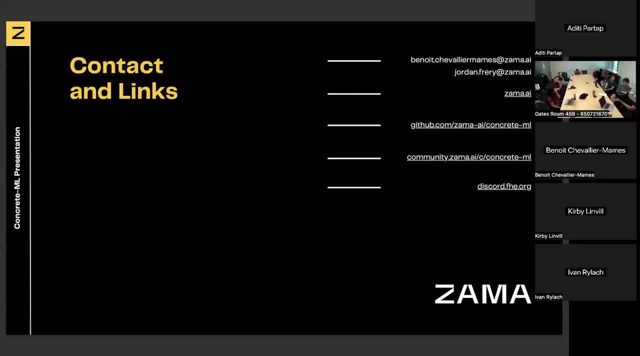 So do whatever you want and show it to the world, And you can go on. you know we said the support channel. So if you are able to make, if you are able to beat us on the cipher, great for you. So tell it to the world and find, I mean, we'll tell you great. 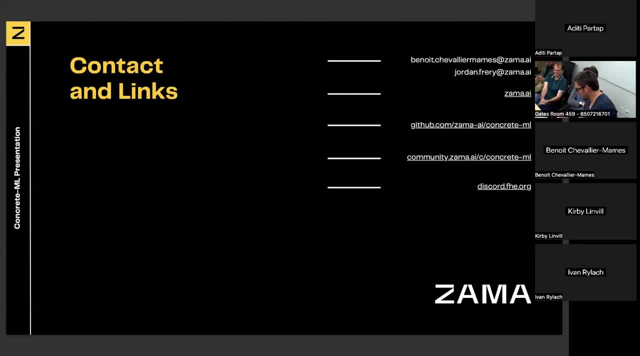 And we extend you another cap. Yes, so that's it for us. I think GitHub, so you can also hit star. I mean just some star over there, And yes, that's it. I don't know if it's a hard question. 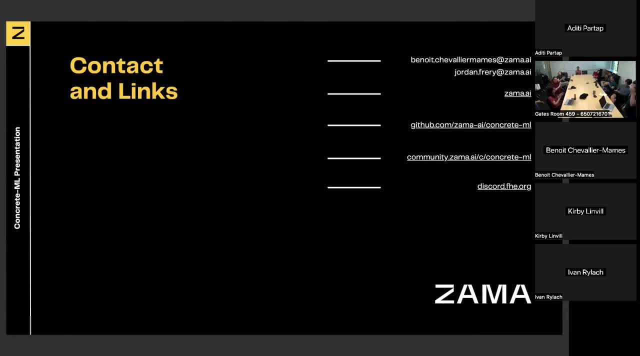 Let's thank the speaker. Yeah, yeah, So there's one question already. So they're saying, like in the home of a domain, can we have an argmax function? This is from Isaac Yan. argmax, yes, it is available with the matrix things, So it's a bit like you know. for the 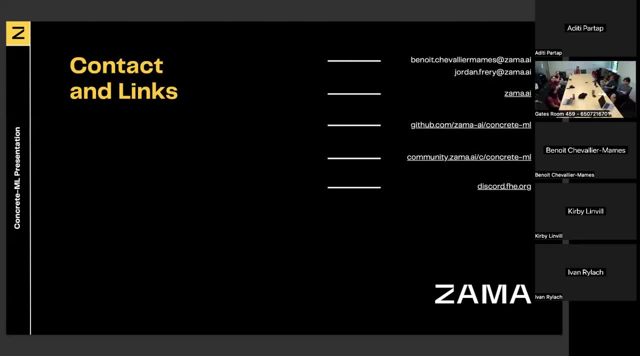 trees. So more or less you compute the max And then with the matrix, we're going to compare where the max is. It's going to be low, not as efficient as it is in the matrix. but yes, I think there are several approaches to actually compute an argmax homomorphically. 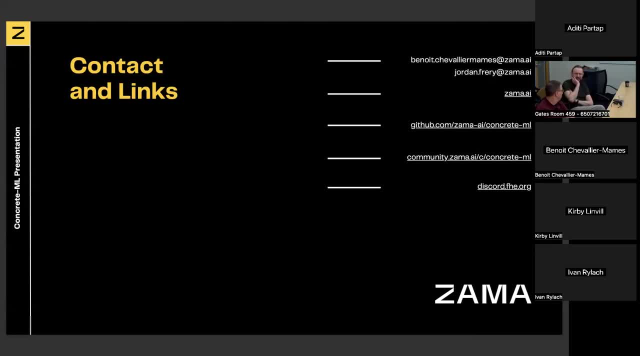 But fortunately there is one that we're, to my knowledge, we're not using right now. Are we Not in computer man? maybe in Python? It's? when we are asked that kind of things by the users, we tell them how to do it. 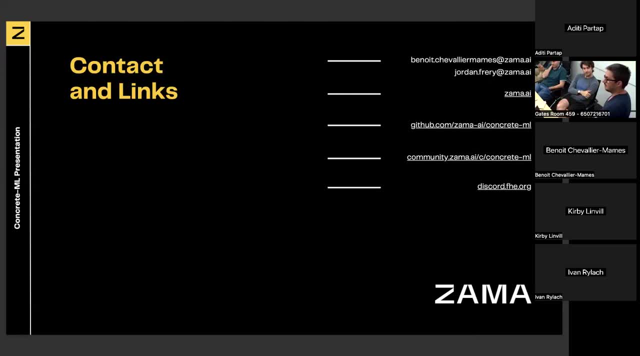 But I wouldn't say it's baked in the product for now. Yeah, I'm trying for the math library for blockchain to require this at some point, but so it's in the works. But every, I mean for all the schemes like CKKS. 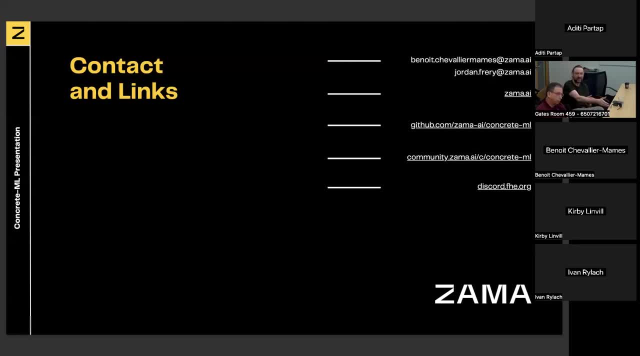 I think there are like a specific solution that works well for CKKS. So, but yeah, The answer is yes, you can do that. Was there a question from the audience? No, Yes, Yes, Yes, Yes, Yes, Yes. 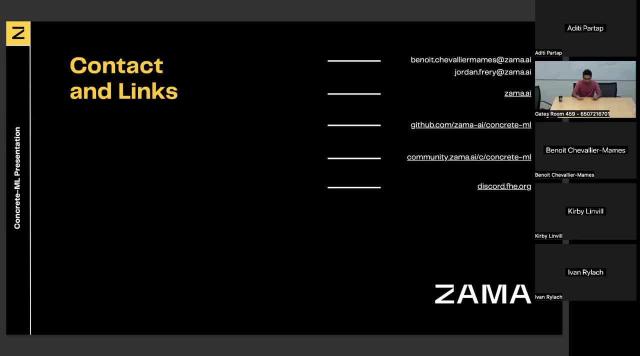 Just thinking through the hardware example you mentioned about acceleration. I kind of wanted to just so that conceptually we're at like one millisecond for PBS. let's say like in an optimistic scenario it's like one millisecond for every bootstrapping. 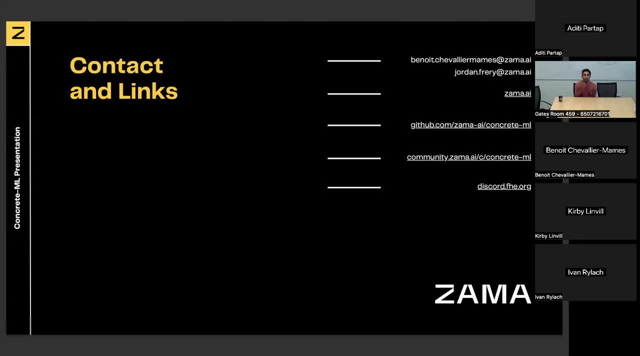 operation Is the way you would think about acceleration, that like eventually we get to, I guess, two 1000x kind of increases where a single PBS is like a nanosecond, like a cycle on the CPU And then it seems reasonable to say that you could. you could be only two X worse than like a plain. 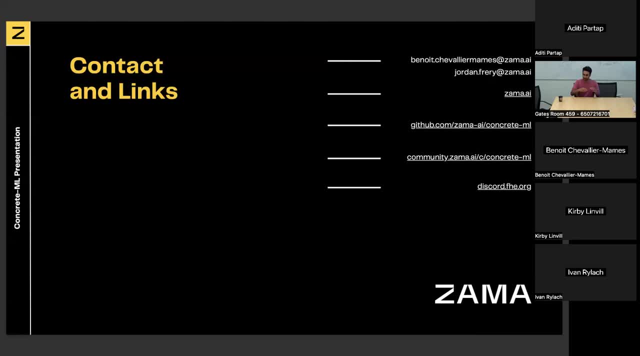 tech CPU because, like each operation you're doing you, you do the normal context operation and then you have to do it with PBS. But I guess what I'm trying to ask is like getting to, within you know, one to 10 X of one point tech speed Once you just on the chip that you're making. 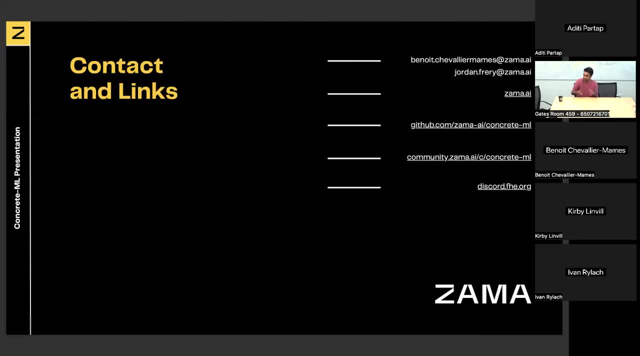 you have to dedicate a lot of diaries to doing the PBS, because those are expensive, right Like each each PBS do you have to do after Each flop. And so then, like, how are you going to get to a one to 10 X? 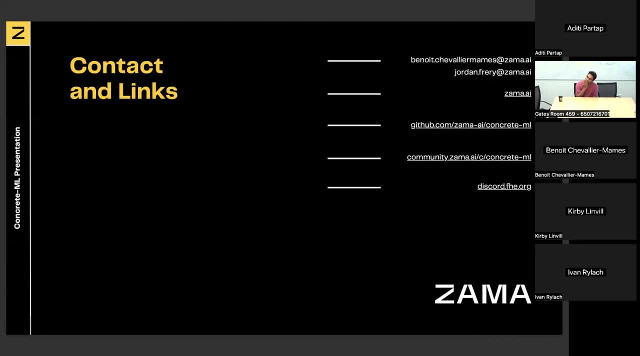 So so there are potential things to unpack. So the first thing is: so it's not like one millisecond but it's closer to like six milliseconds on a CPU or whatever. But just as an order of you know to have an idea of what costs a TV, a TV would be. 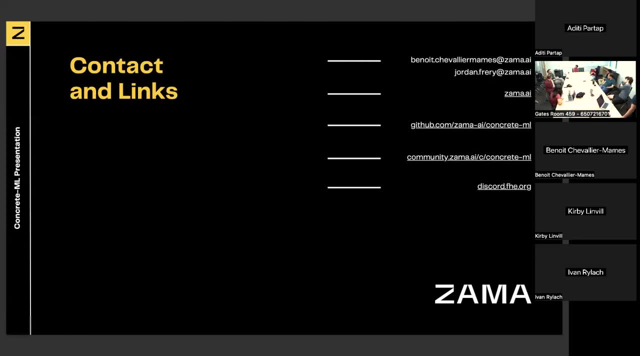 of course it depends on the parameters and everything, and the parameters to the particular circuit that you're evaluating more quickly, and the compiler It's actually finding the parameters back on the fly, depending on, you know, trying to optimize the whole circuit and their constraints. So it's, it's really bad, but like. 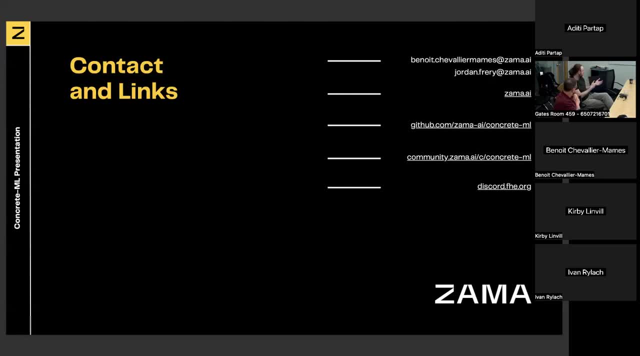 if you have like to remember one, one figure, it would be like this six millisecond or one billion, or just like one boolean gate, like the most elementary or more proportionate When it comes to the hardware. So we have a few people internally who actually work on 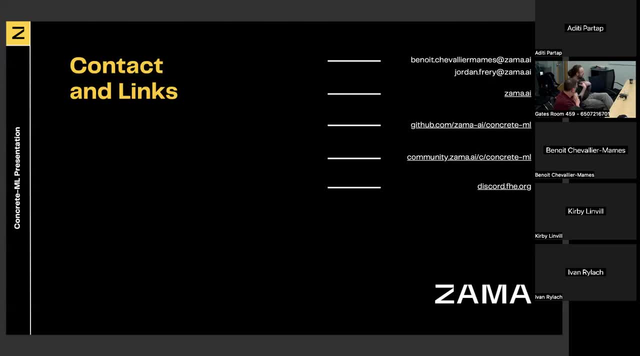 design, But we're not expecting people from their company to to go all the way like where is like for just research. So we're partnering with people who have their own. they have different strategies to implement BDs. So there are companies like KONAMI and Aptobyces, so they all have. 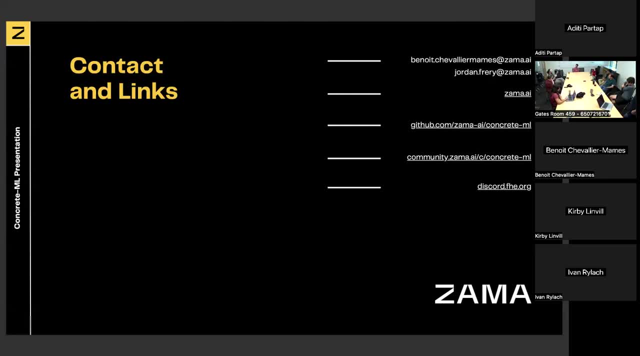 their own angle of this And they're trying different things. Apt besten to have this write issues essentially the bootstrapping operations you need. For that, you need to implement either an NTT or an FFT. Yeah, it's mostly NTTs right now. right, It's like 80% NTTs. Yeah, At six milliseconds. 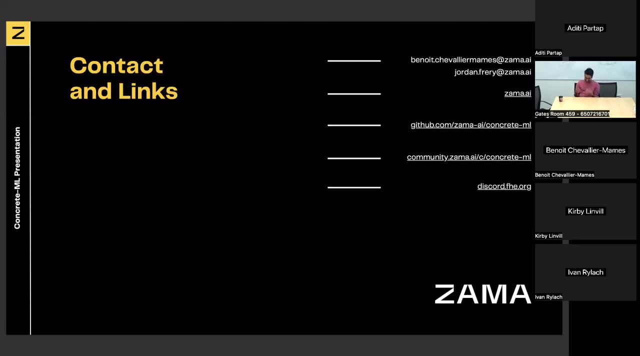 it's like four milliseconds. The bottleneck is doing FFTs And so without NTTs you don't have a choice. You actually have to use NTT. So it's a little bit more cumbersome from a computational point of view, But with the FFT, with TFAT, we can use the FFT. I mean the single heretic FFT. 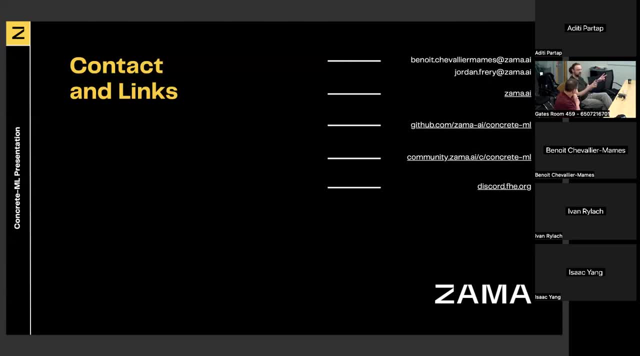 So they can be noisy there, noisy in the sense of approximation errors, It's fine. So you can actually use fixed point numbers and do an FFT with that. And I mean FFTs has been known, in other words, for like 50 years. How big are these FFTs? I'm sorry, How big are these FFTs? 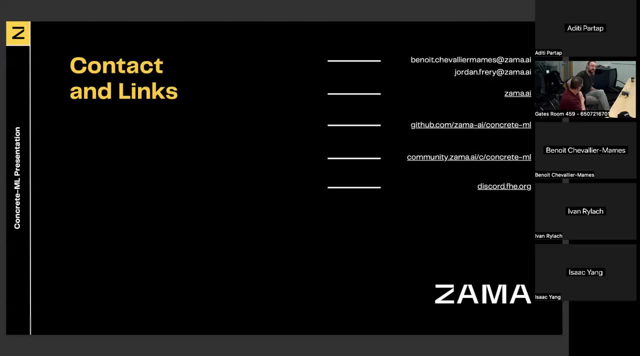 How big. Typically, I would say. the typical size of the input vector is like 1024 coefficients, which is nothing. They're all 1D, They're all 1D. Yes, yes, I think there is an extension of the PDS where you can do things that are 2D, But yeah. 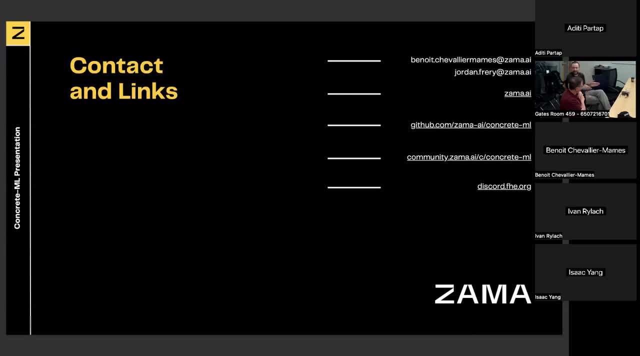 essentially for at least this first wave of hardware accelerators 1D is like, yeah, we don't need all of that. And so, yeah, Yeah, Yeah, Yeah, Yeah, Yeah, Yeah. And so that's why we're so optimistic about the mass adaptions, because the only 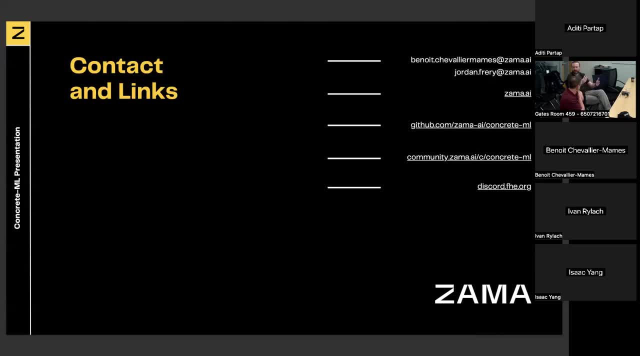 thing that is missing right now. we don't have to improve things at the critical level anymore. Things at the engineering level, yes, Like providing better compilation, being able to synthesize circuits to guarantee optimal topological transformations from the plaintext algorithm coming from the user to the actual circuit. But what do you? 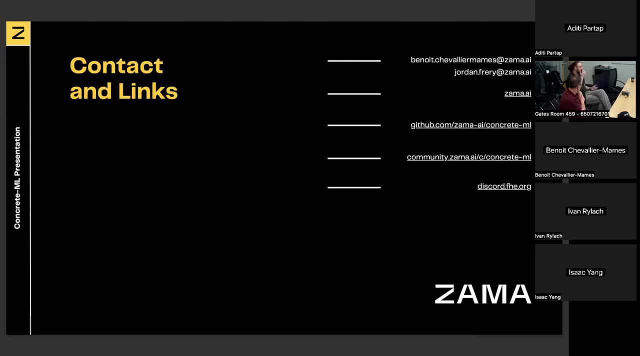 see behind the scenes And possibly best with FFTs. I think that's an interesting question, Or a lot of people are doing it from a different perspective. I think it's clear. I think it's gonna be an interesting question for FFTs because, when it comes to the acceleration, 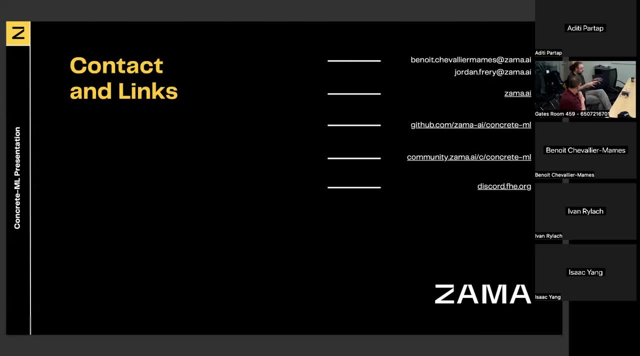 we see that. yeah, I mean, at some point, if you could just like put a lot of FFTs- you know FFT modules- in there and just boost everything. And this is typically what is happening right now. Yeah, Yeah. 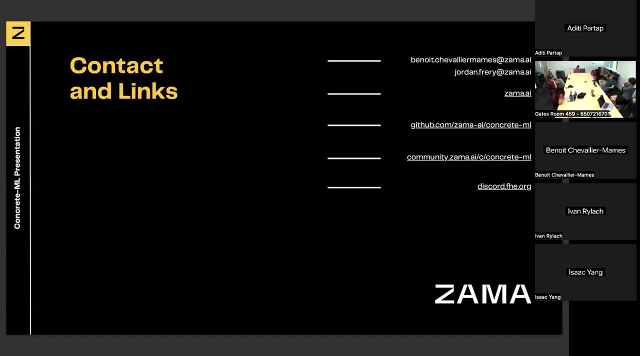 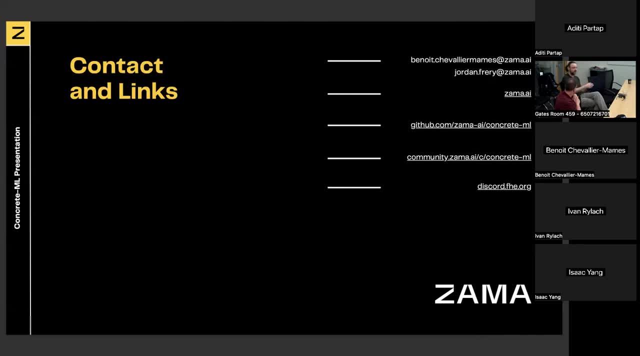 and then go back to the standard domain, do some kind of truncation or whatever, which we don't know how to do in the domain, and then go back. So you spend your entire time in the PBS just switching back and forth between the standard 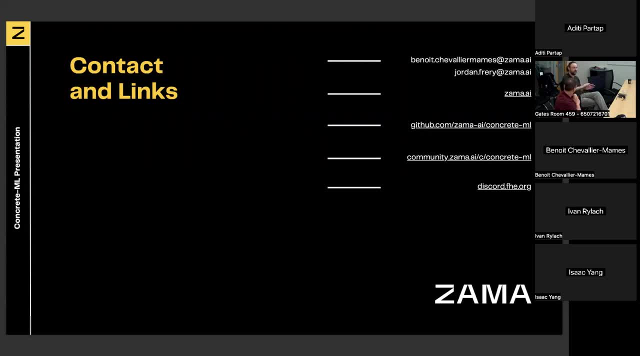 domain and the key domain. And, by the way, if we had a solution to everything, that would be fantastic, because hardware acceleration would be needed by putting out of this world. But in the meantime we don't know how to solve that kind of problem. 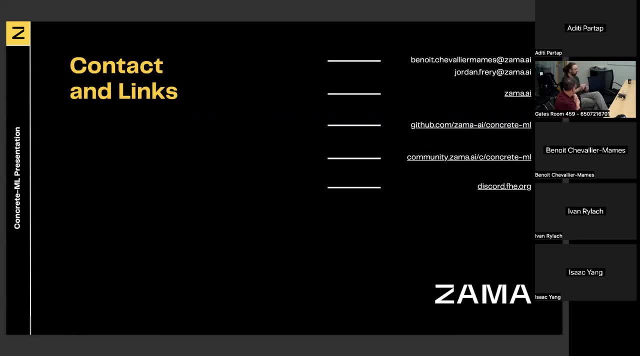 So it's not only about doing the FFT conversions of everything, but you also have a little bit of logic that you need and that you can do quickly. but you need to have like a hybrid thing. And there are other companies, Like Cronomy. they have like a way of I don't know how to describe that. it's kind of a. 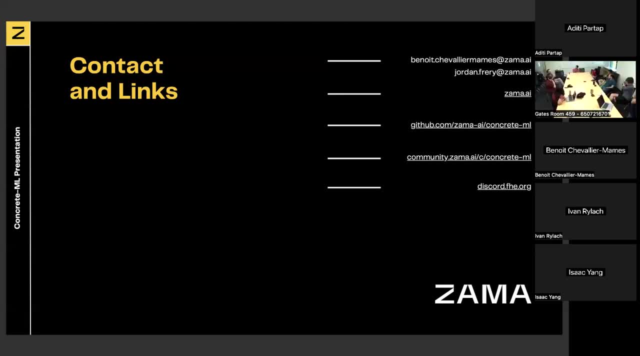 flow computation, where everything is like: what's the name of this? Streaming? Yeah, it's kind of streaming. Yes, exactly, So you can kind of stream, have a stream of computations, like having some kind of an avalanche effect, depending on the availability of what you're computing at some point. 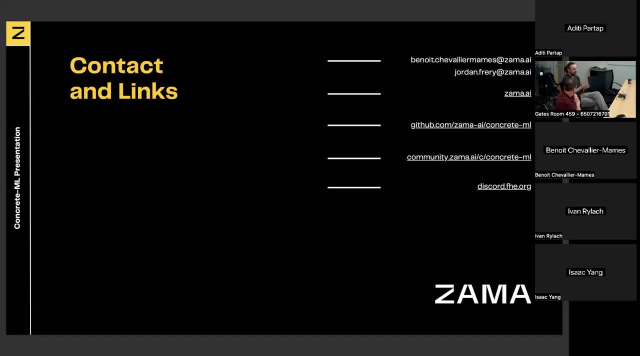 But you can do that, So you can. basically, yeah, they showed that they have like a very interesting- it's not typical to FFT. you can program the other hardware that can accommodate with any kind of computation. But I guess the previous question was: it's really fascinating that you could imagine. 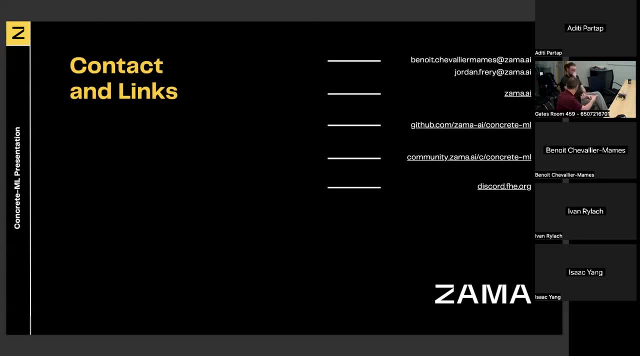 the X86 changing. It's just a PBS instruction. Yeah, you can do something like that. Make a lot of space in the back, Yeah, yeah, So so even there, I don't think that is actually that costly, because when you think 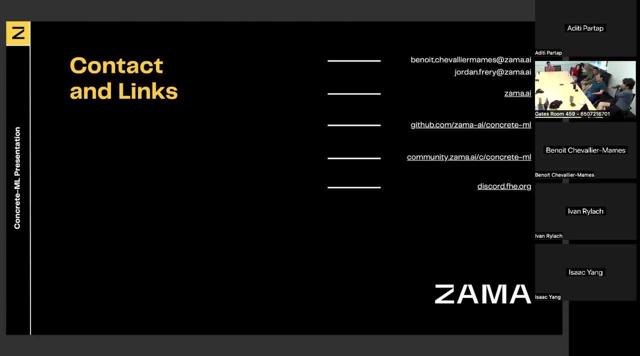 about like where all this big is, some chip goes to not doing it. yeah, it's caches and it's branch prediction and stuff that's like not in scope for what you're doing here. Right, Prediction you could get rid of, because everything we do more. 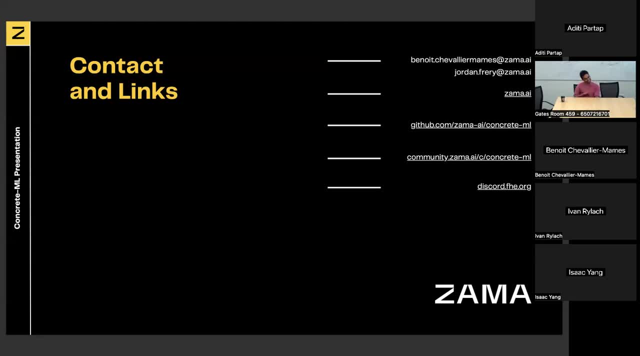 Exactly, I know Before hand. You've paid that price already, You know, And it has to do. You can get rid of that And I think that it's. but yeah, It's actually fascinating to think about this. It's interesting. 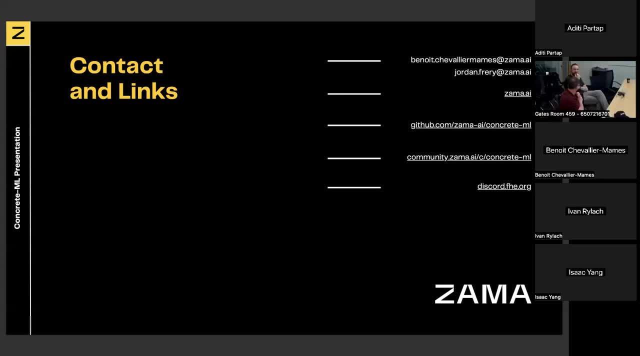 of a homomorphic CPU or a homomorphic filter machine. Nobody's doing that yet, or is that something? So when we created XANA, the big idea was: okay, we're going to create a homomorphic filter machine which is hardware agnostic. We're going to have like a kind of a standard format. 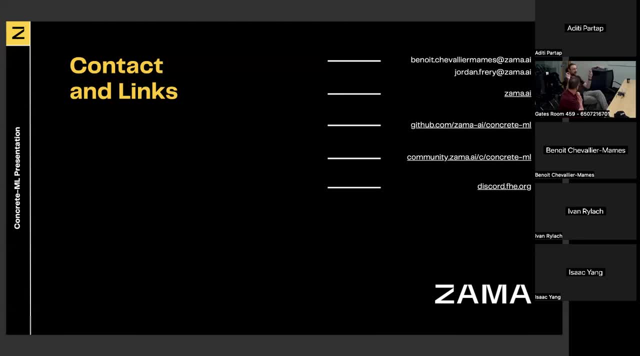 for circuits, like a XANA kind of homomorphic executable format, and then we're going to have this collection of the two machines that are specific to different, like target architectures, Like they will be the default one for CPUs and then maybe one for a single GPU or maybe. 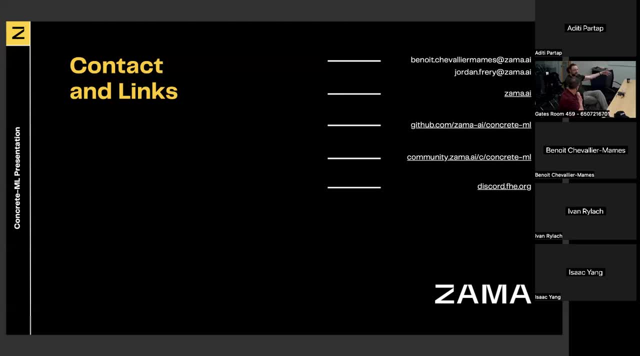 a bunch of GPUs, then the day an ASIC or whatever is available, a specific one every time, But then on top of that we will build a compiler that generates bytecode that can run on any of these machines. It was like our vision, and then we figured that it's not as efficient as 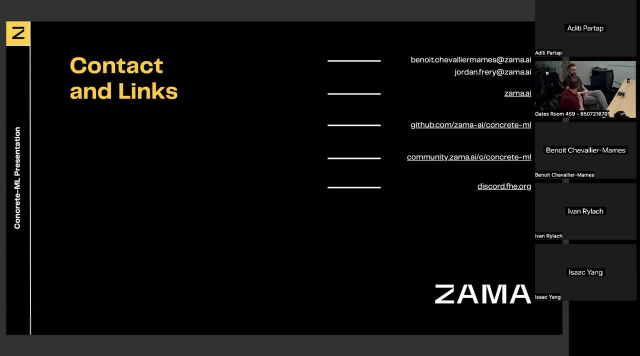 complex. So we started piling all the way: generate code for the target architecture and then just deploy that to push the button and just forget about the virtual machine approach, because so we at the beginning we tried that and it was so there was a lot that- the crypto, I mean. 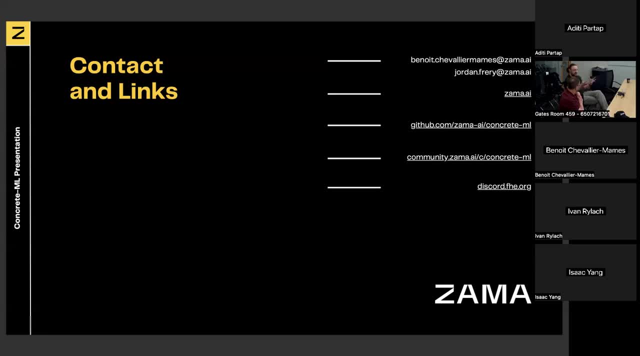 the crypto was what it was in terms of performance and everything on a single CPU, but there was a lot going on with memory management, like things, objects in the cache and stuff that you don't see when you operate on top of a crypto library as a virtual machine, but you lose a lot of time from. that and if you, if you actually compile all the way to the target code, you can integrate orchestration. you know scheduling and stuff you can take and they're already like you can resource to an LVM to do that. there's an entire like ecosystem of gradients and tools that you can. 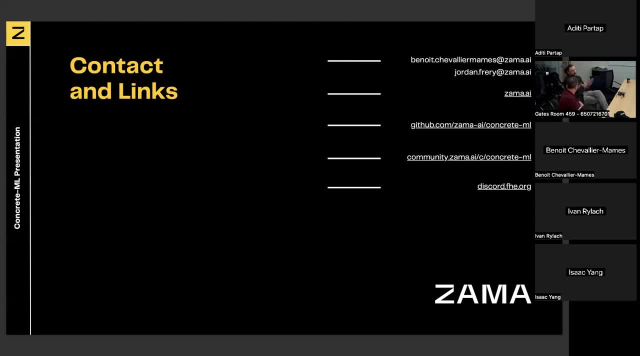 reuse. So that's what our compiler does. it goes back to an LVM after doing all these transformations and actually relies on the back ends. So you have good. you have good looks, good locality. yeah, exactly, exactly. and so because it wasn't, I mean making the crypto as efficient as you can is 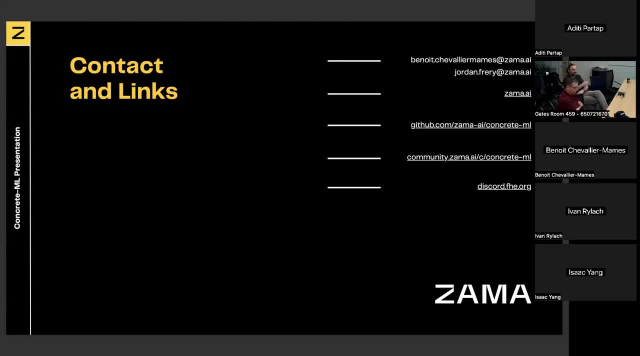 always good, of course, But it's not good enough. you have to take care of so many stuff when you actually deploy it. Yes, and it has nothing to do with the crypto, but you need to have some control over that to optimize stuff, and so it's. it's like. so the virtual machine approach is pretty sexy. because it couldn't make it like easy to work with. you can have an interoperable people who have like a kind of standard format so they could like handcraft programs, like do you know, write down programs like by hand or something, or even their own compiler- all the compilers would. 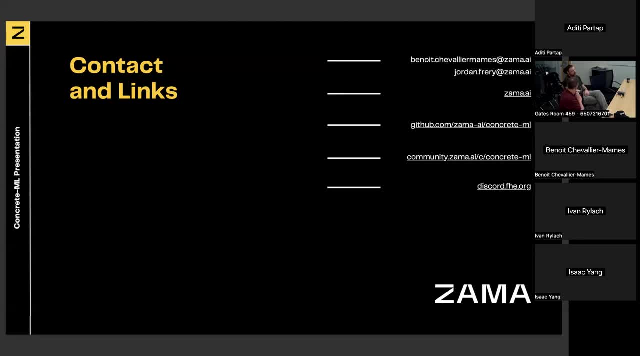 be, you know, interoperable. who are thinking of using WASM as like a universal language to mix both codes, instructions writing like normally with up with up code. homomorphical codes like to extend like and work on encrypted values but have some kind of representation of the memory and 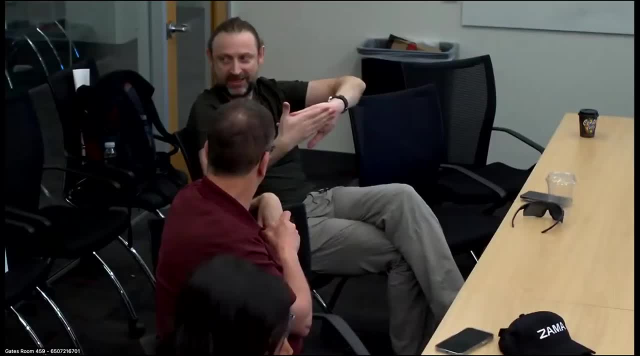 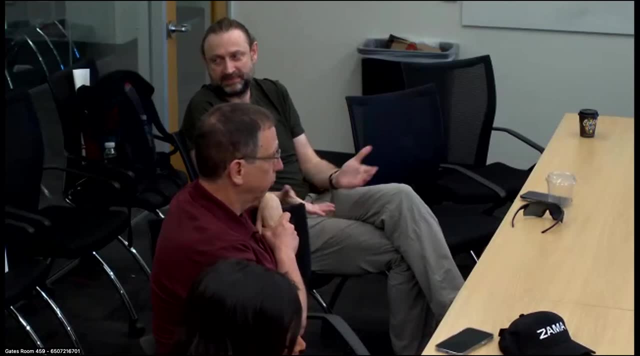 the instruction set. that was like it's proposable, but in the end we know that it's not going to be efficient enough. if we go that route, yeah, but you get your whole user interface for free, but exactly so. that's why it's it. it's in the works. I mean, this is exactly the kind of 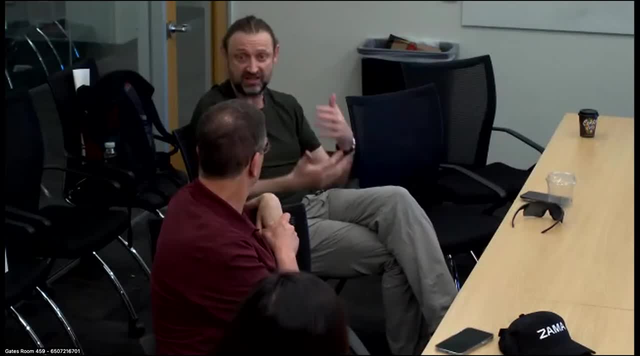 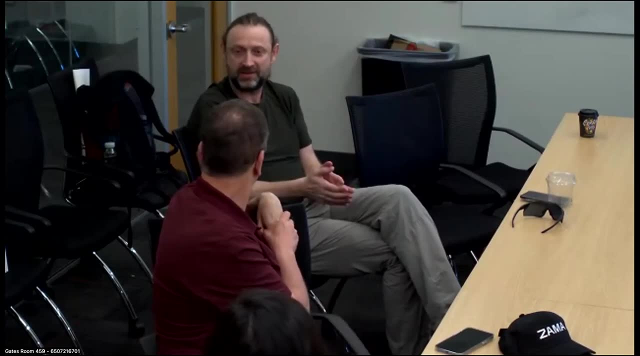 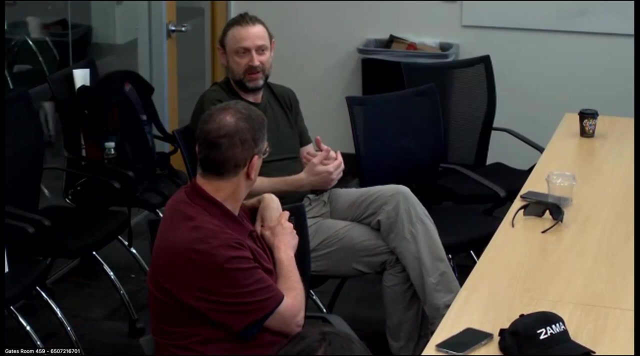 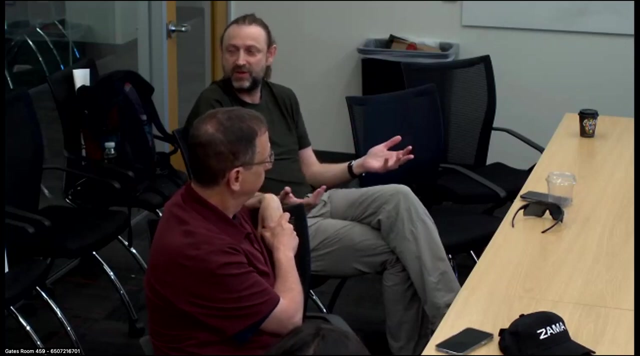 things that we're having like leadership, like discussing- okay, because not nobody's using this for real right now. nothing is really working, so things are in the pipeline. it's not there yet, so maybe in the end people will prefer the vm approach. it's good that you know there is. there is room for everybody right now, like we need more and more. 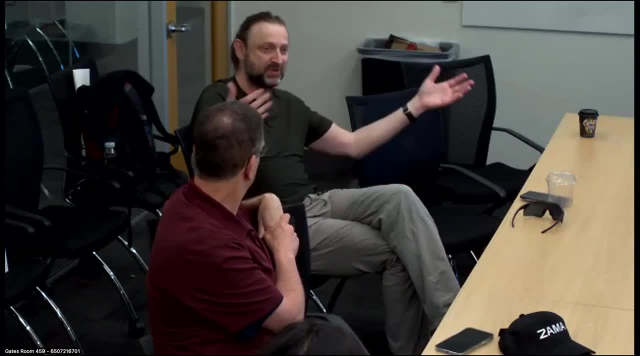 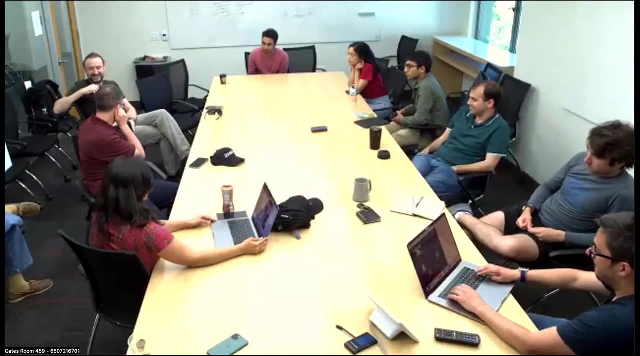 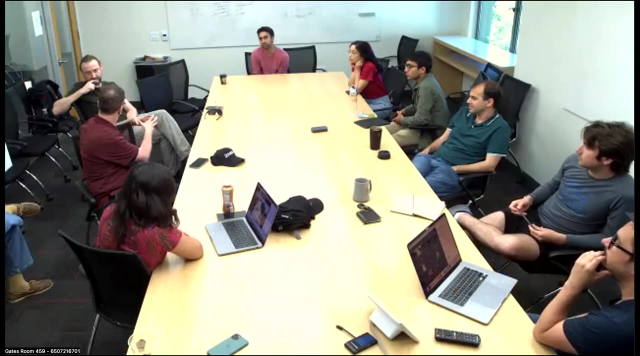 contributors, ideas with attempts, with demos, initiatives with the community. you said something interesting that, uh, you know, you, you're, you're that, you're this right that you think, you think that basically, the, the crypto construction for FHE converged to FHE and now it's kind of mostly engineering. 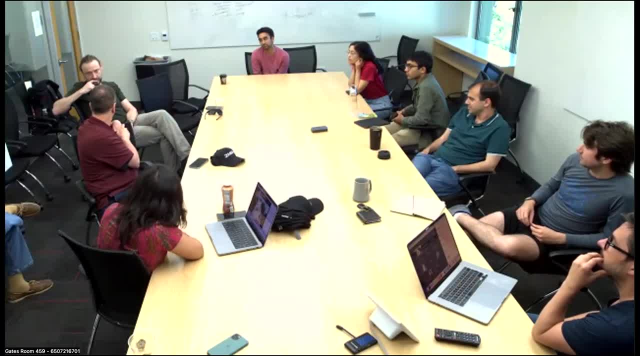 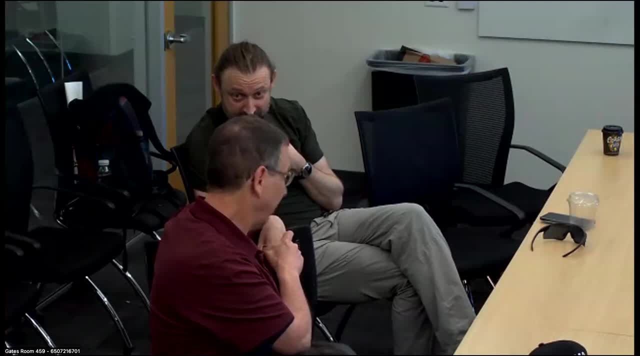 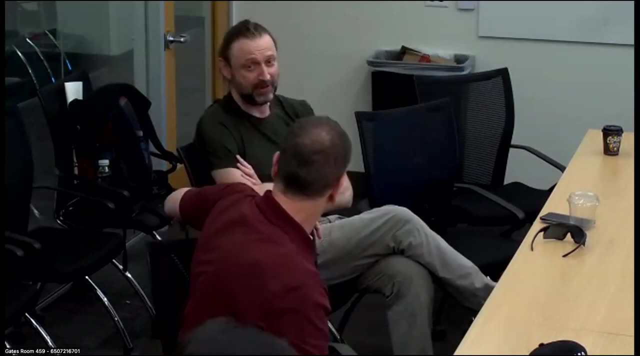 or do you think there are still room for breakthroughs in FHE constructions? there is room for breakthroughs, but uh, by the way, this is like my opinion. it's not everybody's opinion, but it depends who you ask, like people, even in the community, I think. 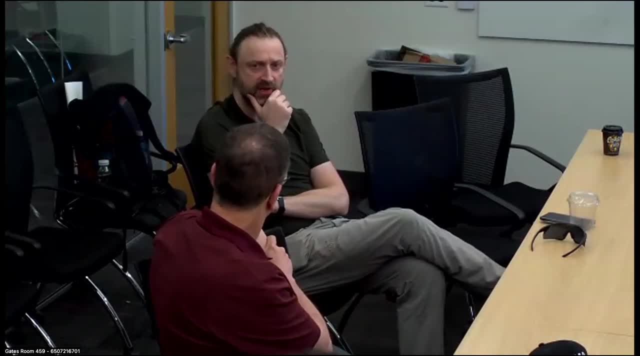 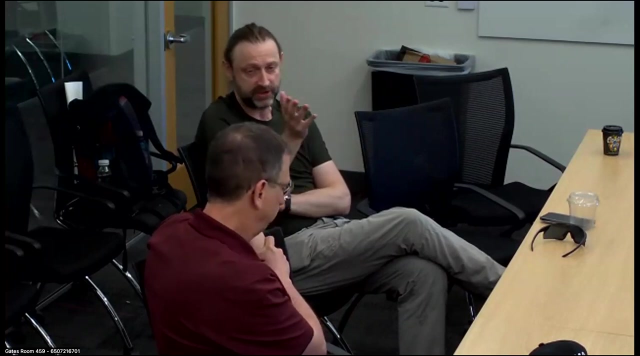 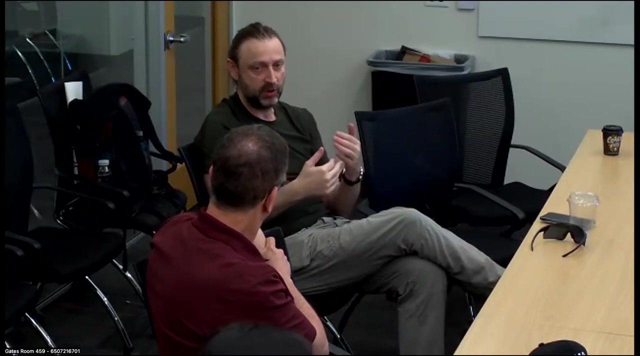 CKKS is like more popular than TFHT. TFHT was like always looked at as kind of the underdog. another scheme was there's a common misunderstanding which is: oh, TFHT is just like for bull intercores, which is not the case. you can process like small integers, but uh, yeah, but but to me, like because of this more flexible capacity, 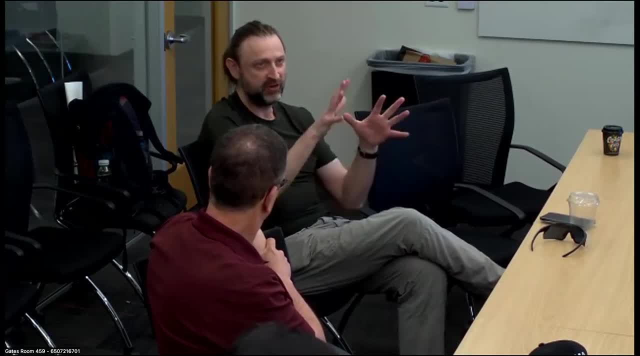 and because you can pretty much take them close like 18, you can take a multi-variate like function into a network of uh. basically look up tables, univariate functions and linear operations. uh can basically apply that transformation to anything. it's like there's this reconstruction appearance of machine learning where 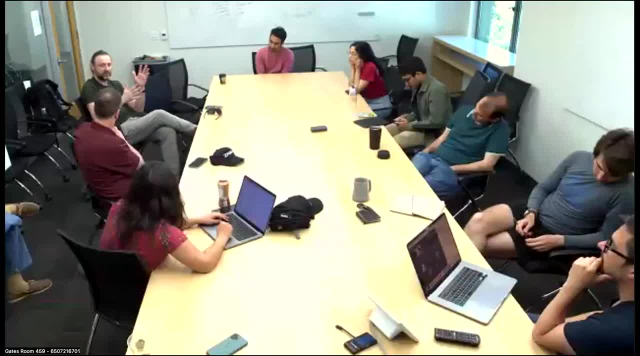 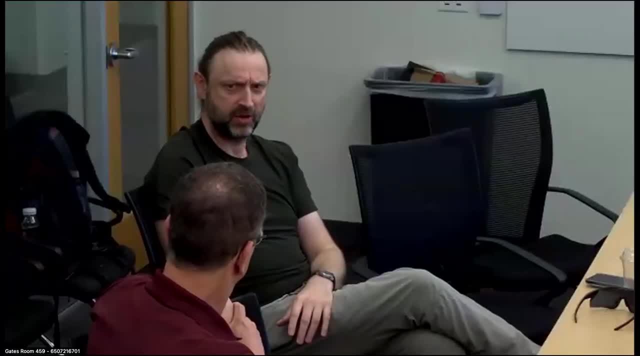 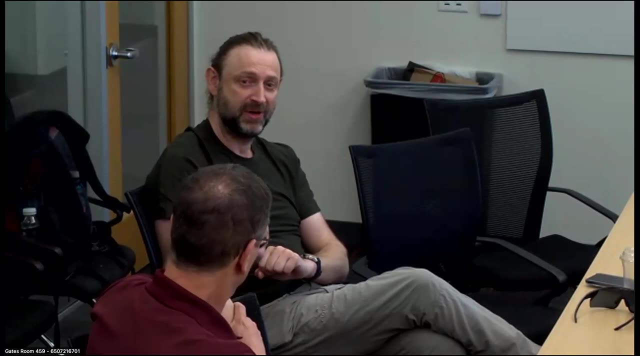 you prove that any multivariate function can decompose into a layer, a two-layer, I guess, one in a hidden layer. right homo graph axis position of your anna. we're still looking for a discrete version of that, by the way, where you where everything is like discretized into integers and you're allowed to use like. 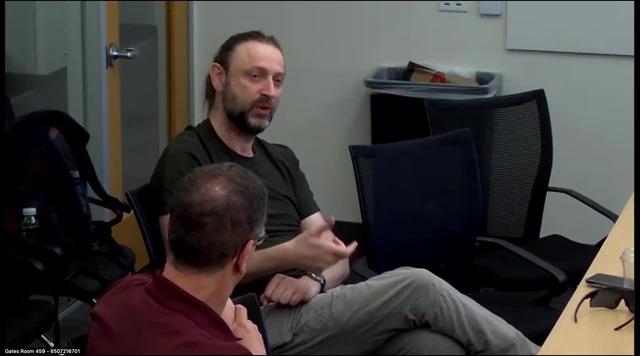 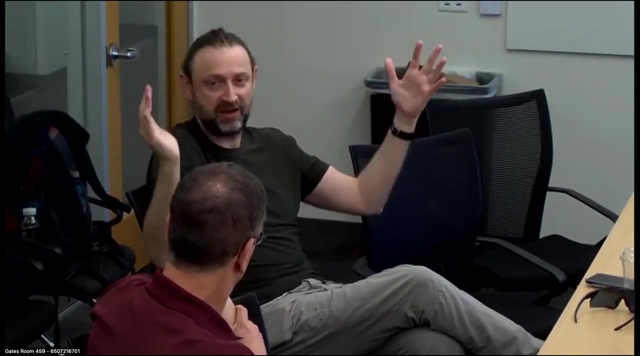 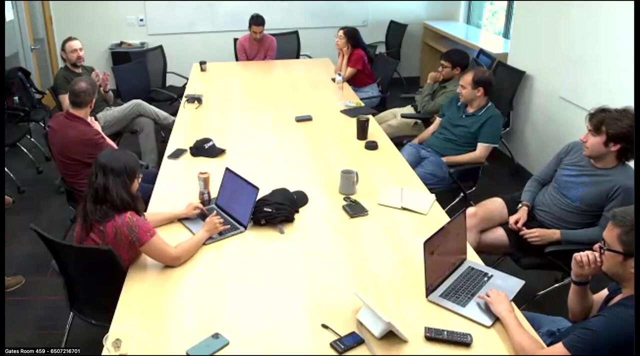 linear combinations, modulo something, and then look up tables and you're supposed to reconstruct with your network like any. like specified big multi-variate function, yes, but so in my vision, I think, I think TFHT is what we need. we don't need more. even if there are breakthroughs on the crypto side, there will be breakthroughs. 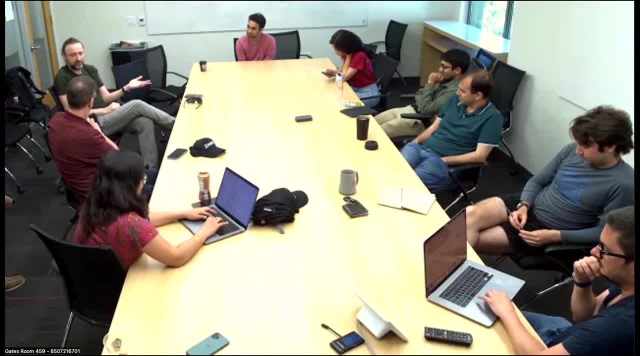 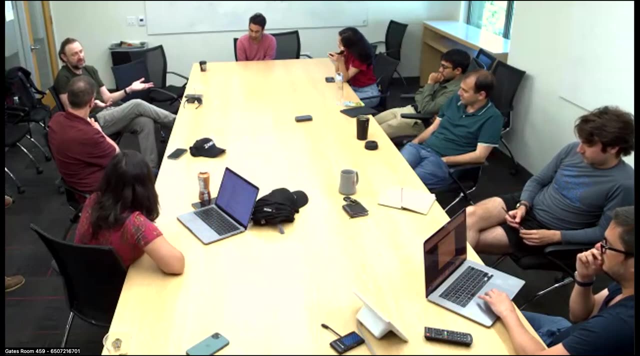 on the crypto side. but even without these breakthroughs, with good engineering and hardware acceleration, there's a huge appetite right now for data protection and people are realizing this now. I mean, it's always been the case, but now, with the ai, i've heard that utilities, i think, the user chat. 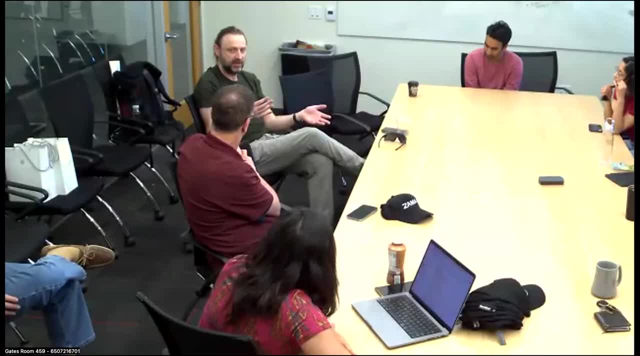 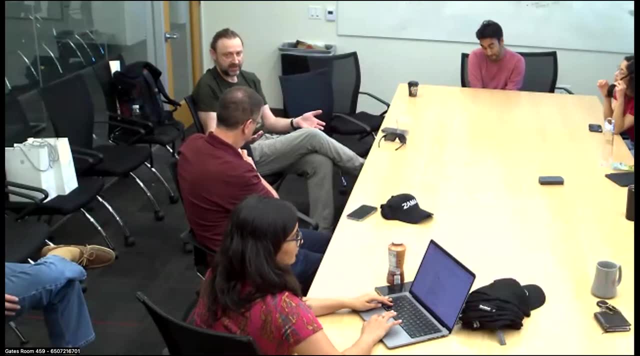 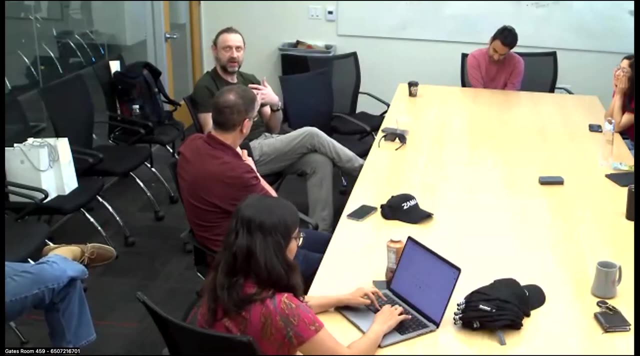 because of that, because there is no data isolation, uh, between the service provider and the user, and so, if the chief can provide that, it's not the only thing that can provide that, because that's not the only problem. they have to chat. that's not the only problem, of course, but i think, now that there's 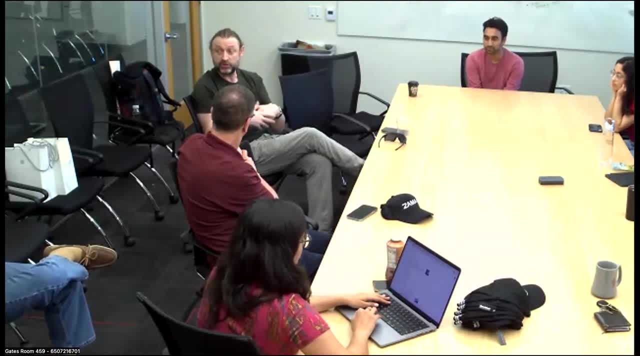 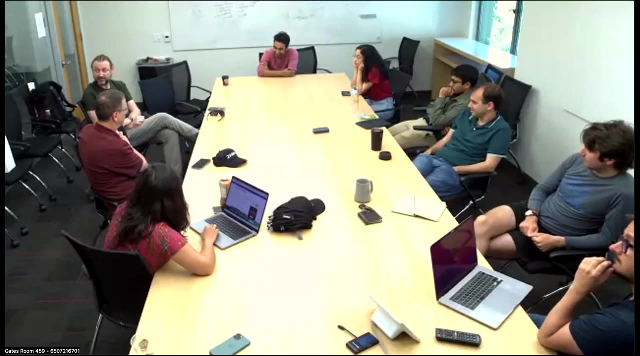 starting to be like market openings or opportunities that are opening for this. actually, you're introducing a problem because right now they filter the requests so they won't answer certain questions and if the questions are encrypted, they won't be able to do that. that's true. that's perfectly true. also, they will not be able to take advantage of these input. 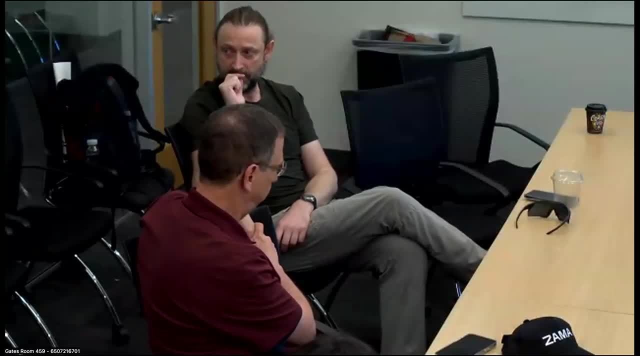 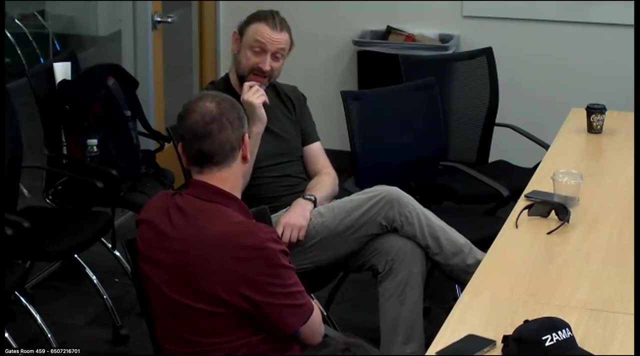 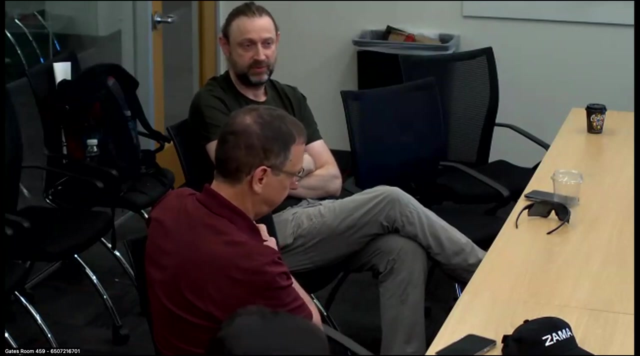 outputs coming from users to actually improve them. so you will have to use like a, a an instant, unless you can train them. yeah, sorry, unless you can train them. oh, we can train our group data. it's just uh, it's just very efficient right now. yeah, so we.